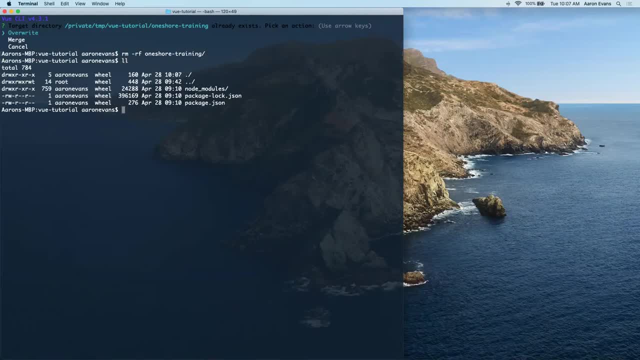 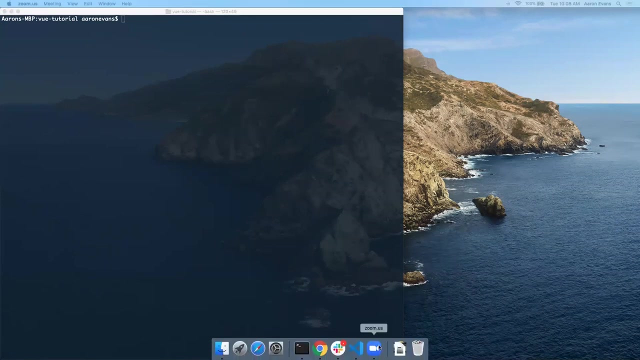 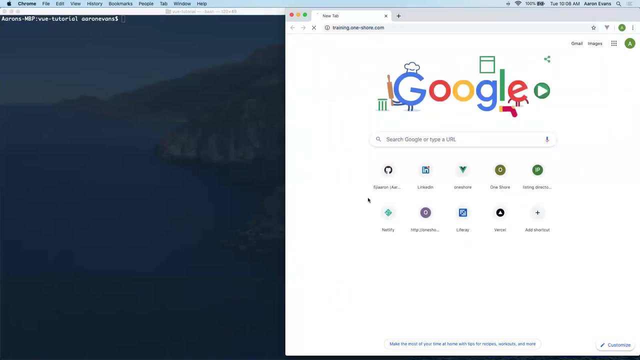 Let's kill this off, Okay, So We've just got to clean this out, All right. So now we've got an empty folder, So Let's start over, All right. So All right, welcome Today. I am going to start by building a website: trainingoneshorecom. 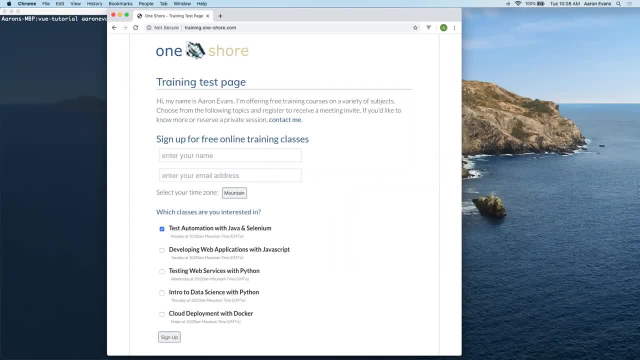 This is just a mock-up right now. The idea is that it has some static content and it lists the courses that are available: the test automation with Java and Selenium on Mondays, developing web applications with JavaScript on Tuesdays- all at the same time each day, and then you can change the time. 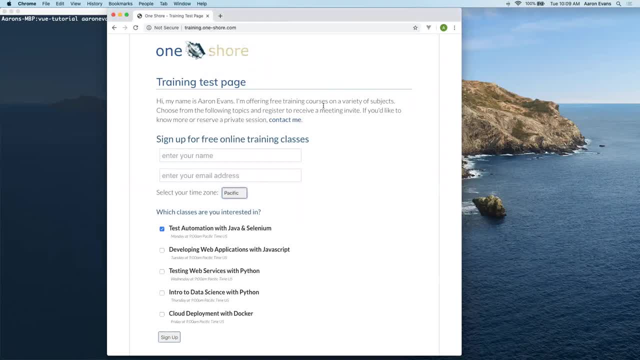 zone. This is just a mock-up written in static HTML and JavaScript. The sign-up form, as you can see, does not work yet. What we're going to do is we're going to re-implement this, Maybe improve on it a little bit, so that people can register for classes and create. 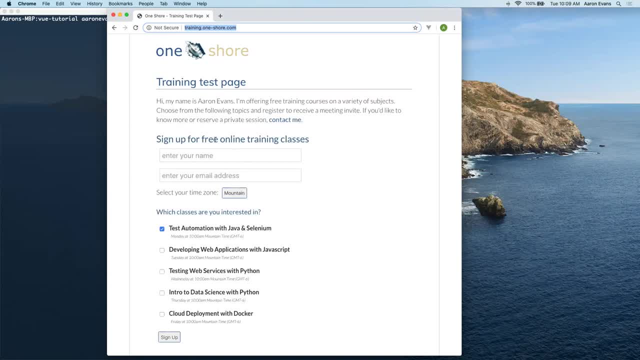 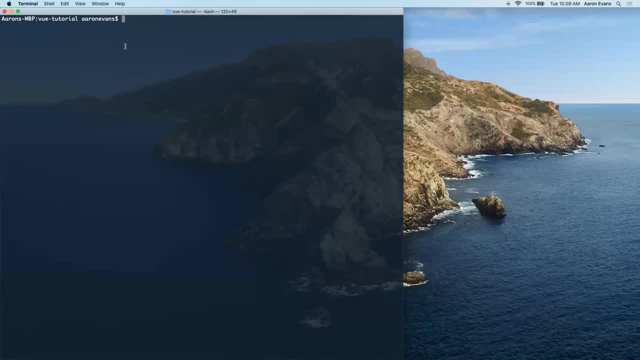 it as a Vuejs application and deploy it to NetBeans. First thing I'm going to do is install Vuecli. so you type npm: install dash g for global at Vuecli. We can look at the document. All right, There's documentation for this. 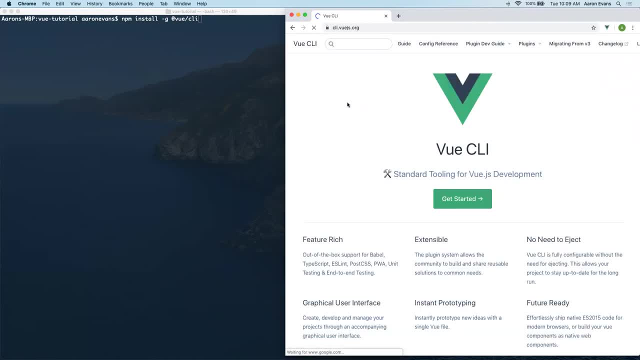 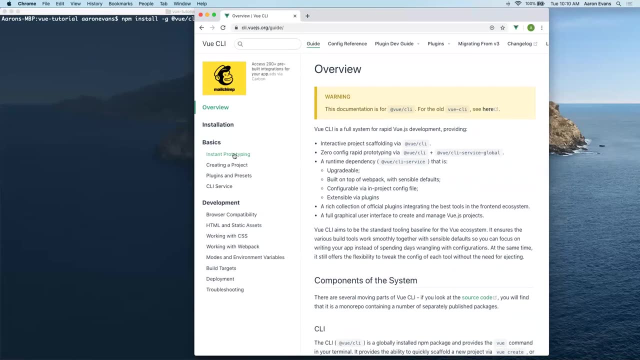 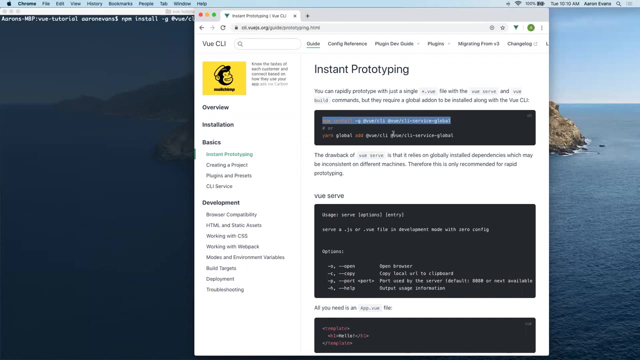 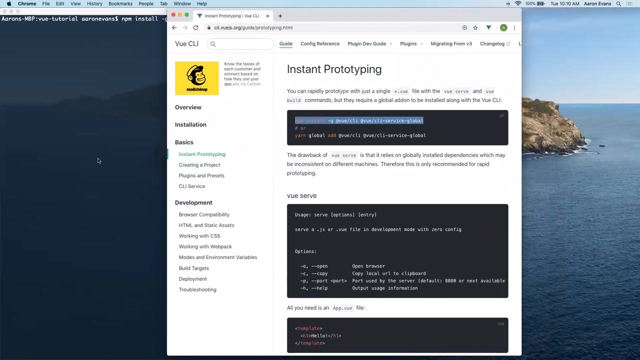 Vuecli: Getting started with the Vuecli. What you want to do is you want to install this and you can also install the CLI service global. I'm not sure what that CLI service global does. It may just use the serve, Okay. 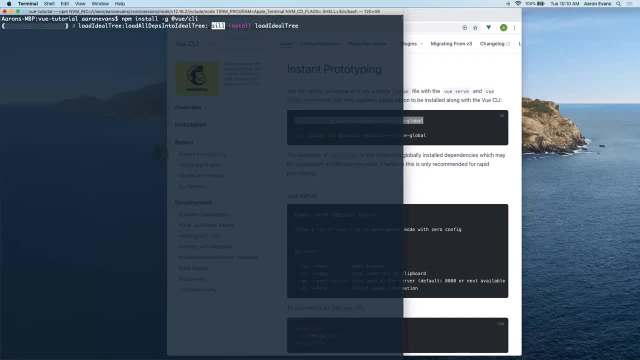 So let's just do that. I already have the Vuecli installed, so this will take just a minute to go through and reinstall or fail and say it's already completed. So I'm just going to open up another tab and open my code editor. 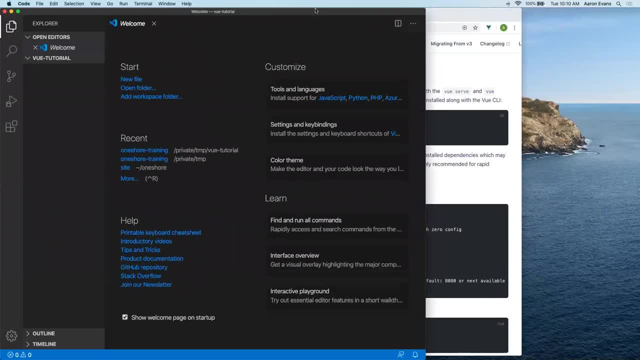 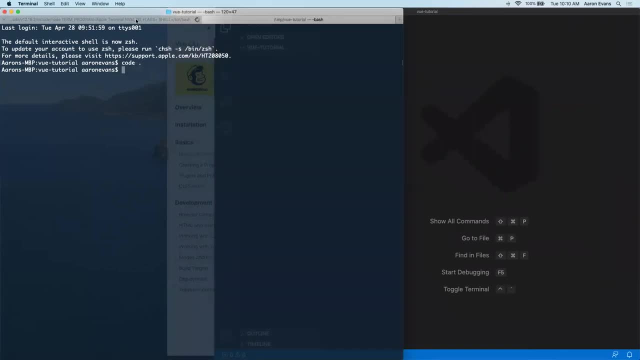 I'm using Visual Studio Code. Close the welcome here And see how this is doing. All right, It's wasting time, but eventually it will succeed. and then what we can do is, since I already have it installed, I can just type Vuecreate and hop on over here to the webpage. 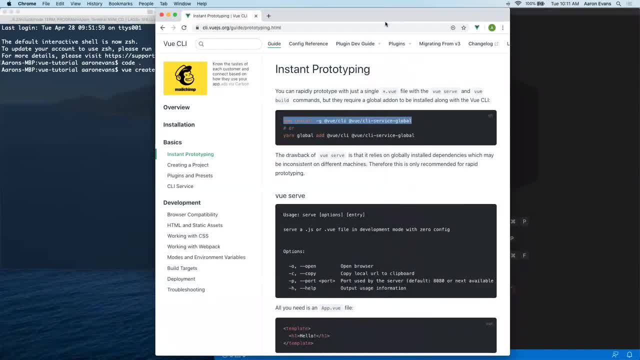 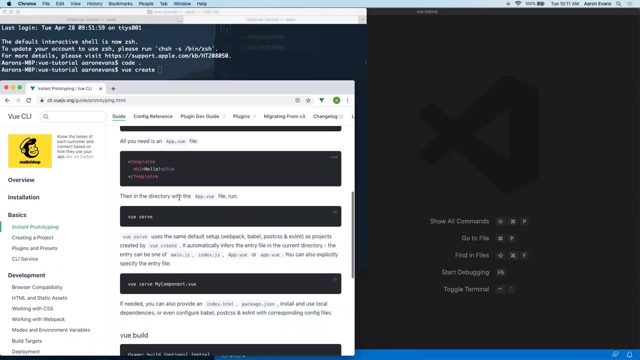 and show you what's going on. Let's make it so I can switch between tabs fairly easily. Nothing will be full screen, All right. So what I want to do is: Well, I don't want to Vueserve, I want to Vuecreate. 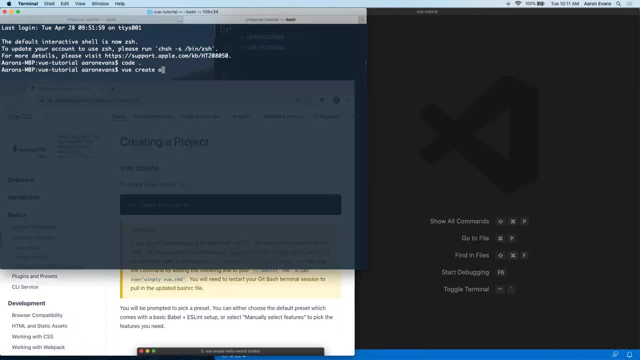 So creating a project. I go to Vuecreate and I'm just going to call it OneShortTraining and it will create the project. You see, the first thing it asks is: how do I want to set this up with the features? 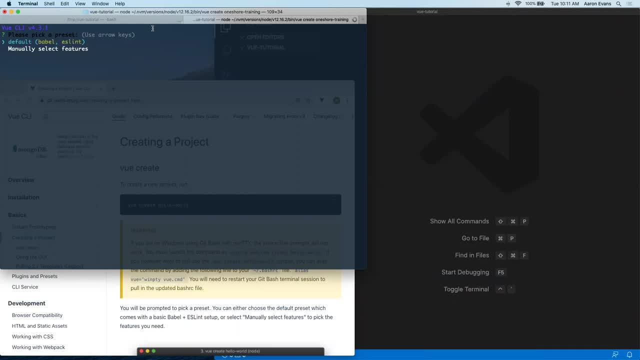 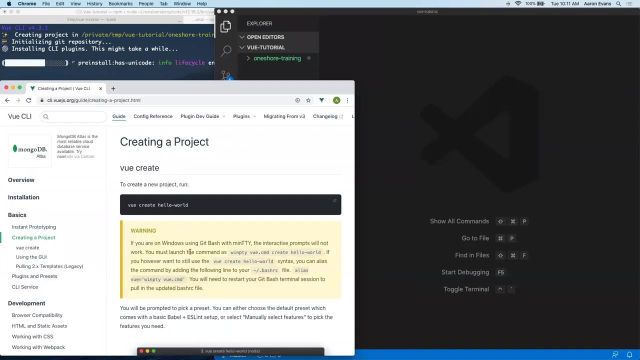 I'll just choose the default. It will use Babel for compiling and ESLint for checking static analysis of the code. It'll give you warnings If you don't follow the JavaScript guidelines that are specified by ESLint, which are configurable. So let's go ahead and look at the documentation while that's loading. 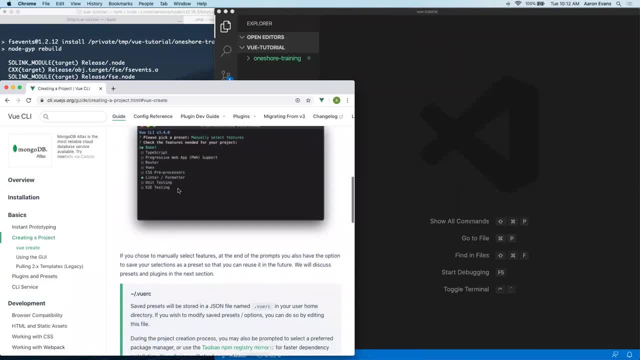 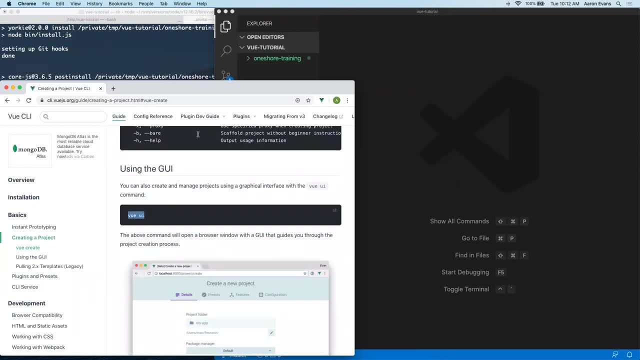 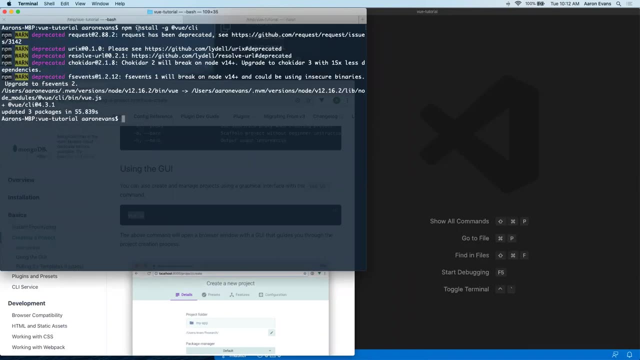 It says: pick this and you can optionally go through and change that. You can edit your Vue RC. You can also use the Vue UI to create a project. Let's look at that. Well, it's already running, So let's take a minute to look at the Vue CLI or the Vue UI. 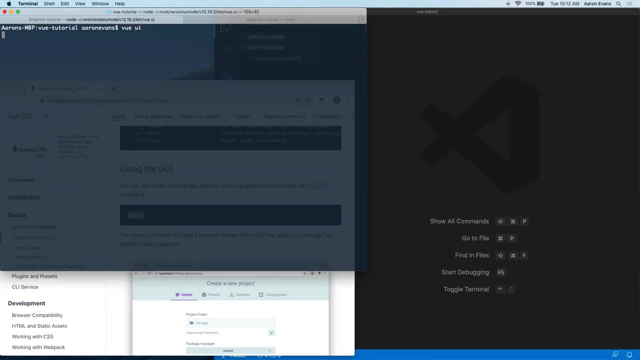 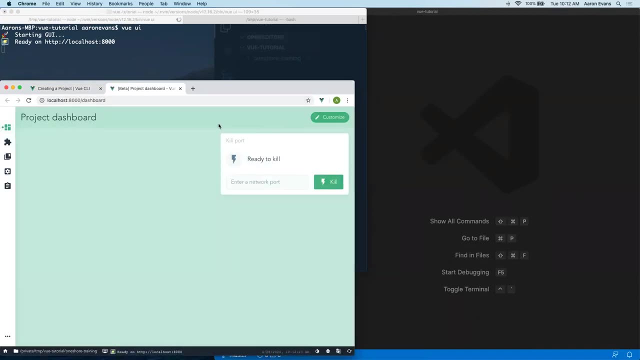 I mean, if I just type Vue UI, it's going to open up a new browser on port 8000 by default and it allows you to do a lot of things. You can kill a port if you want to Say you have multiple apps running. 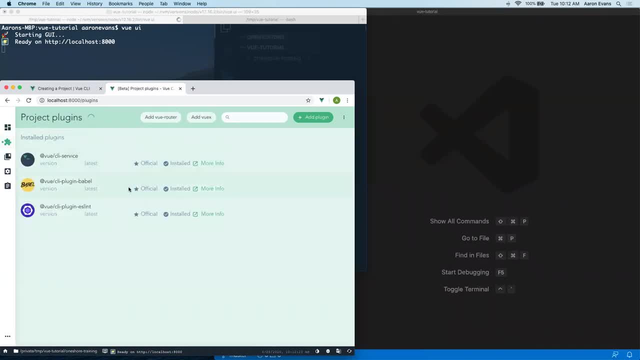 You can install plug-ins. We have the CLI service of Babel and the ESLint plug-ins- See the dependencies of CoreJS and Vue, ESLint and the Vue template compiler. Different configuration: You can configure your project to specify what do you want for your public folder. 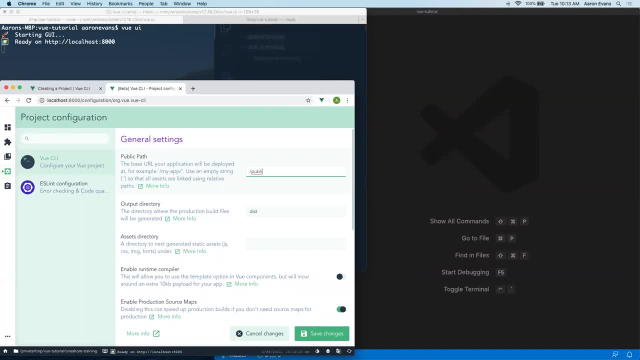 You might want it to be public or whatever. We're going to keep the defaults for now. Just hit refresh, since we didn't save it. Cancel changes. okay, And you can configure your ESLint, specify your ESLint RC or you can go from essential. 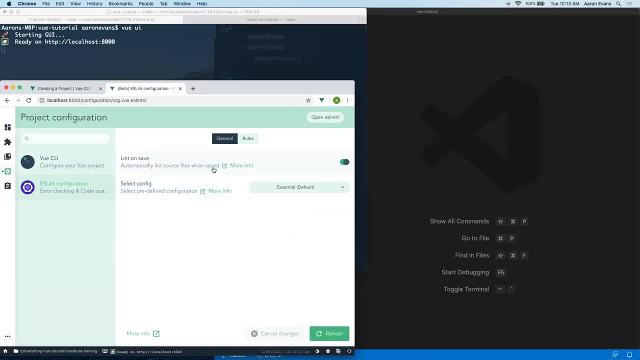 to strongly recommended, or recommended Just different levels of warnings that the linter will show. Let's go back to our dashboard. We can kill, We can customize, We can also create a project. I think I need to expand this out too. 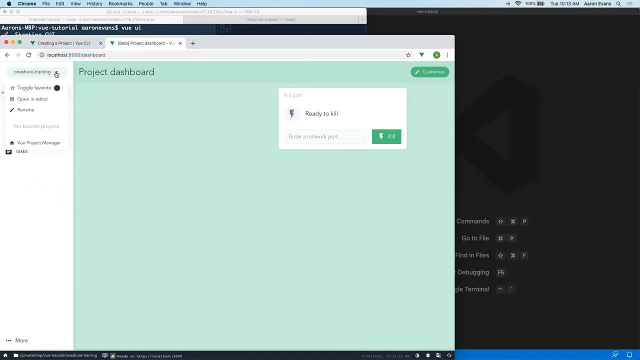 Let's see that. Oh, it already has it. here has my project, So I can rename this project if I wanted to. Here we go. This is the screen. I wanted to see The project manager. I can create a new project specifying folder. 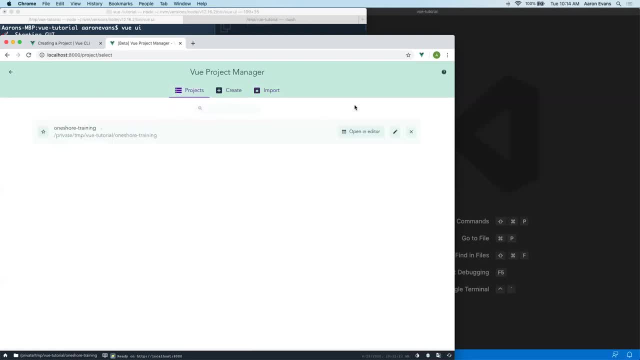 I can import a project from a different folder and so forth, So I could actually create a new project. I can create a new project And I can do it in temp-hello-view, something like that. Does it need to be private? 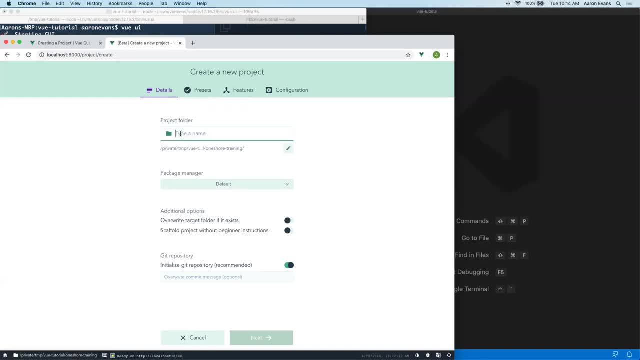 Temp-hello-view. Oh, it needs to be under this current directory where I'm at, under the view tutorial where I started this. Okay, All right. All right, So I'm going to update this New project manager so I can create a project. 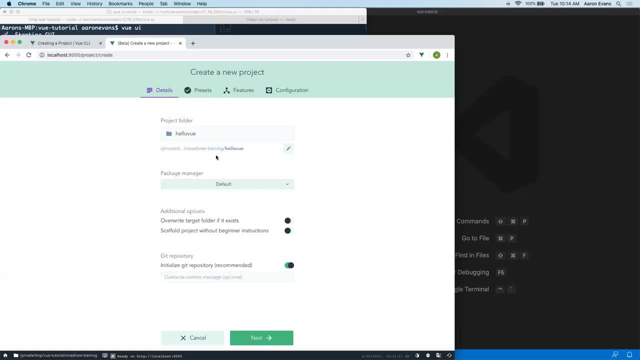 Call it hello-view. And now it'll go under one short training. I don't really want it under there. but Oh, I also want to show you can initialize a Git repository or not. You want to select your default presets or not? 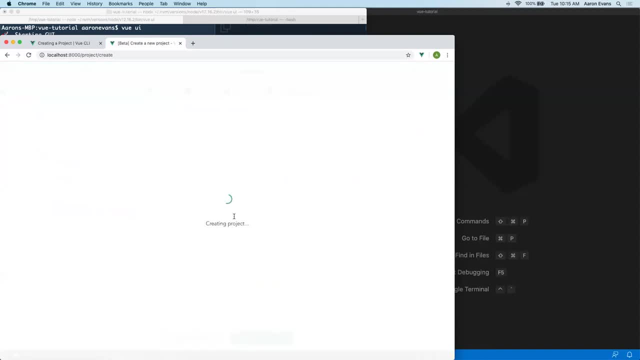 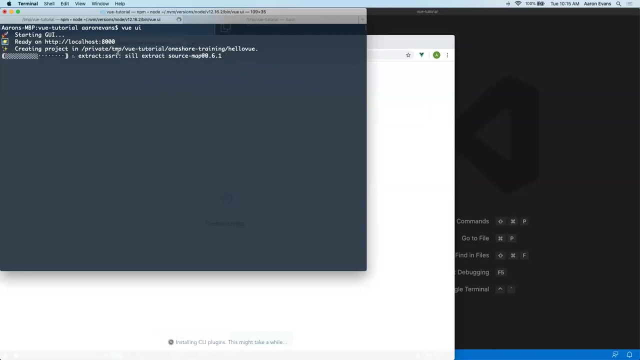 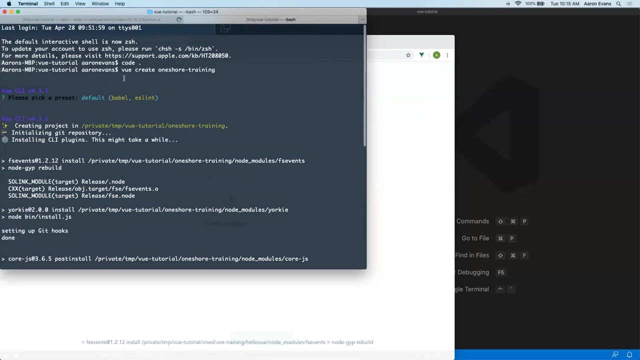 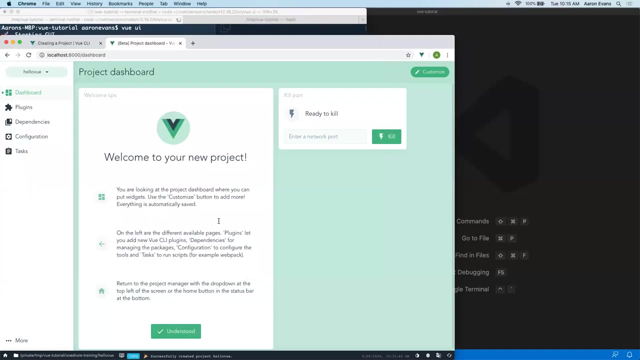 All right, Great, manually, and it's going through and it's, you see, through the view UI. it's essentially doing everything I just did in the other folder where I typed view, create project name and you can see. it shows the project dashboard. welcome to your new project. so 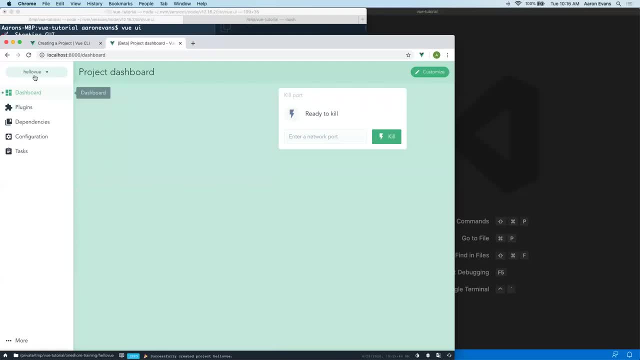 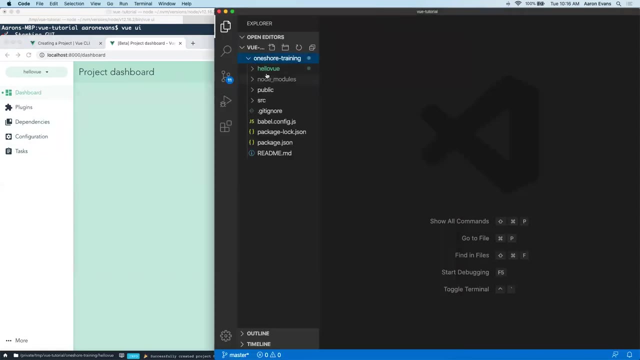 let's go ahead and look at that. so we have one short training and we have hello view. so let's go ahead and look at hello view, which is under here. it's kind of ugly that it's nested like that. but we start with public. we have 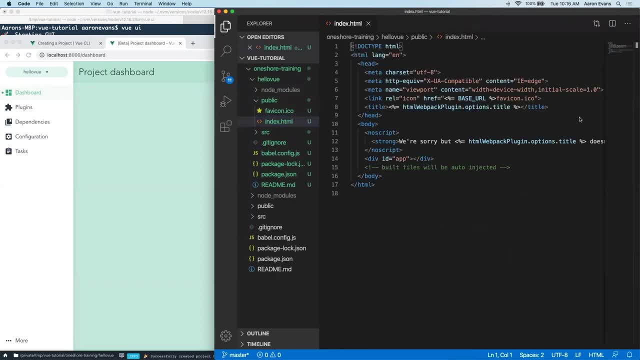 our indexhtml and it's just a template. right, it has HTML, so it has some meta as a title and it gets the title from these webpack options. you can look at these template variables- base URL and Where To Begin and title- but what we really want to see is, uh, that our app element exists, so build files will. 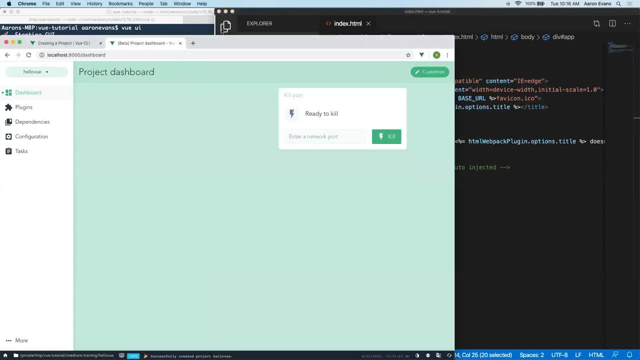 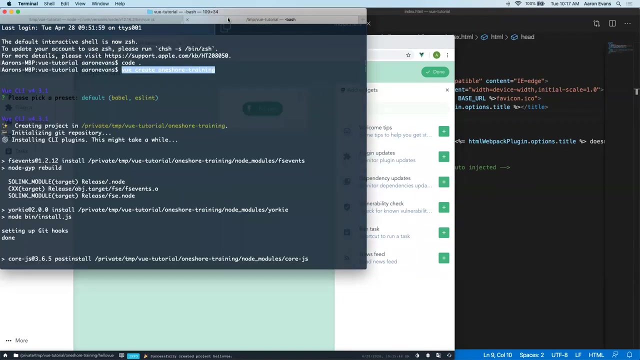 be auto ejected. so right now we are not running this yet, but in order to run this um, can i run view serve here? i don't know, i never used the ui before. what are these? um? i don't know um, but in order to run this, if we want to run our app, we can. uh, let's kill this view ui. 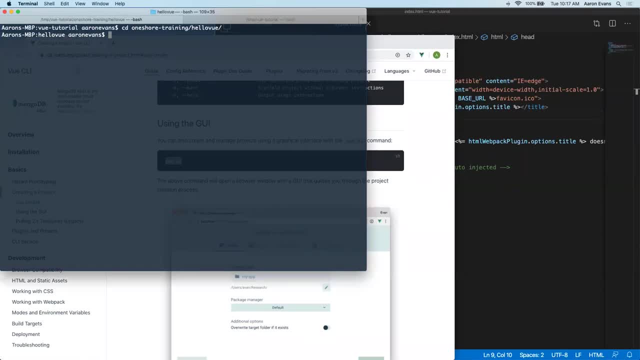 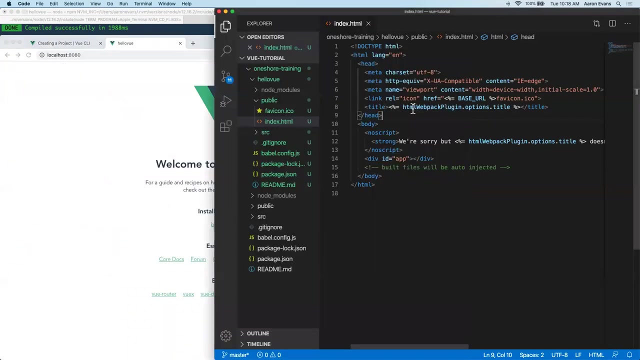 um, so we're in this hello view folder and i can just type npm, run serve and it's going to start up a development web server and you can see it. uh says start on port 8080. we'll go on over here and oh this, it has this. hello welcome to your view app, right? um, let's go ahead and cancel out of here. 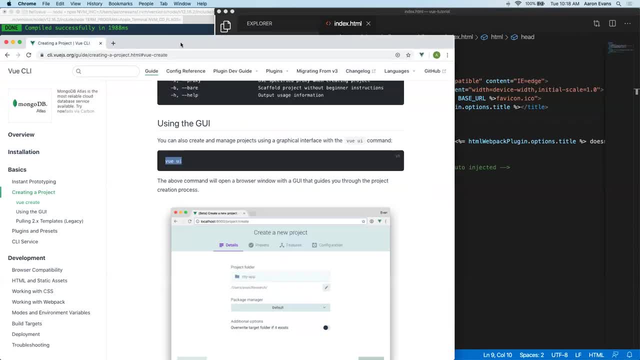 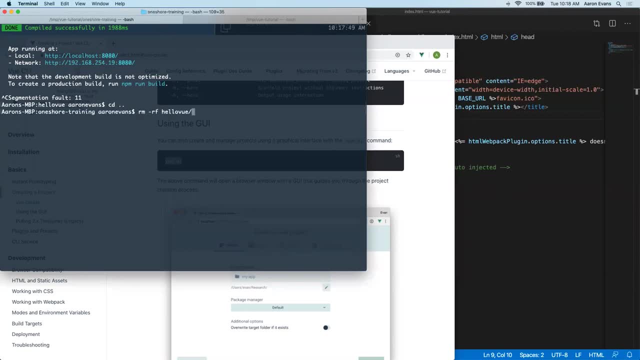 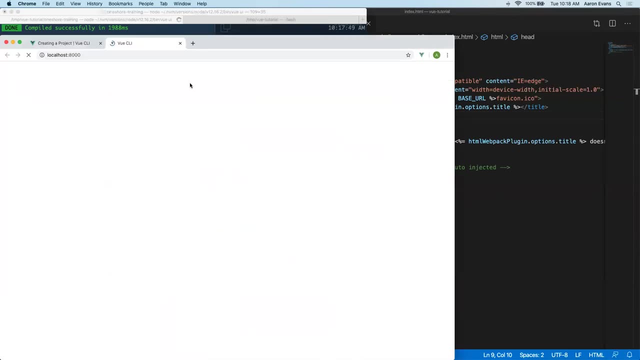 i'm going to go ahead and delete the hello view and we'll work on the one short training. i just wanted to illustrate that you could create apps from the view ui. let's go ahead and destroy the project via the ui as well. oh, it doesn't have option to kill it. um. 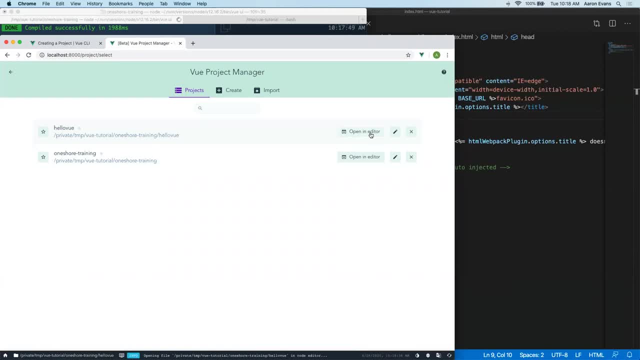 project manager: opening editor. opening in code editor. what editor is it going in? it's not opening it in code. i don't think. it's opening it in vim. let's kill it off. i don't even care about that. ui, maybe it's cool, um, but i don't know how to use it. 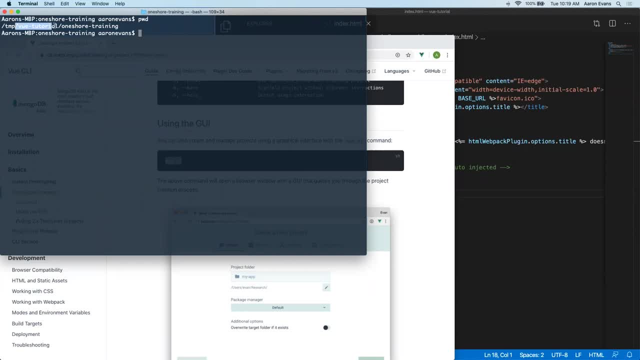 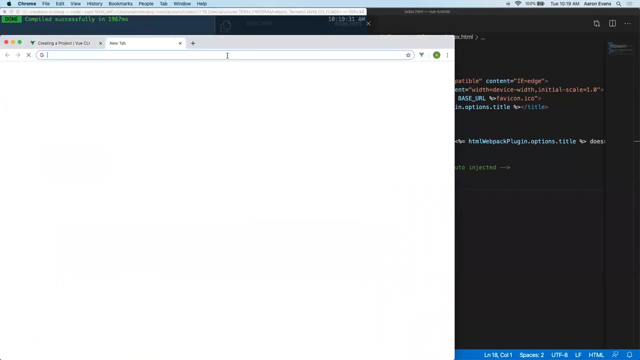 so we are in the under the view tutorial. i have this one short training directory. now this is there's nothing here. if i uh, if i type view serve here, oh yeah, npm run serve, let's go ahead and do that and we'll go here. we'll close to here. so now we are um. 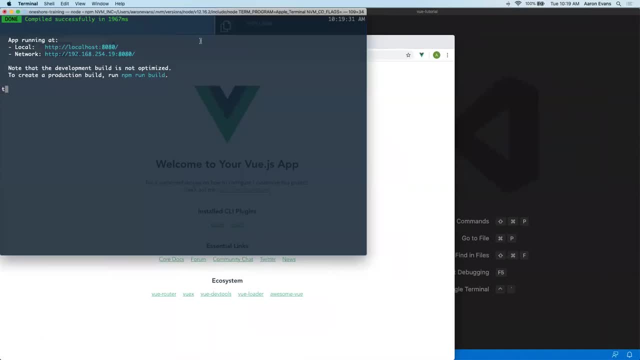 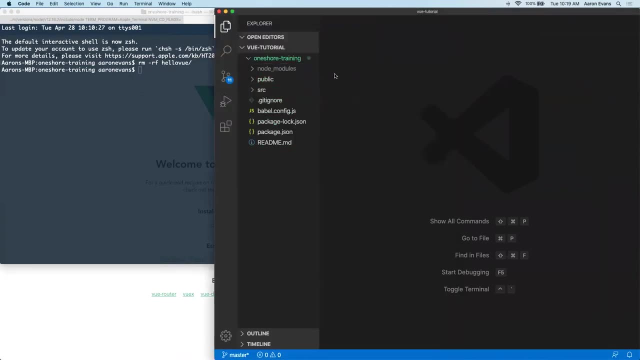 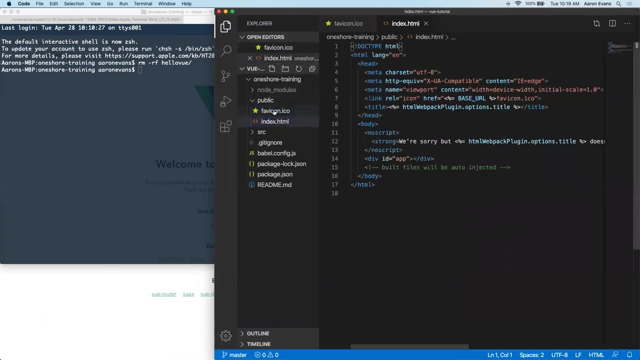 i thought i removed that hello view folder. there we go, all right. so what have we got? we've got public. we've got an icon, which is the view icon. we'll try and replace that. we've got wii, our index, which has our app, and some stuff for the title and stuff, And then we have the source. 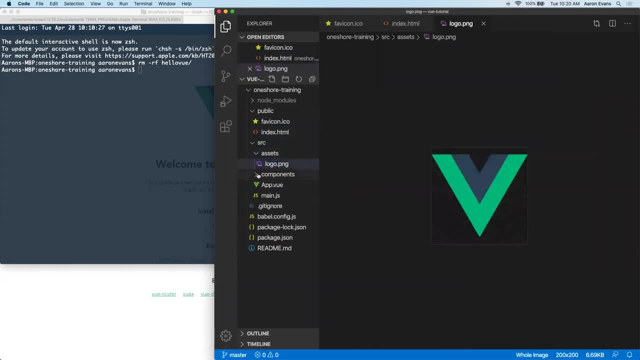 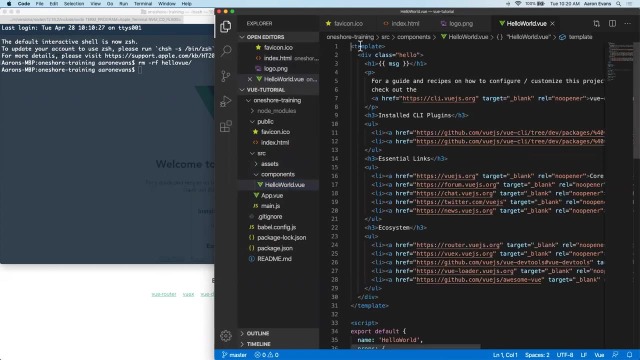 folder, The source folder, has our assets, It has the Vue logo. It also has components. So the hello world Vue component And you can see that this template here, this is a Vue component as a standalone file. We haven't looked at this before. Last week we created Vue components inside our 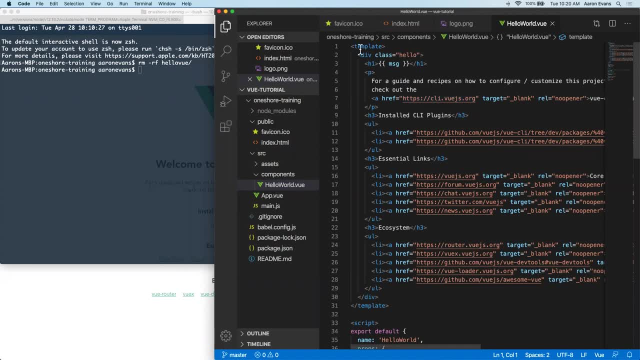 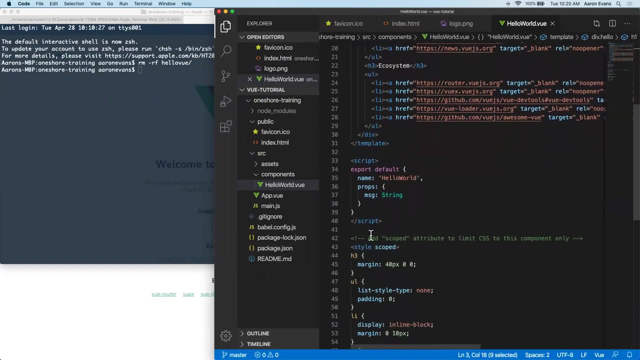 HTML or imported them with script tags. So a Vue component in a single file component looks like this: It has a template Within, the template is HTML and you know our template tags and so forth, For instance the message, And then it has a script, So you can see it gives a name to our. 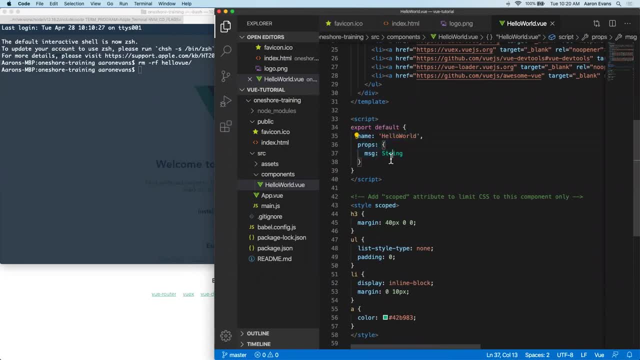 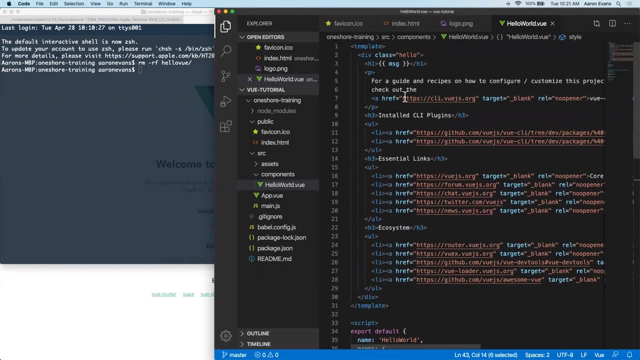 component. It's called hello world and it has properties. This property is message and it tells us it's a string, a type string. So we also have scoped style attribute. this is scoped is not part of HTML, but view knows how to add scope style so that the style I add to this component will not. 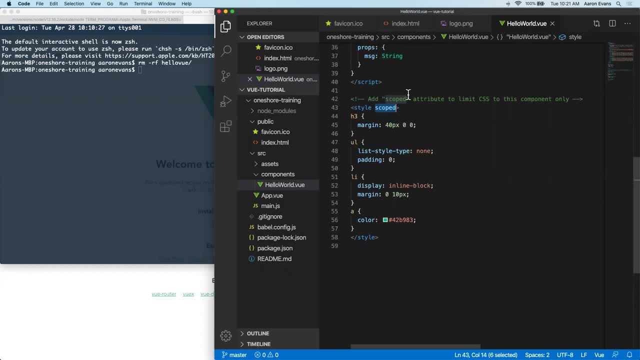 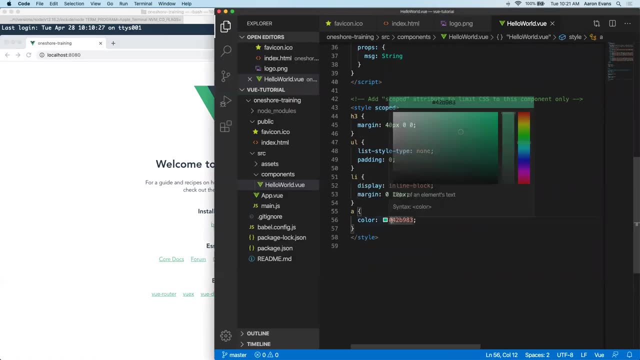 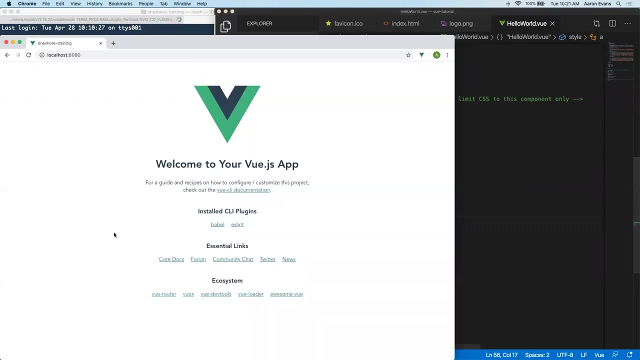 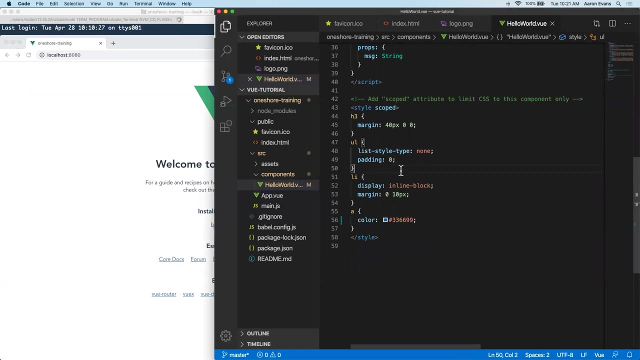 bleed out into any other HTML or other components in this document. so, for instance, we can change our link colors. right, we can change these to the three, six, nine oops that I like for my own branding. so now my links are kind of a dark blue. we can also do things like we can change the font. 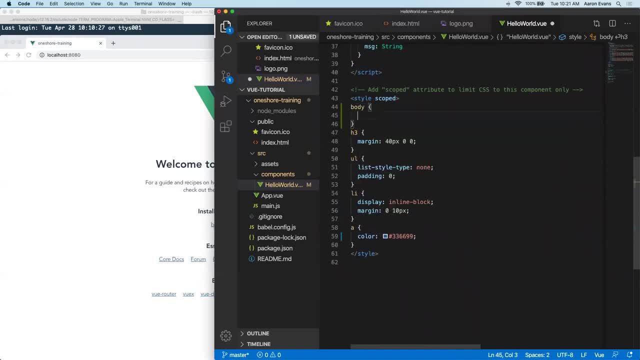 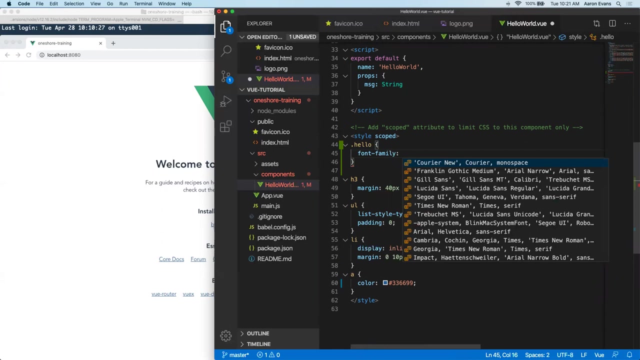 and we can change the font for the whole body. well, let's not change it for the body, let's change it for our hello class, and then we can do things like we can. a font family. you cannot change it to courier, just so. it's something that's easy to notice when it changes and it 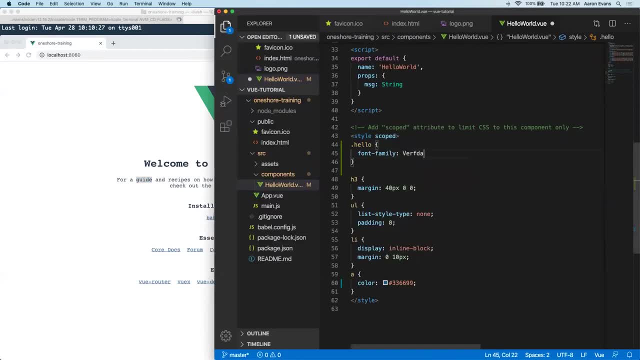 looks like a typewriter font, or we can change it to Verdana, which is what my one chore logo uses, and then we can use sans-serif um as a fallback, so we can fall back if. if your system doesn't have for Donna, then it will fall back to sans-serif. we can even do aerial. that's kind of a midway. 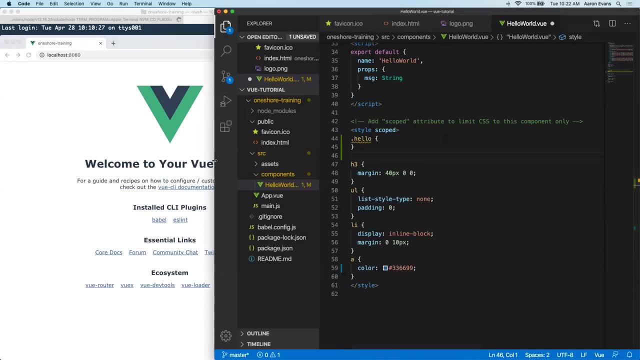 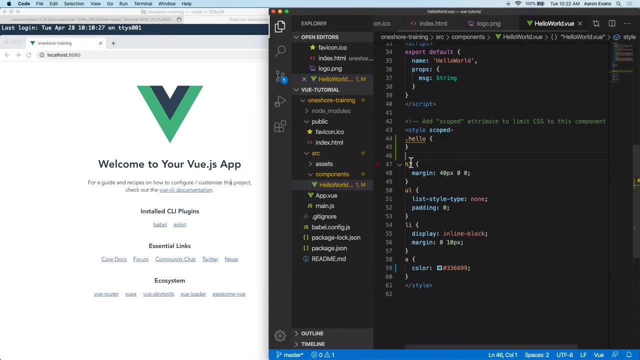 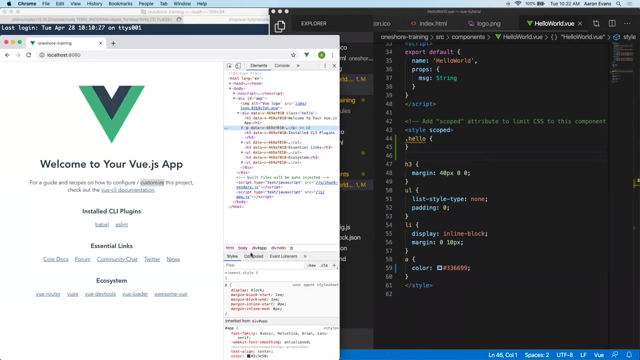 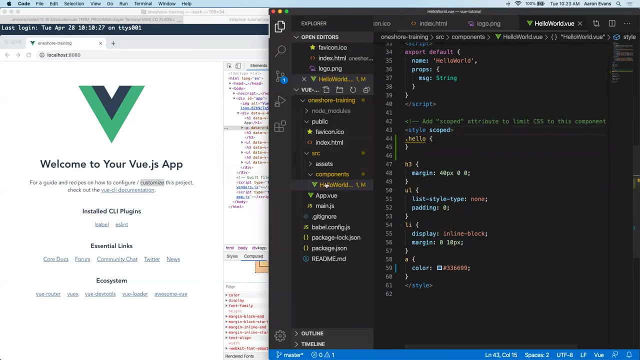 let's go ahead and move this over. we don't need to see that as why we don't need to see. that is why either, and that goes back to whatever these defaults are. What is this default font, Computed font, family, Avenir, Helvetica, etc. That comes in from, probably here, yep. 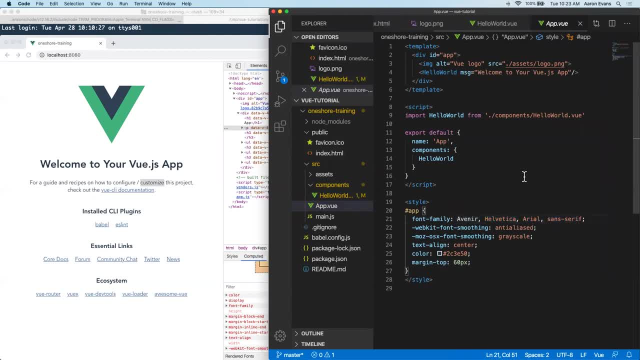 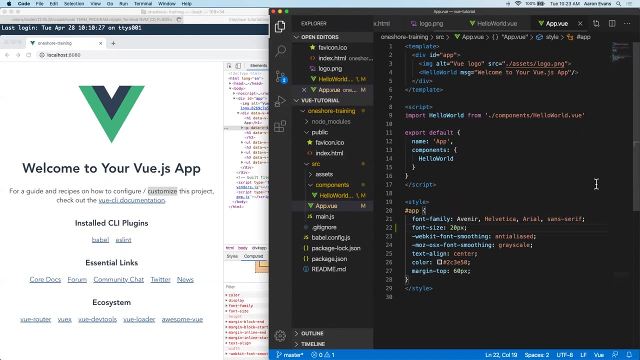 from our app default. So that's pretty good. We can also in the app. we can do things like: we can change the font size, change it to 20 pixels, make it bigger, So you can change your style in your app or in your nested component. Let's. 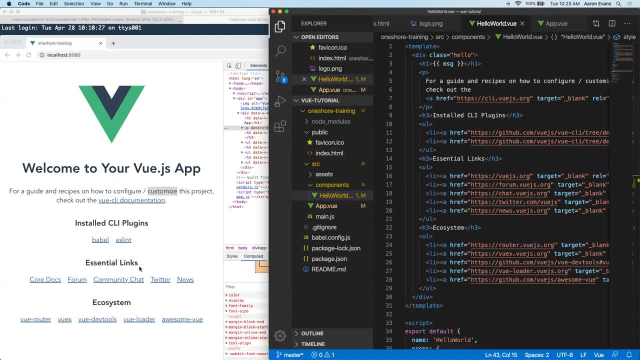 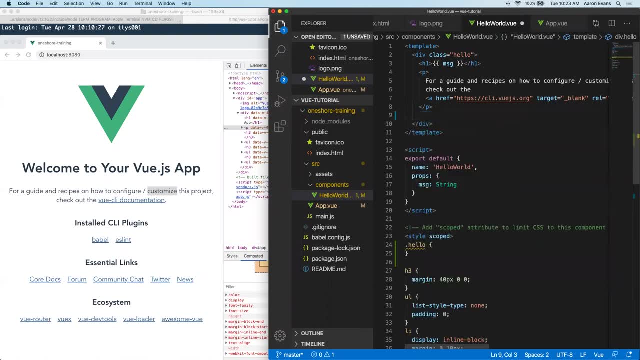 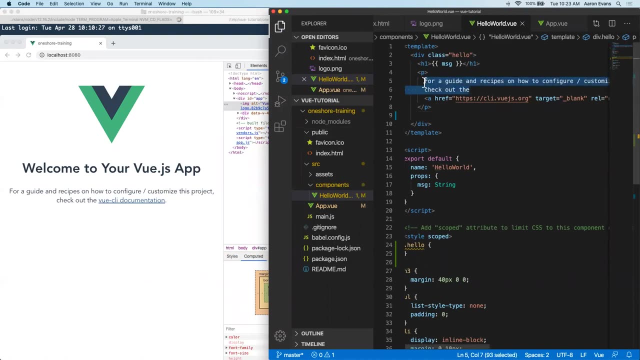 take a look at this hello view. We've got our installed CLI, public plugins, essential links and ecosystem. Let's just go ahead and delete all these things, And there we go. Let's go ahead and just change the text. Well, let's not do that. 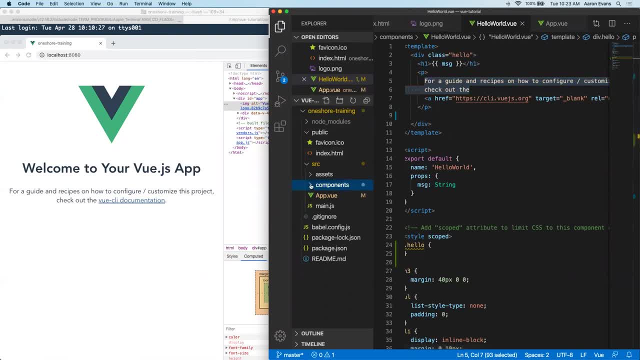 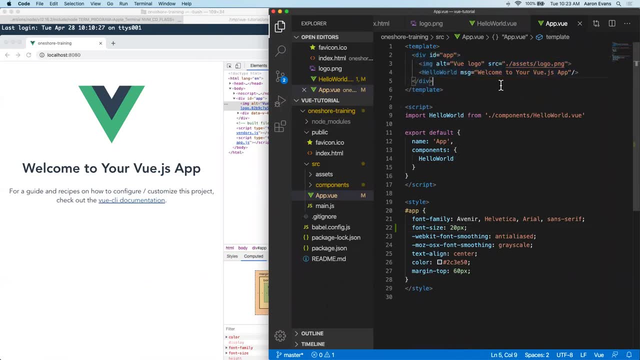 let's create another component. So we have our list of components here and we have our app view For our app. what does our app do? Well, it starts off with a template and it has welcome to your view app. Now, this welcome to your view app is part. 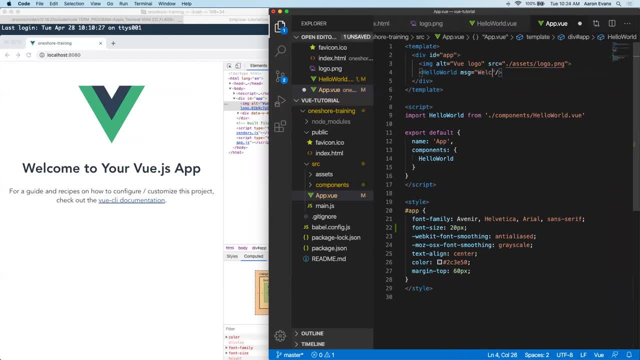 of the message so I can change this to say: welcome to your view app. one sure training. and it changes this. this is actually calling the hello world component, so you can see my wrapper component. here is this ID app and I'm gonna go ahead and change my logo too, and this is going to be. let me see, I 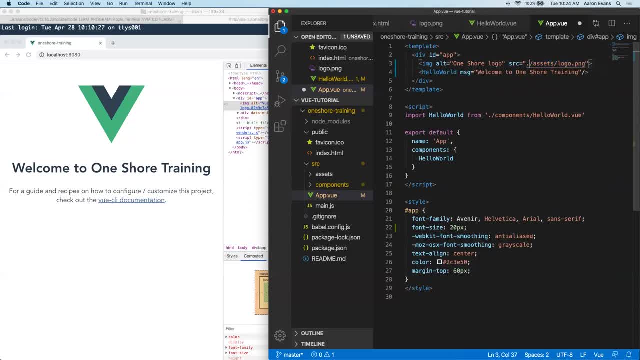 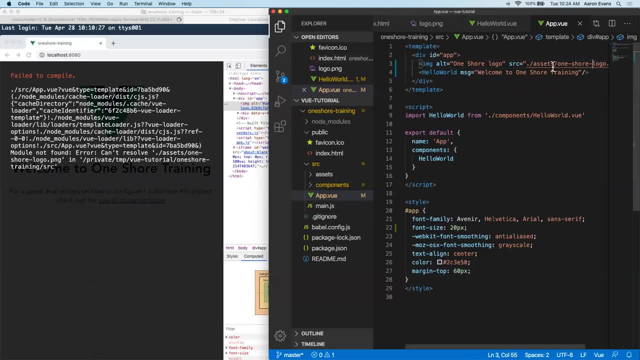 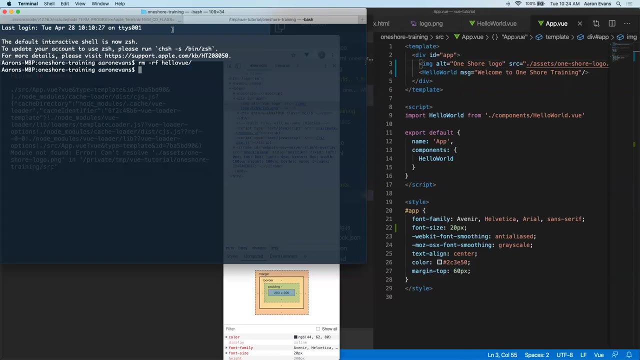 need to move that to. I need to move once you're low in here. okay, so it fails to compile. why? because it can't find this in assets. so let's go ahead and we'll pop on over here and we've got our. oops. I shouldn't have done that, that's gonna. 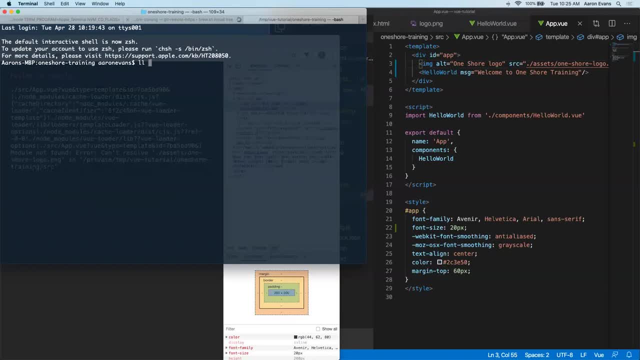 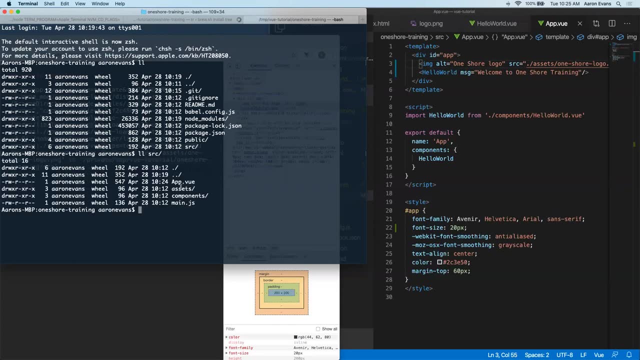 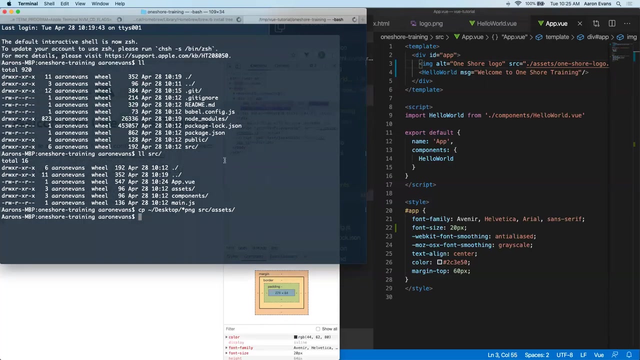 take a while. I just wanted to show that we have in the source folder, we have the assets folder. so what I want to do is I want to copy and I have my logo to source assets, yes, all right. and then you see it. it automatically reloaded. it had the. 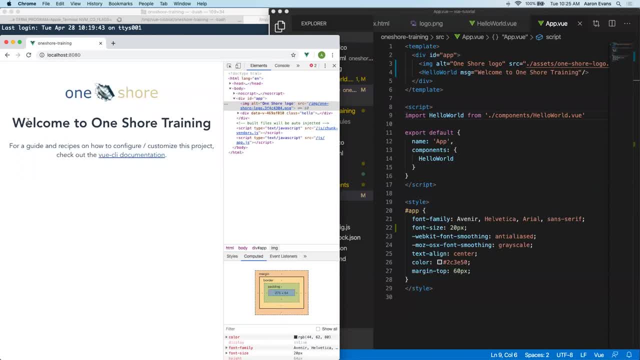 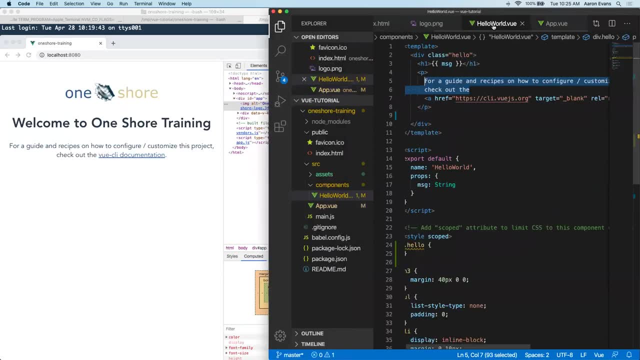 compile error that it had to do that, and then I just wanted to show that we have that. it said it couldn't find the assets. now it has the assets, so we're doing pretty good. welcome to one short training. let's change this text here. this is in the hello world view component and I'm just going to copy my 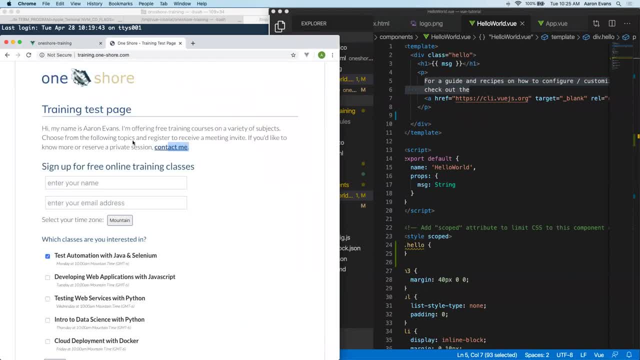 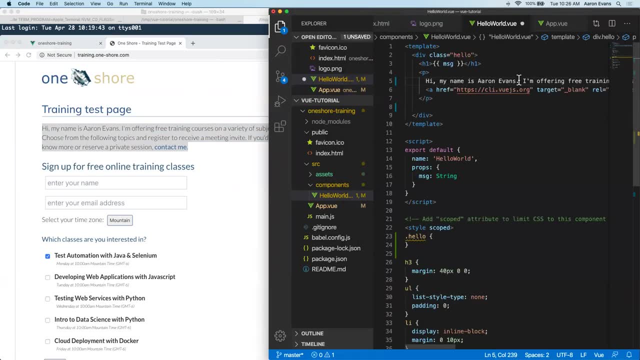 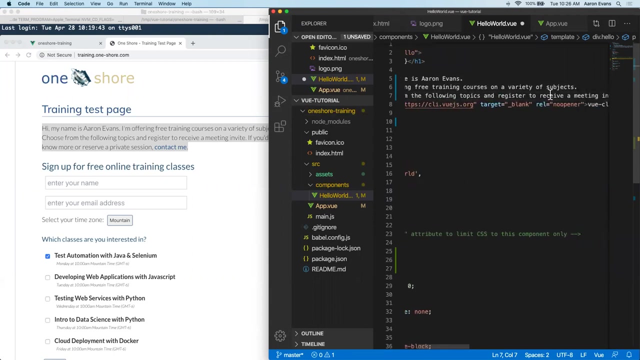 text, so I don't come up with anything original here. not that this is great text, but you, you know, let's get that bigger so we can read it. so I can read it with my old eyes. choose from the following topics and register to receive a meeting invite if. 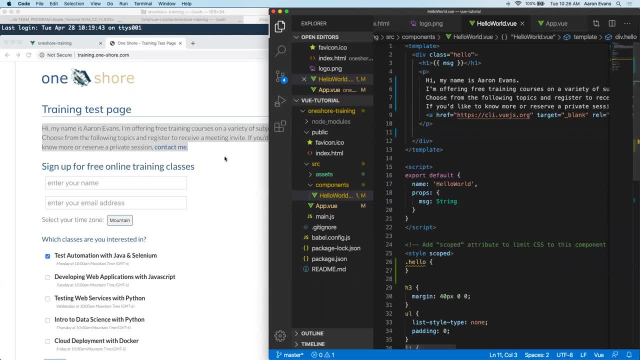 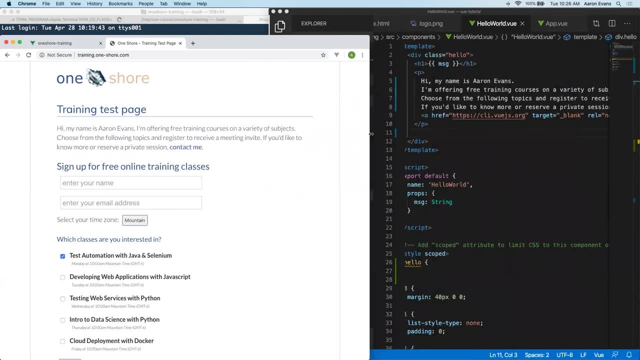 you'd like to know more or reserve a private session, contact me. okay, and that's not going to change anything here now. this is kind of a fix. oh well, we're not even looking at the right one here now look. uh well, we don't want it centered, so we're going to go ahead and 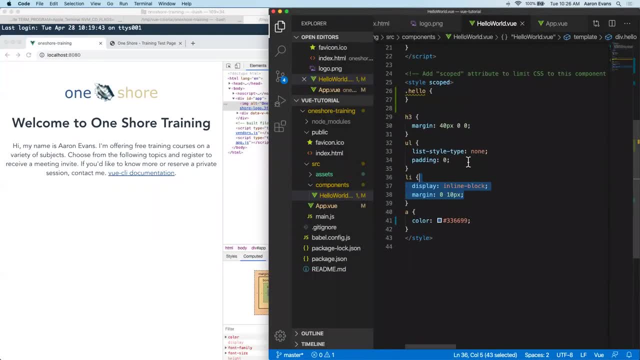 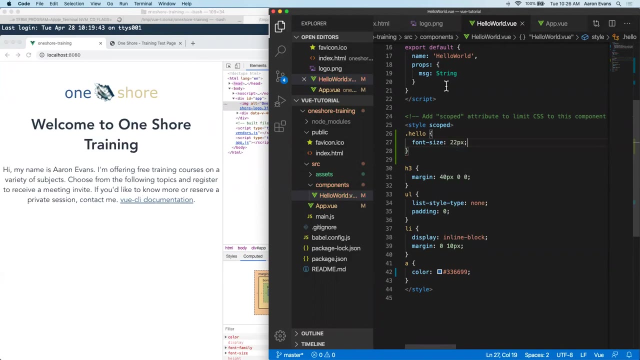 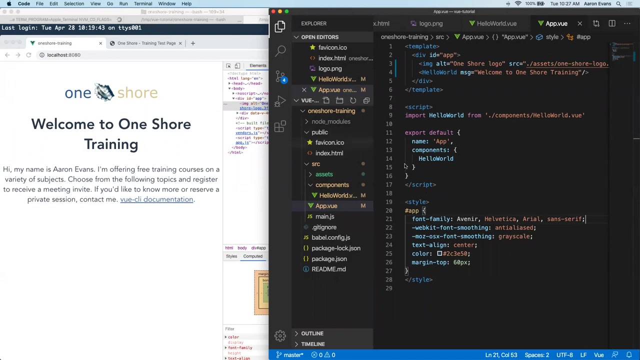 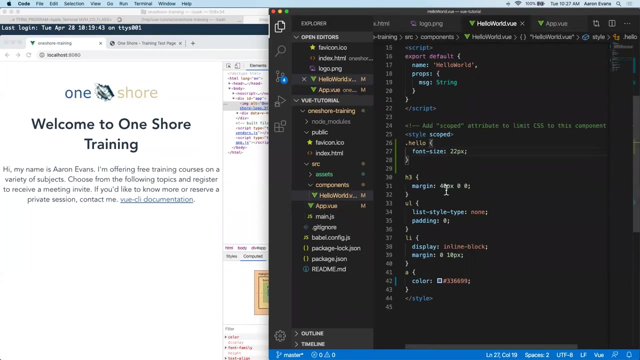 change our CSS here. so let's see is. is this in? what we want is we want our font size here to be, and we'll go back to our app and we'll remove that. all right, we want to change our, you, our display. why is this centered? 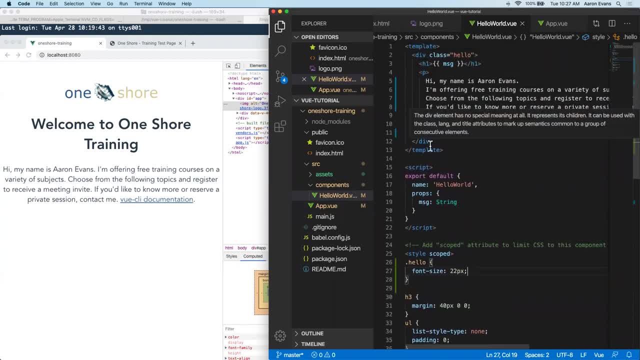 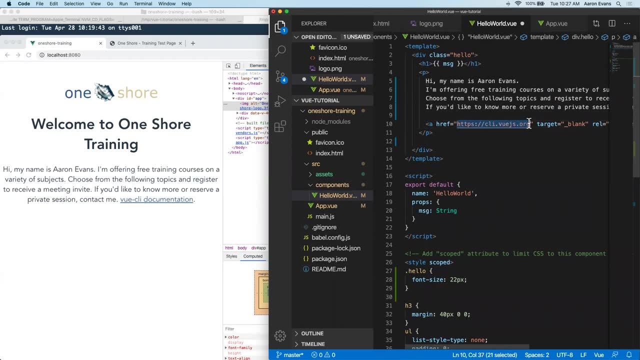 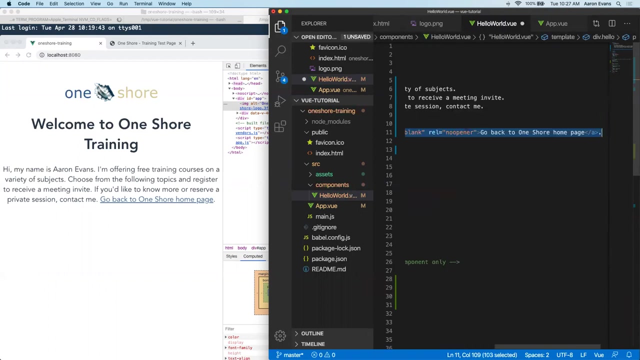 oh, and we don't want that view CLI documentation we want to go to- let's just go to- wwwoneshorecom here. um, um, we want this in another paragraph. so this isn't how I would normally do it. I would probably avoid the boilerplate and 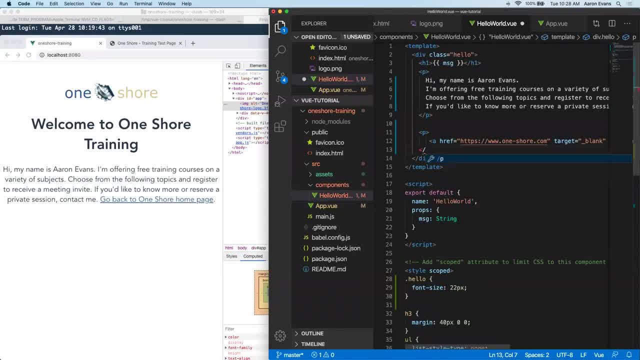 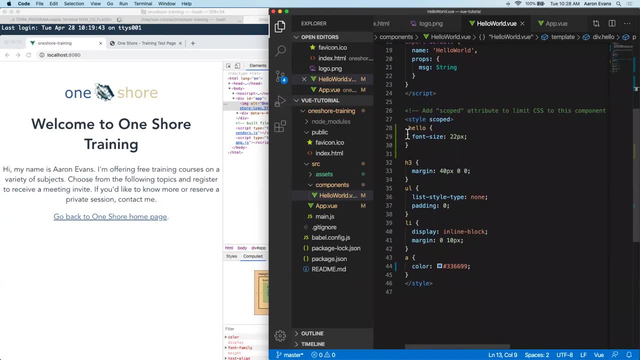 just start from scratch. um, I would probably avoid the boilerplate and just start from scratch. I'm studying my font size here. that's why I added on this element. it looks like I'm studying my font size here. that's why I added on this element. it looks like. 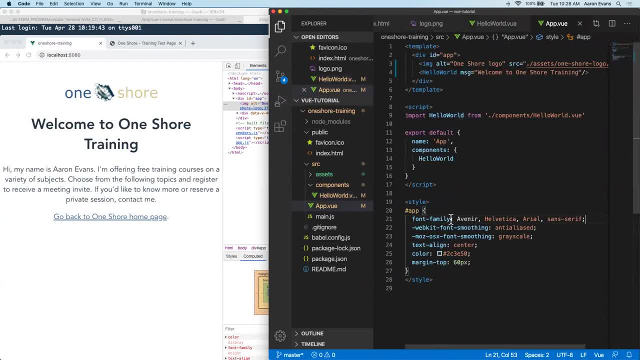 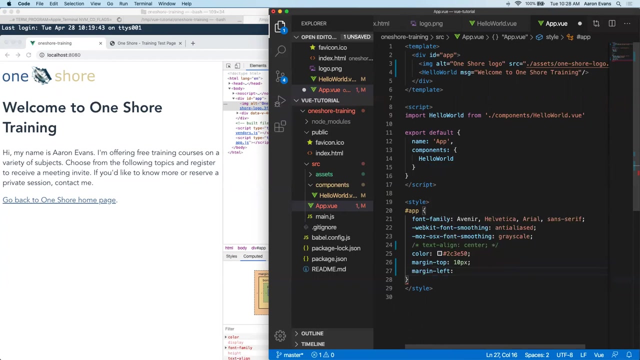 centered in the document. so let's go back to our app font family smoothing and alias grayscale text align Center. we'll just remove that, and then let's. let's add some borders. we don't want a margin top of sixty pixels, we want like 10 pixels. That looks good. And then we want margin left of something like 40 pixels. Let's. 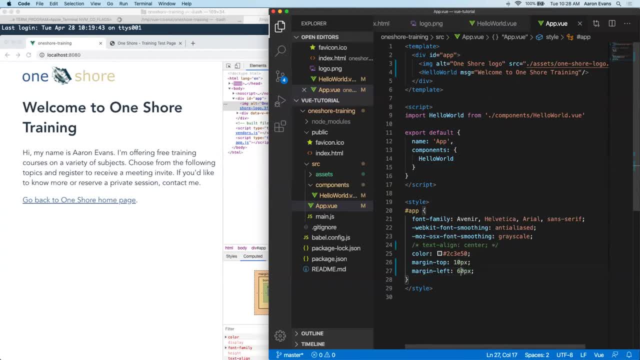 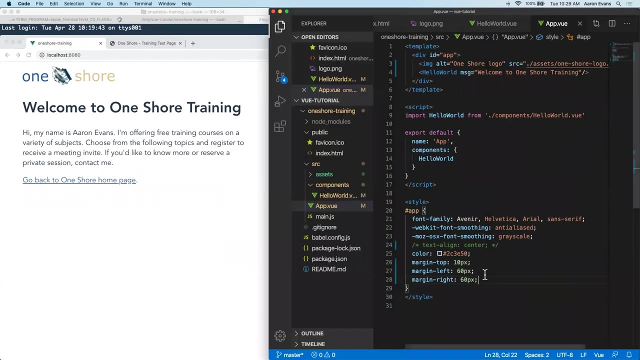 do more than that. Let's do 60 pixels And then margin right of something like 60 pixels as well, And let's do our margin bottom. Let's keep that like 60 pixels. for consistency, We want to use the top. Okay, It's looking like a pretty snazzy website now, right, Well, 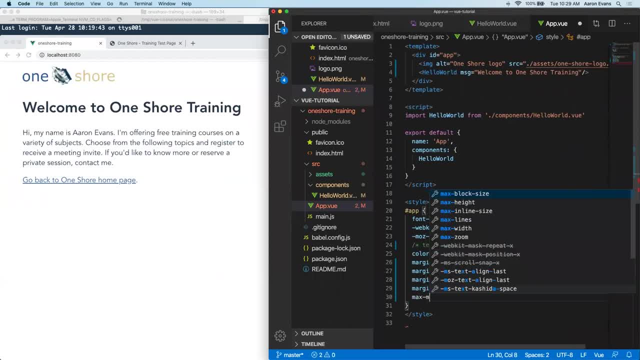 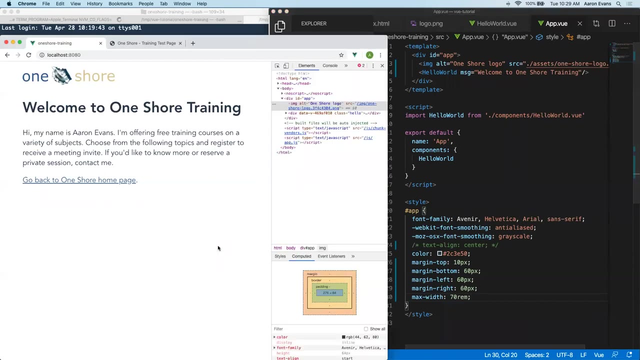 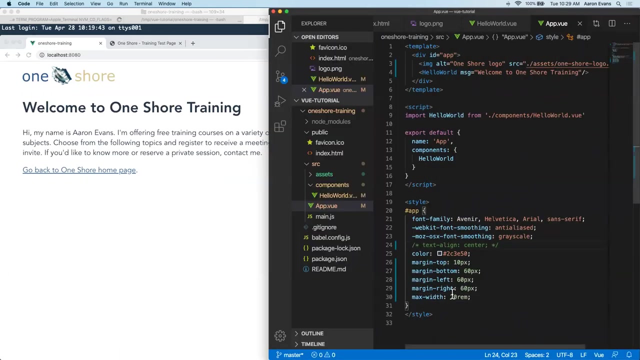 not really. But one other thing I want to do is I want to set my max width. I'm going to set that to about 70. So that way when I expand it doesn't get too insanely wide. Well, that's pretty wide, Let's go to 50.. That looks better If you go huge. this content. 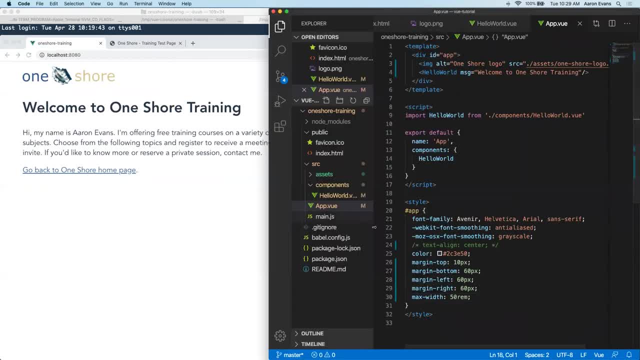 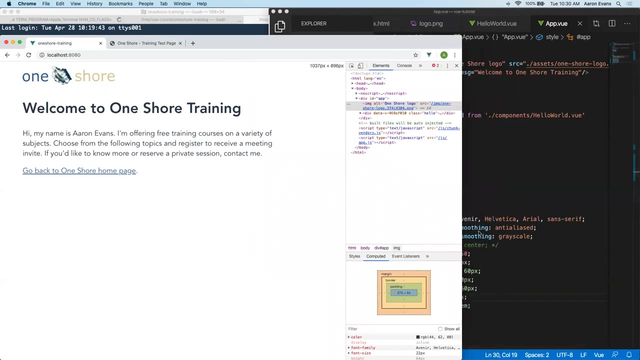 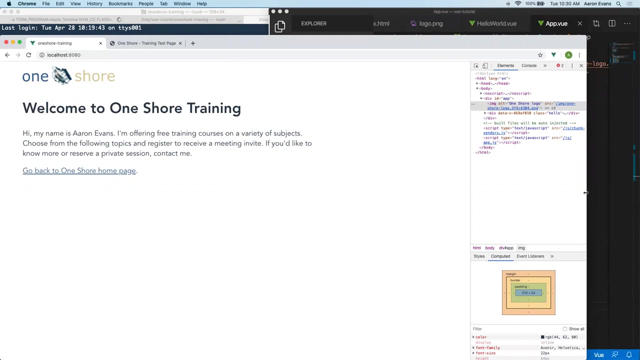 isn't going to get too huge. All right, Okay, Okay, And then let me, so that we tie this to something. Let's see if we can get variety of subjects on the same line. So we'll go: 55 rems, There we go. That looks like a pretty good. 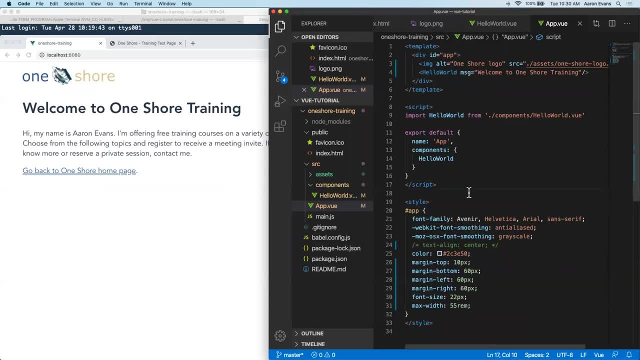 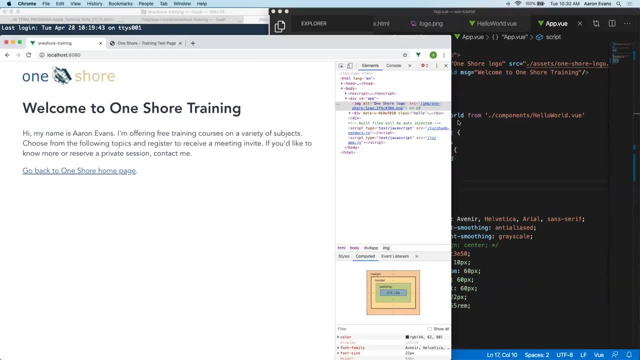 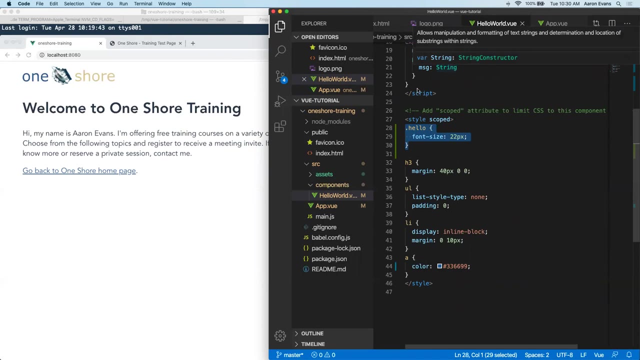 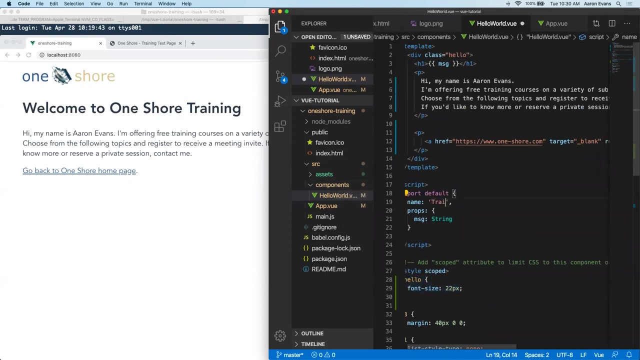 width to me. Okay Didn't mean for this to be a CSS basics course from someone with no design skills, But that's what it's turning into. What we've done is we've created this hello world view component, But we don't really want a component called hello view. We want a component to list our training courses. We could change this. We could change this to training header. 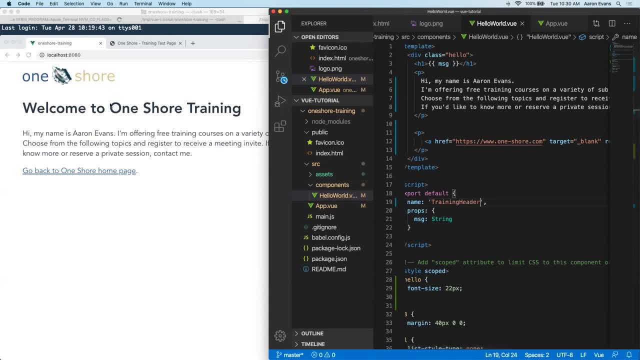 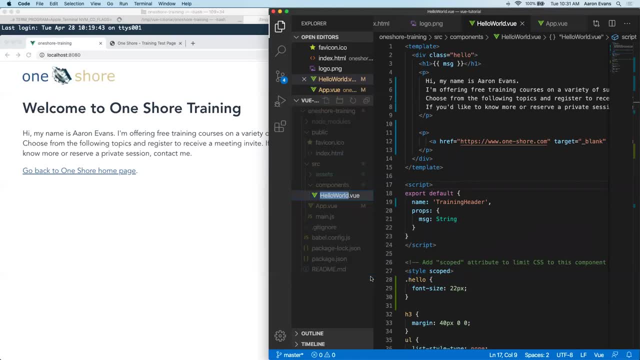 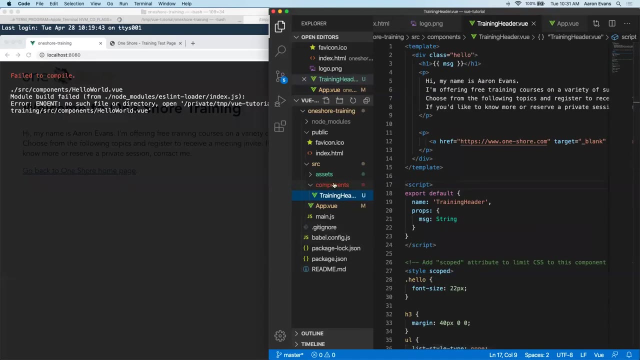 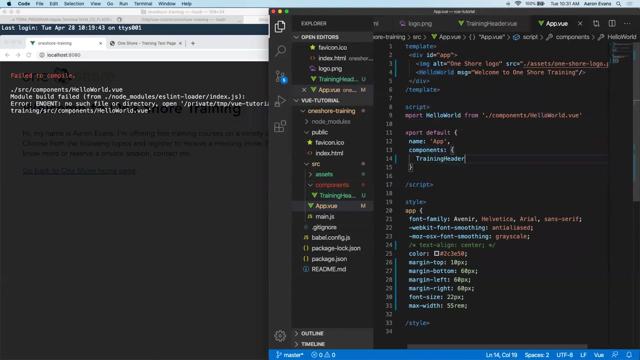 Okay, Now we're going to get a compile error. Let's rename this. Now we've got a compile error. How do we fix this? We go back to our main app and we change our component from hello world to training header. Still not going to work, because what we're trying to do is we're importing hello world, So we want to import training header. 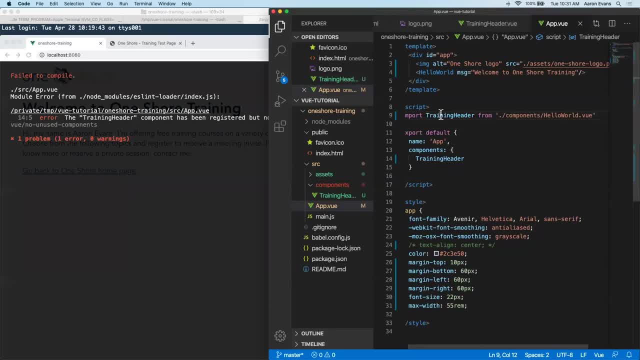 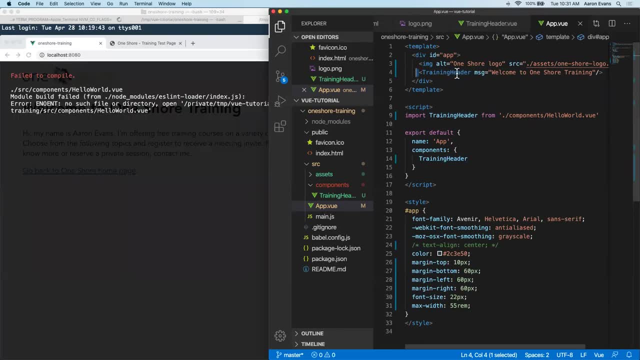 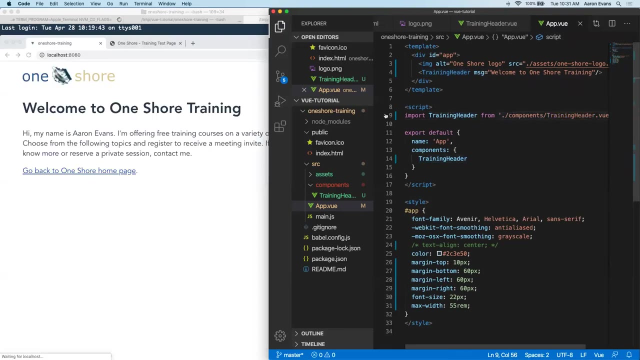 Then we search for training header And the component. we're called this, this component, rather than the image or the div or a hello world, it's called training header And of course, we just need to change the file name And we're back in business. So now we have an app that imports this training header component, Which, pretty basic, It has a ton of scope. 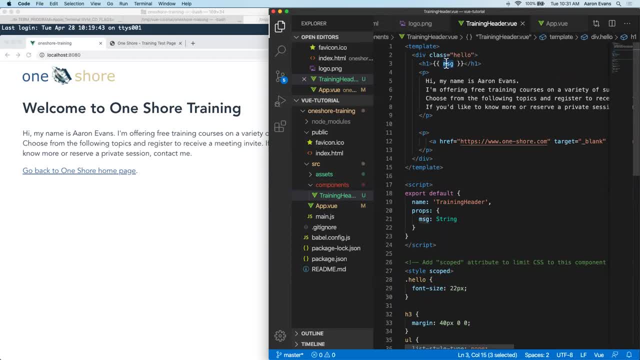 We can change it. No here, No, no, Never mind, Okay message. we'll call this message. we'll change this to title. right, so now it disappears. we don't have anything called title. we need to change this from message to title. it's still not working, but this is, this is a property that. 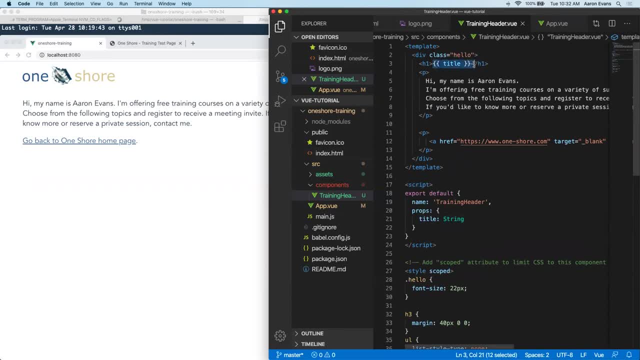 we're setting in our script and then we're getting it in the template, but where is it getting set from? right now it's just saying it's a string, but what we want to do? we could set it to a value. nope, it should be a. 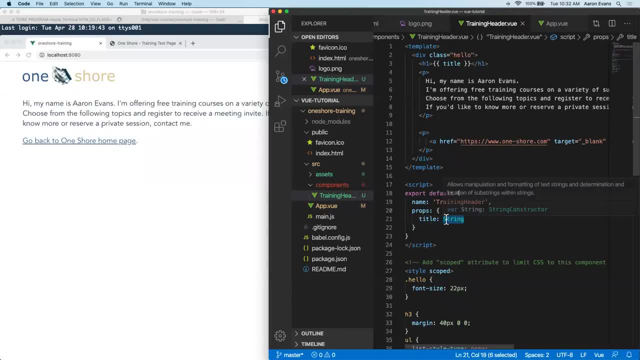 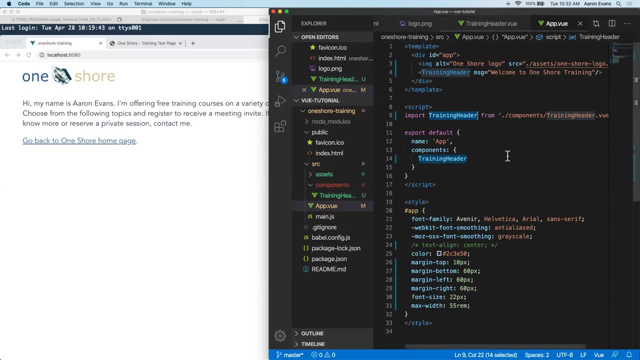 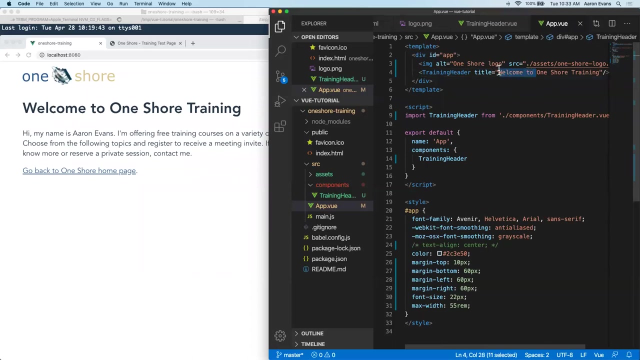 constructor. so strength is the type. now we go back to our main app view component, our app level or our root component, and here we want to set our message here. so this is like a parameter or not message. we want to set it as title, so we can call this one: short train courses. there we go, so you. 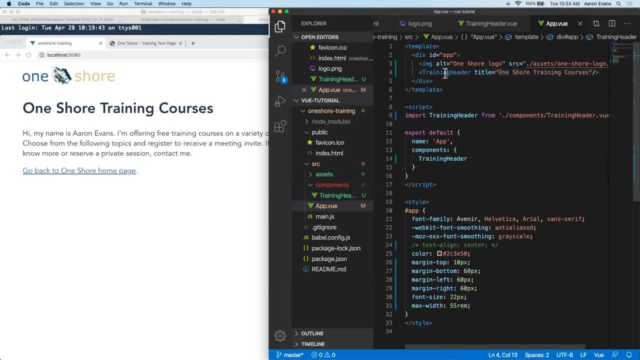 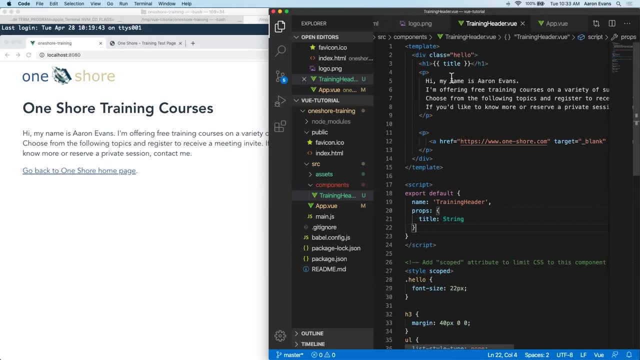 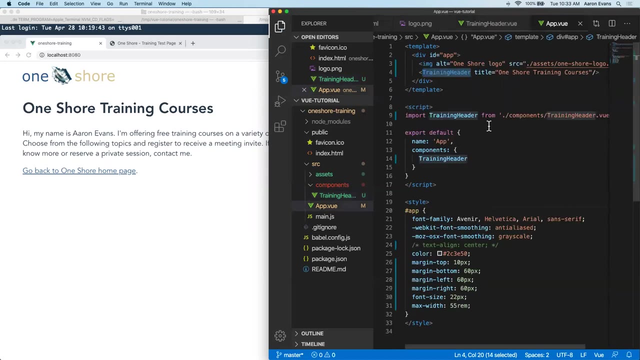 can see, the title is an argument to here, and so it gets it in the properties sets it, and then we're able to get that in our template. so this can be done dynamically, right, but right now we're just passing it as a property. we could actually take it and 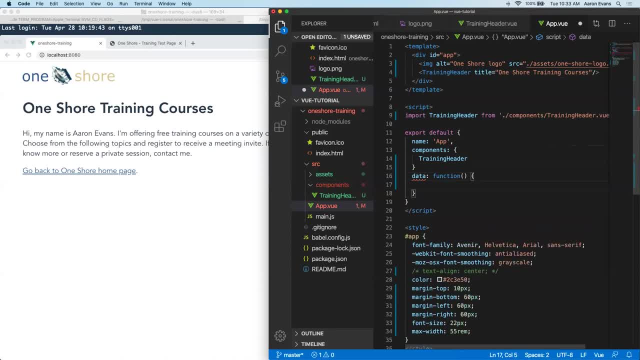 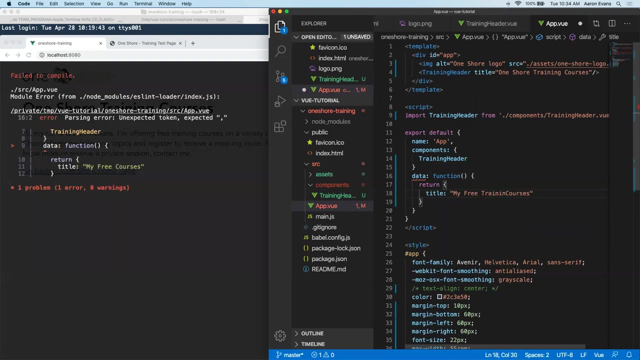 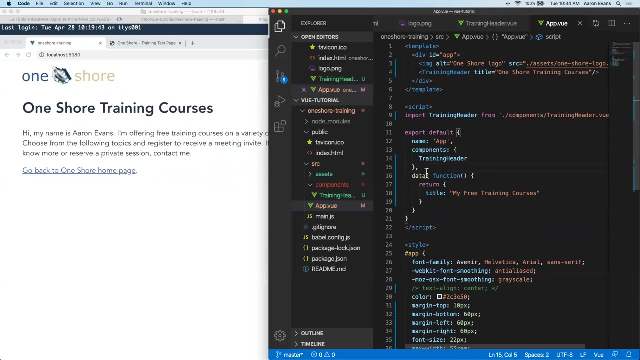 we could create some data and we return an object with title here. so title sorry, I could call this my free training courses. okay, what is it not like? module error: expected comma. oh, first comments: comma data. there we go. okay, so it's not getting my free training courses. 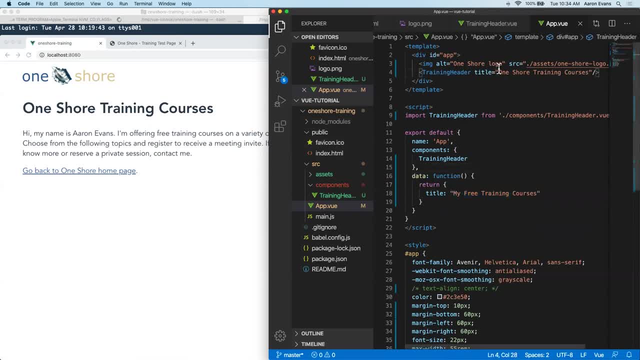 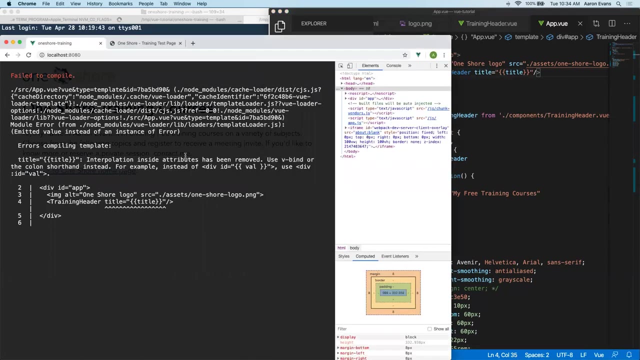 free training course is here because it's coming in the title. But I can actually here. I can use a template in this component And I can put that here. I cannot put that here. Errors- What did I do? Interpretation inside attributes has been removed. Use vbind. 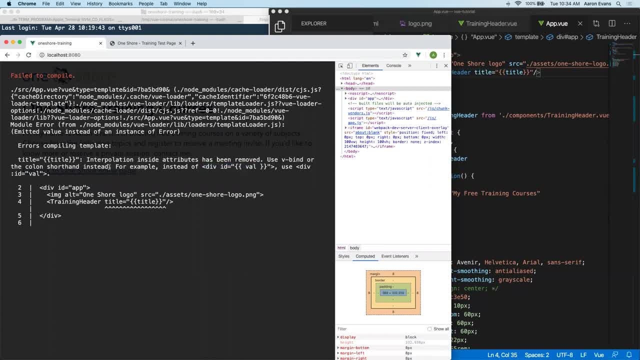 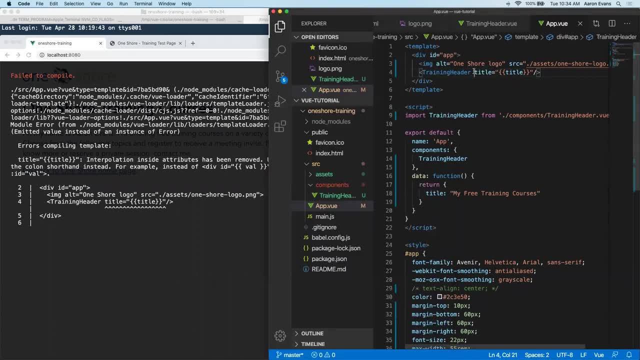 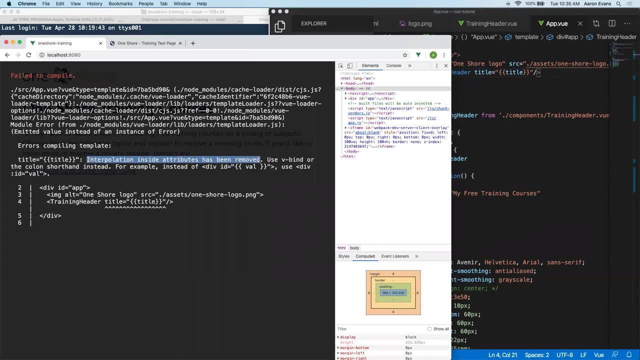 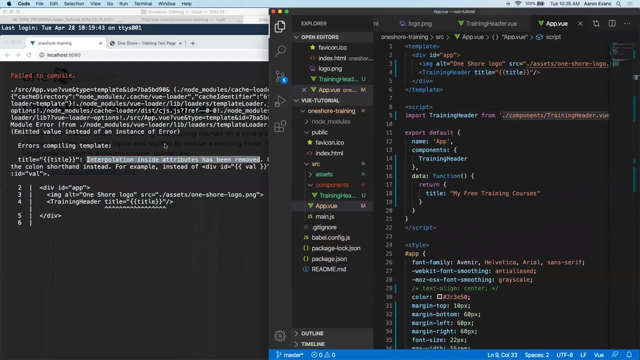 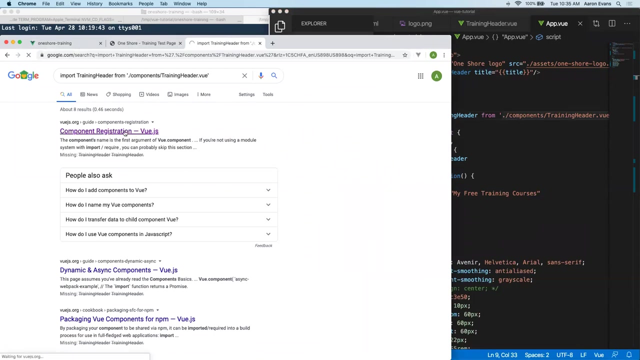 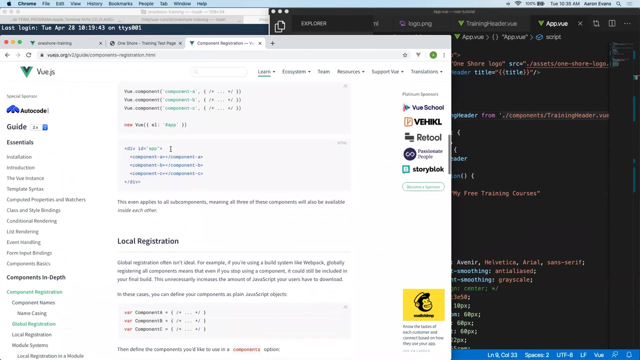 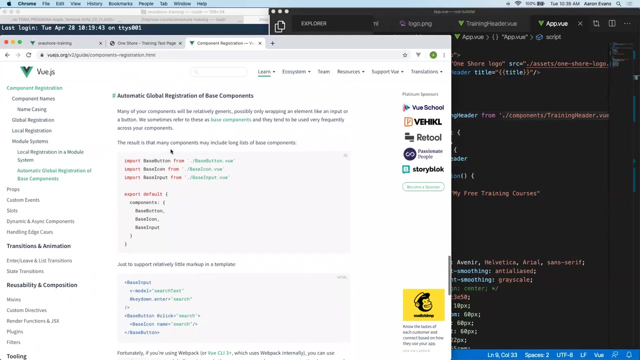 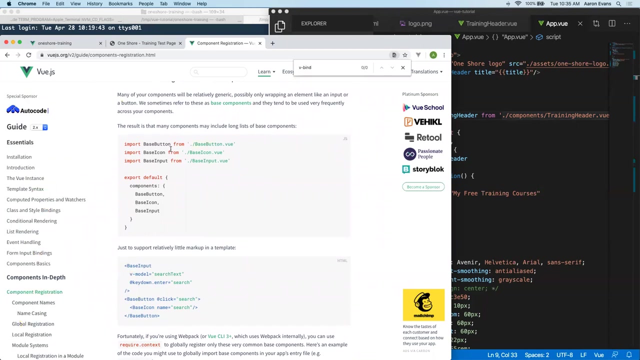 or the colon shorthand instead of div ID Use. div ID equals value, So it doesn't like. all right, Let's look up this issue. I think it's just a matter of that. you can't do it to components, All right. That's not even showing us what we need. 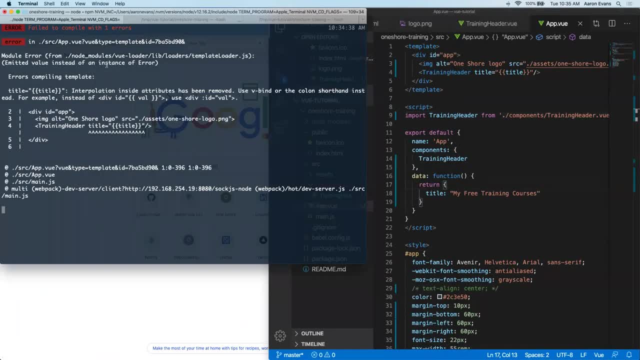 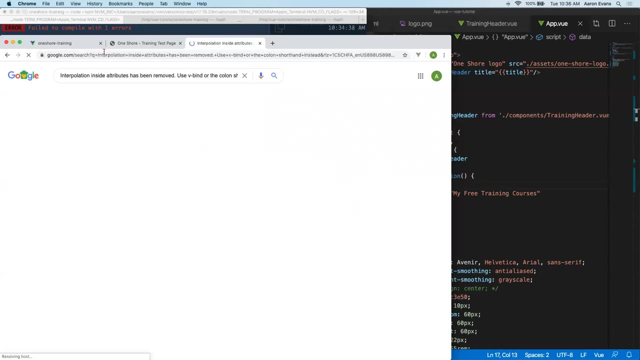 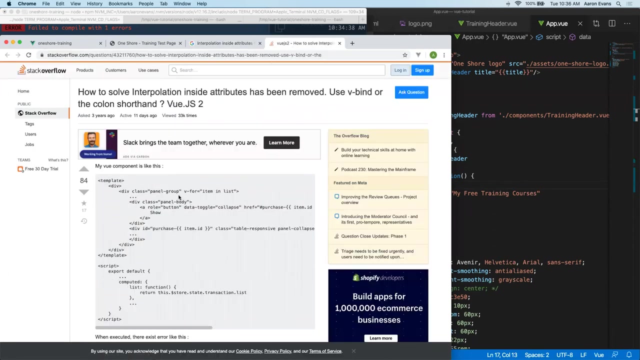 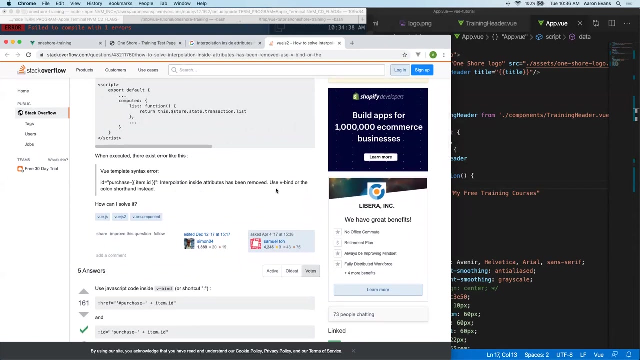 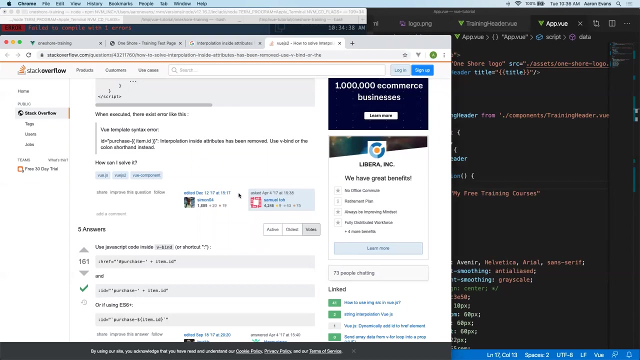 Oh, it's not even. it's not. even certain Interpolation of attributes has been removed. All right, This is a new change Three years ago. This is not new. All right, There exists an error ID interpolation inside, So we put a colon in here. I guess what I would do is I would do colon title. 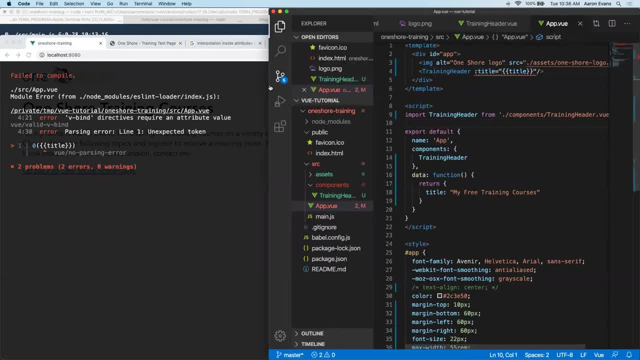 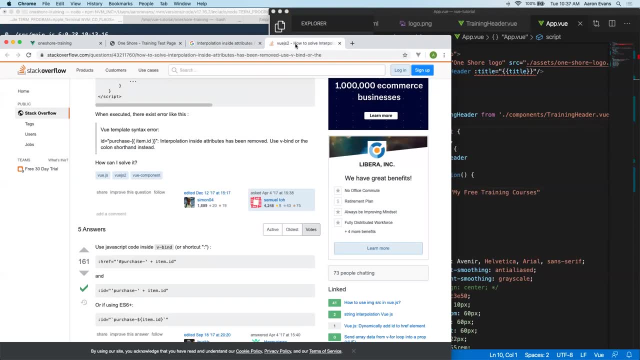 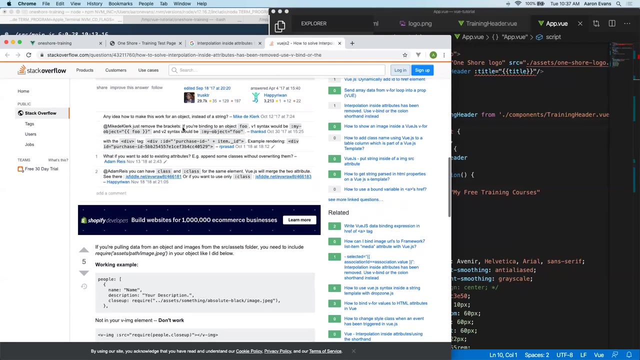 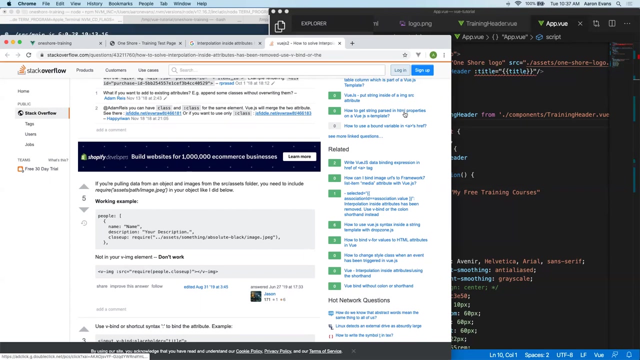 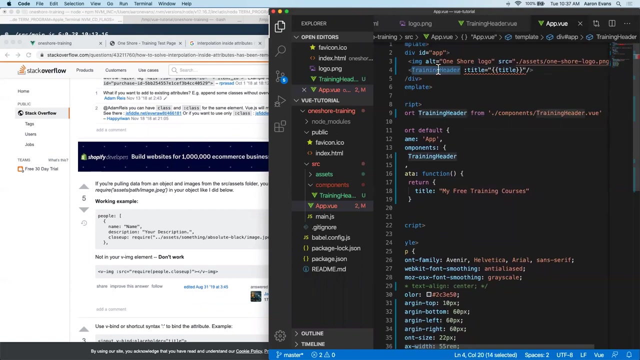 No parsing error. So yeah, It doesn't like binding inside attributes And I think the real issue here is that it's an attribute to a component. For instance, if I add a p, maybe if I had an input value equals. 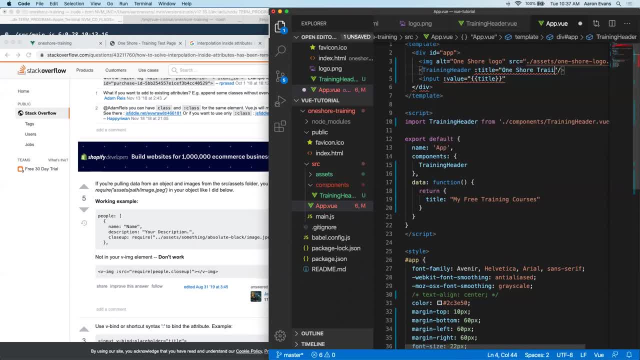 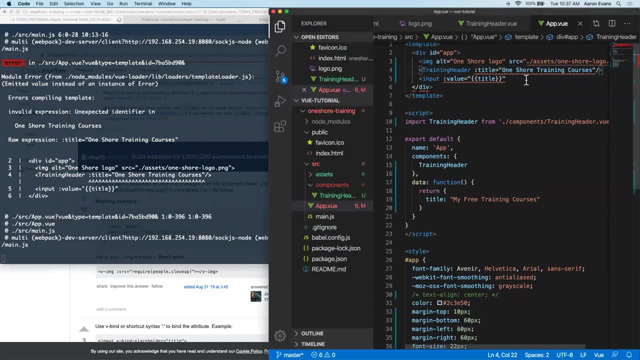 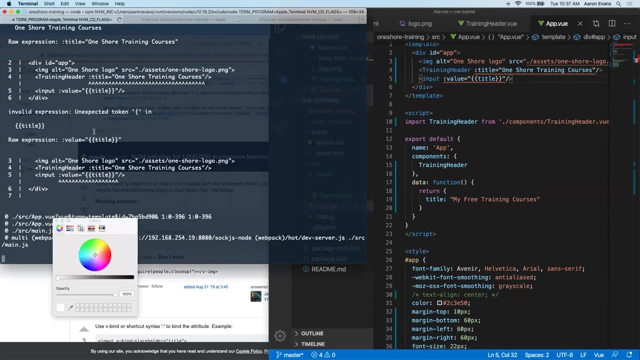 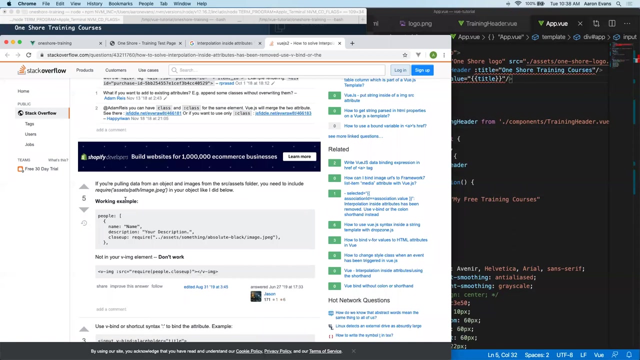 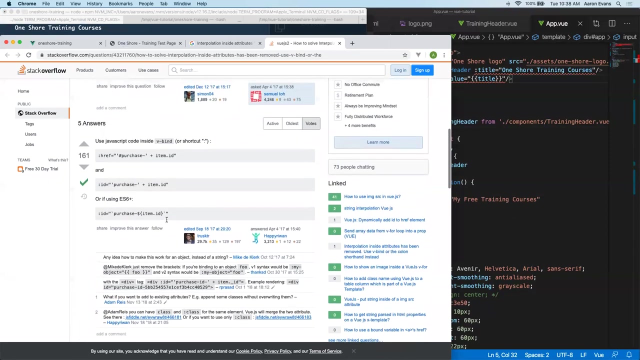 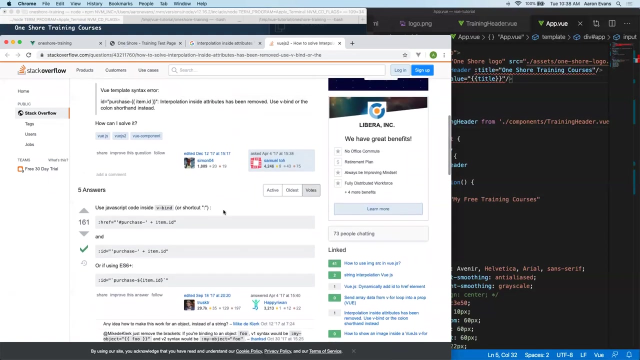 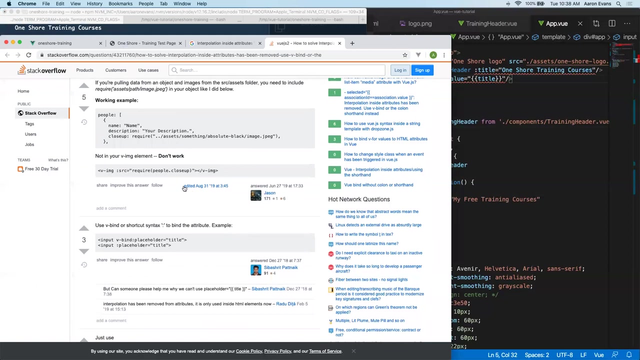 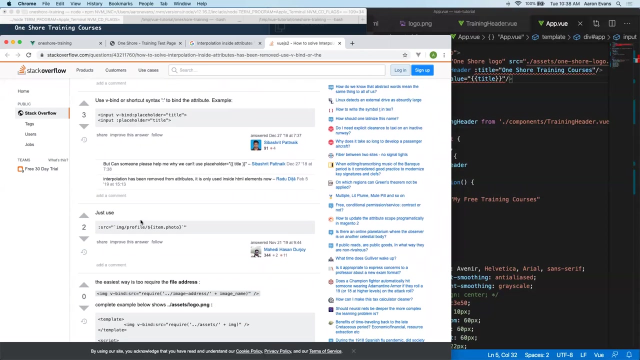 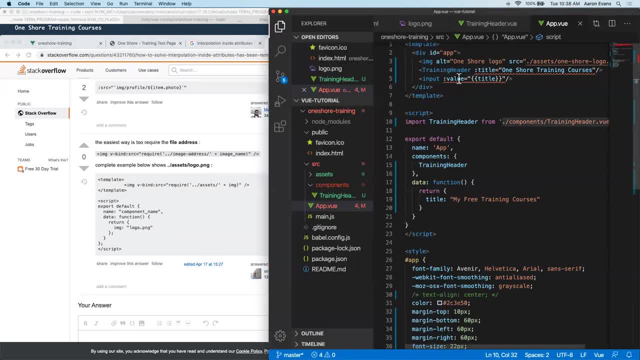 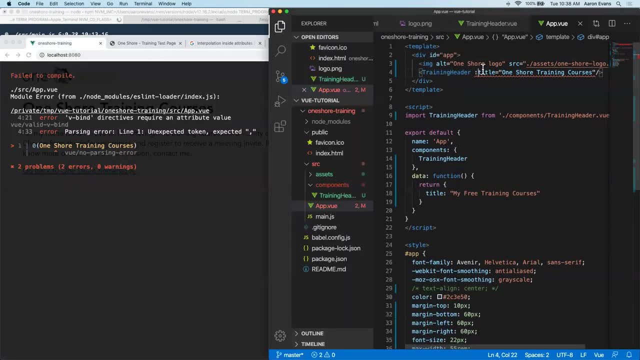 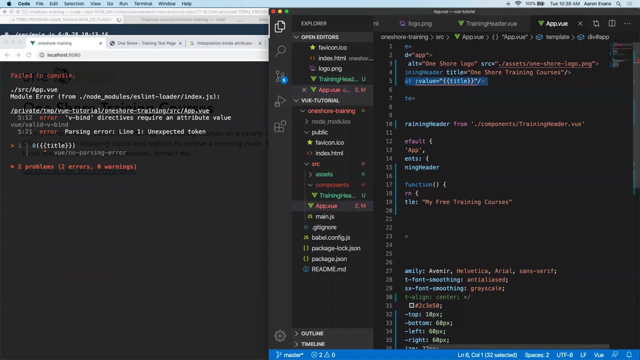 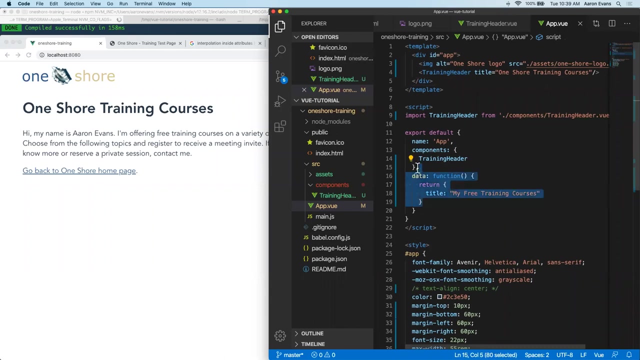 I don't want to require something. All right, let's ignore this. This isn't something I needed to do anyway. All right, so we're back to one: short training courses, So ignore my whole comment about the data and the component. 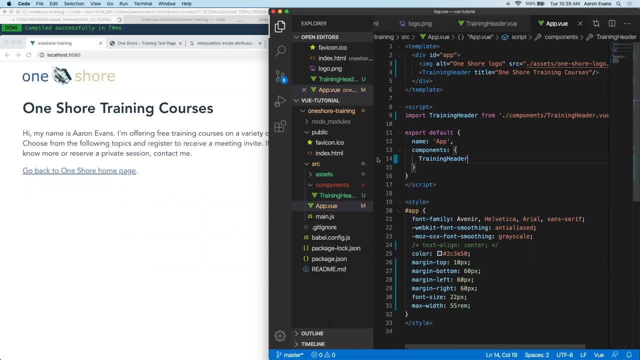 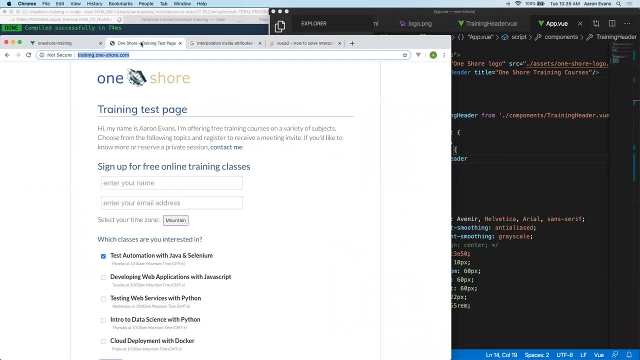 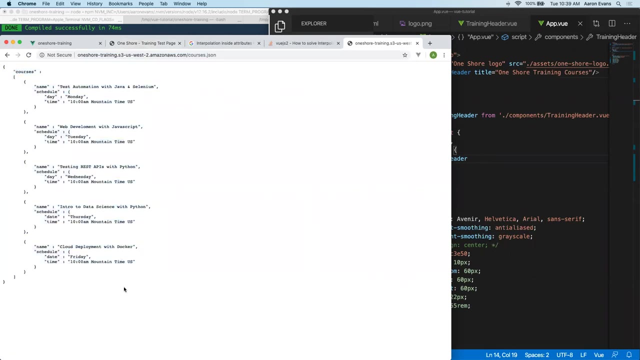 For some reason it won't pass that. just a typo there. Okay, so what I want to do is I want to create another component that will list my data, so my courses. I also have this S3 bucket, which is JSON. 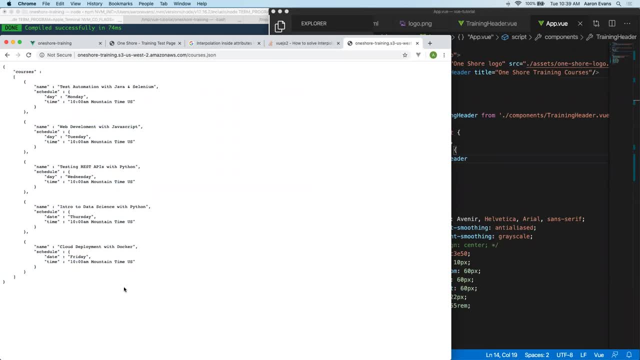 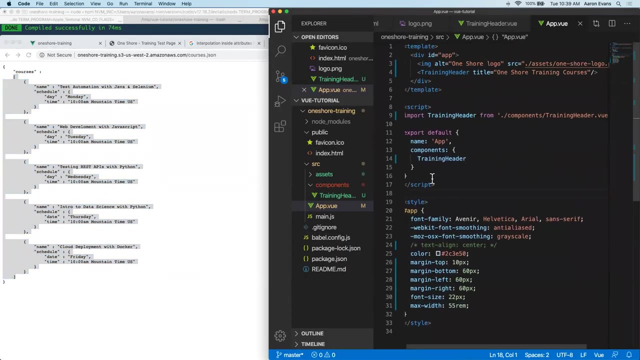 What I want to do is I want to get this JSON and print it so that I can update my JSON and it will update my page. So let's just start off. I'm just going to grab this content here And within my script. 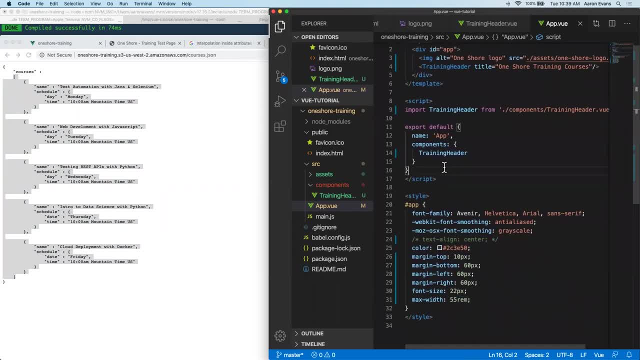 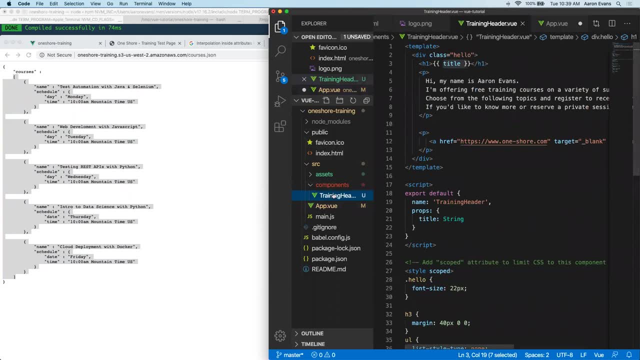 Actually not in my script. Okay, Okay, Not within this script, Within my new script, I'm going to do that, But the next thing I want to do is I want to just copy this component and I'm going to rename this, to course. 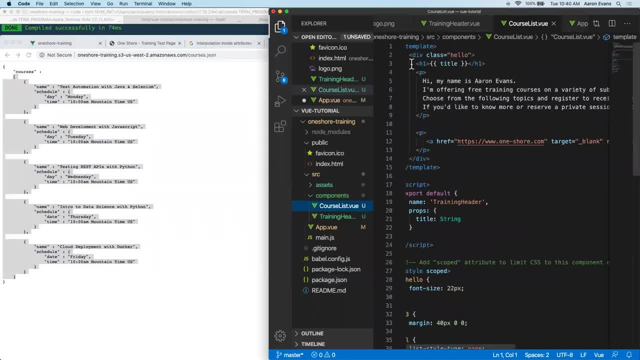 Let's call it course list. All right, let's go ahead and clean everything up out of here. I just wanted to show you. So we start with a template, a template with a root element. It always has to have a root element. 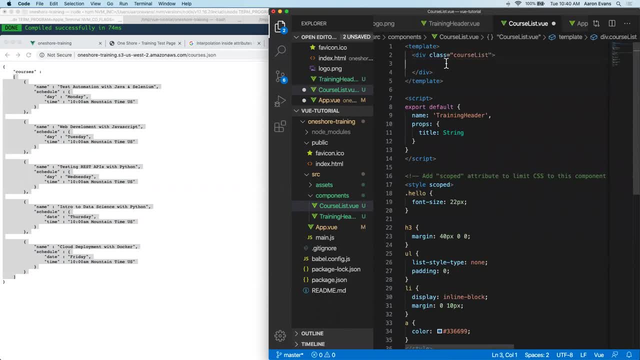 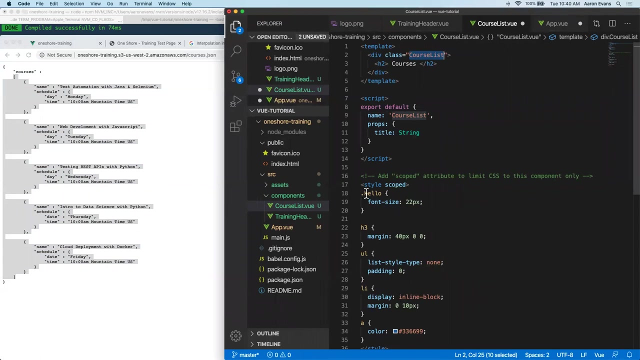 Let's call this course list And we'll just start off with it saying courses. We need to change our name to course list. Let's keep our class, Our file name, our CSS class name, our component registration name, All of this. keep this all. 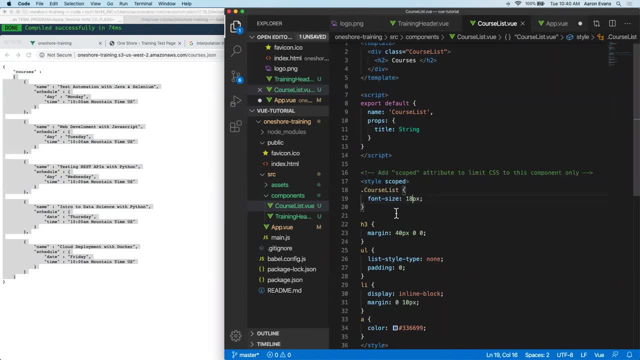 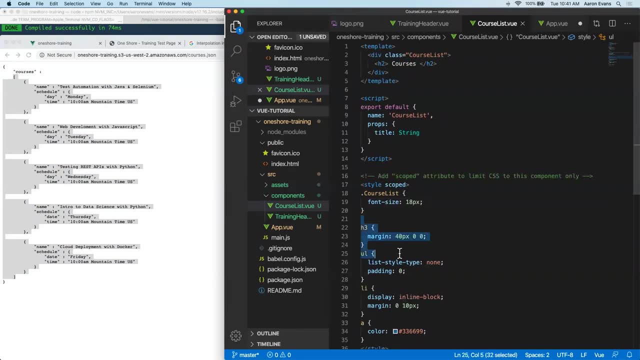 And let's make our font size a little smaller for this. Yeah, we do want to keep our list and our link here. Okay, what have we got? Well, we've got an H2. Font style: underline font. 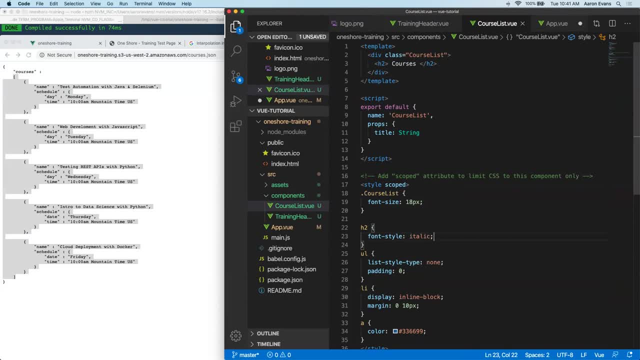 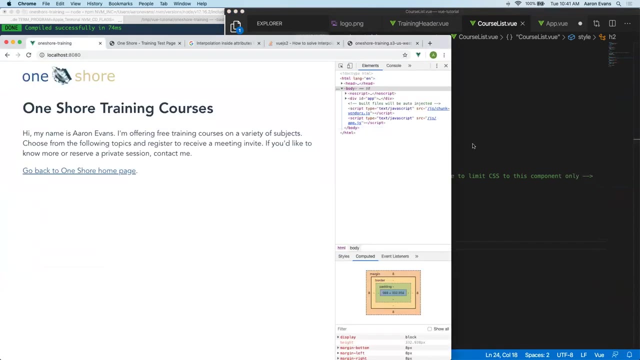 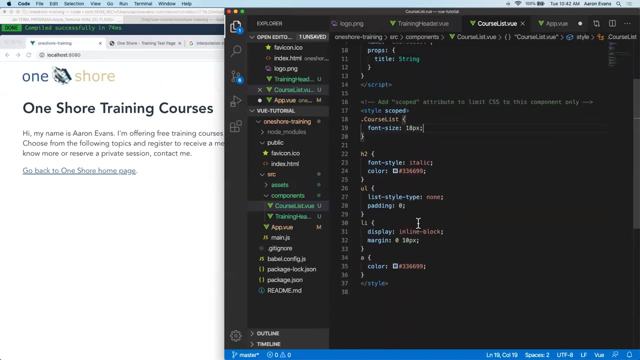 Just so we can see that it's getting registered. Oh, and then we want to go color 34. 33. let's look at our. okay, we want this to be three, five, six, or three, five, three, six, nine. okay, we don't have our, we don't have our component here yet, so this style, it's not getting attributed. 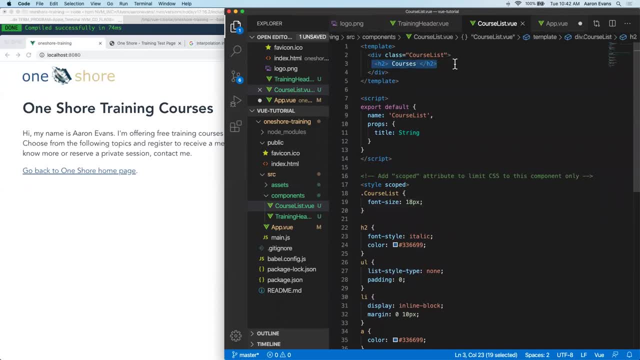 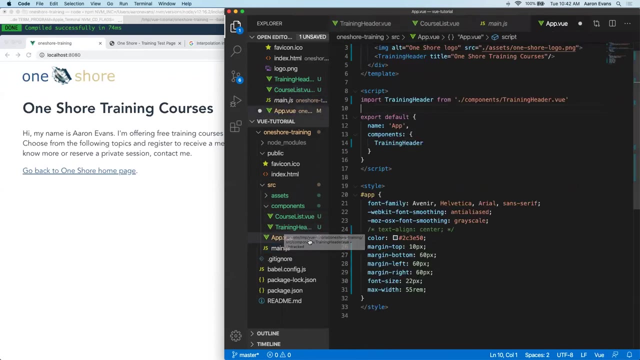 because it's not displaying, so we have nothing here. our component consists of just a single container div with courses heading, so let's go ahead and add this. we've got a course list view. let's go back to our- yeah, our- app view and what we want to do is we want to add a course list. 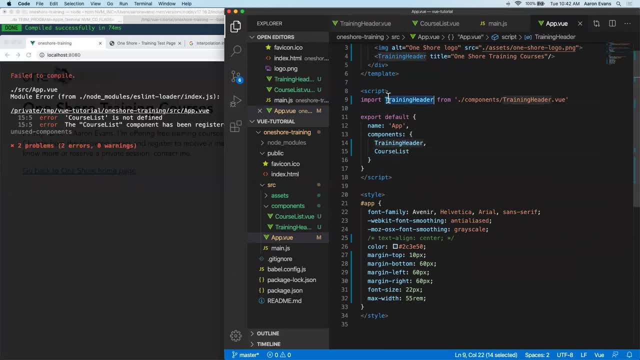 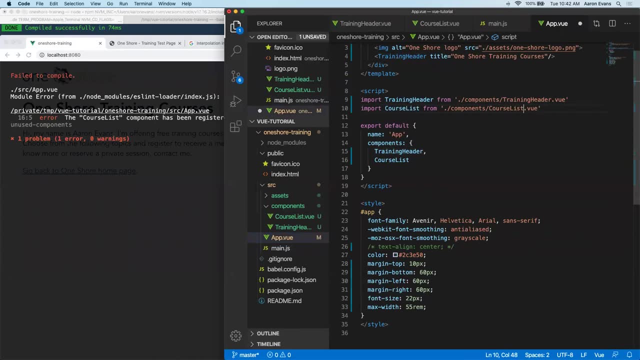 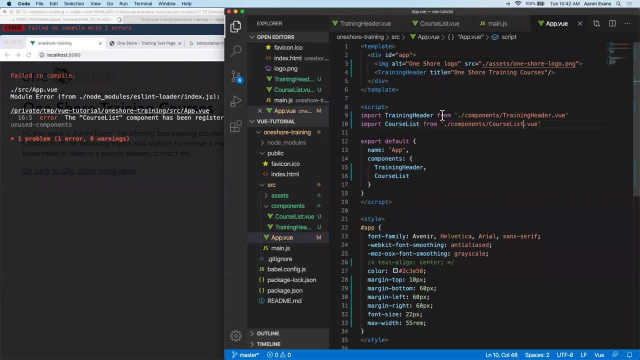 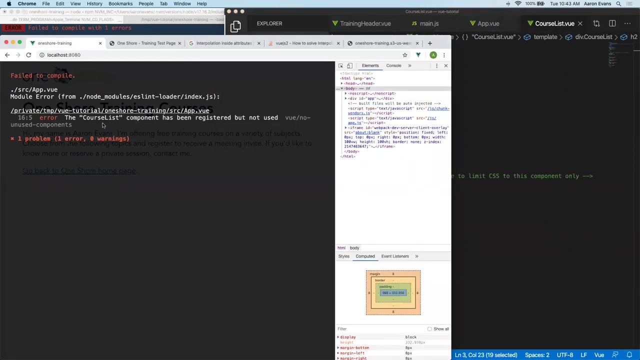 to our components. now it's not defined, we need to import it. there we go. so doesn't like what's going on here. the course list component has been registered but not used. well, that's kind of rude. we probably don't want to be that strict, but 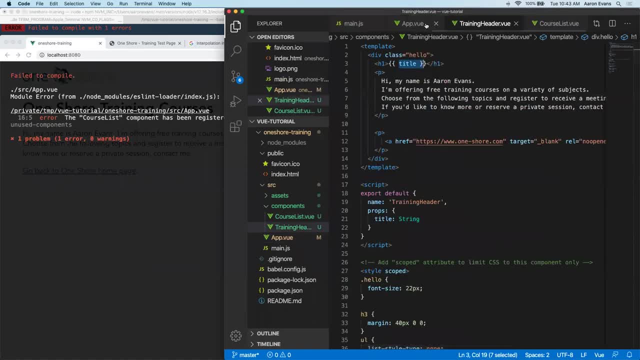 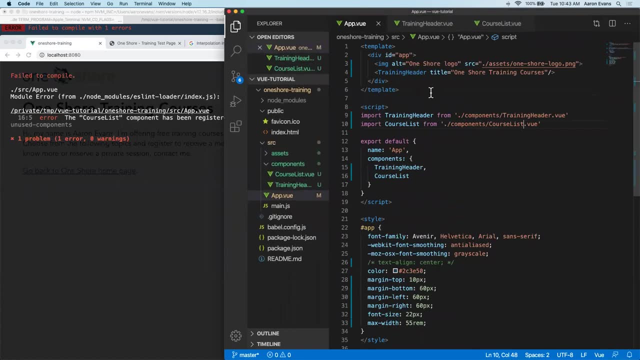 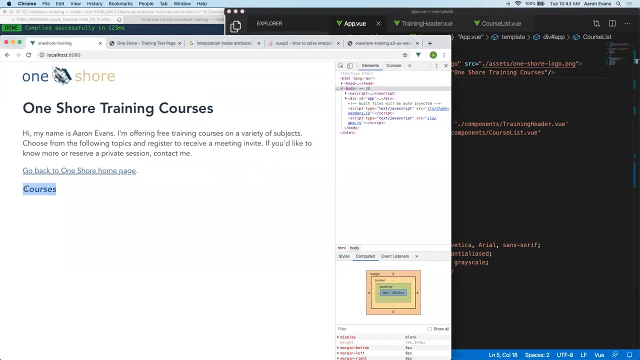 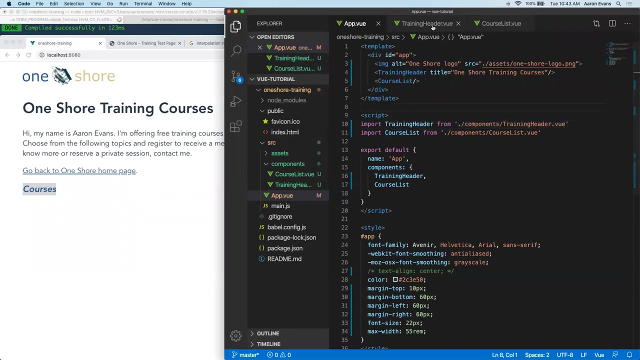 you all right. so we want to add our component and we'll do it just like that, and we have courses and it's an italic, which we don't really want, but we did it for fun, so let's go ahead and add it, okay? so once i edit this thing and i close the application, i just wanted to address a few. 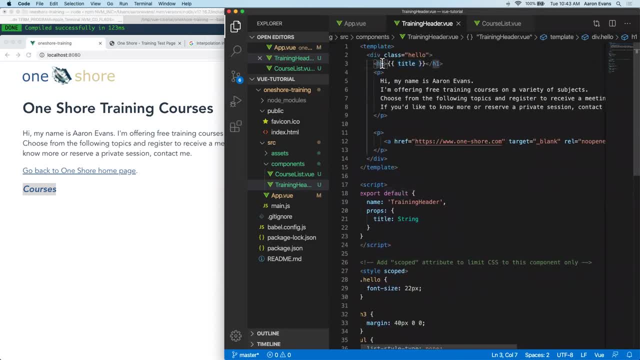 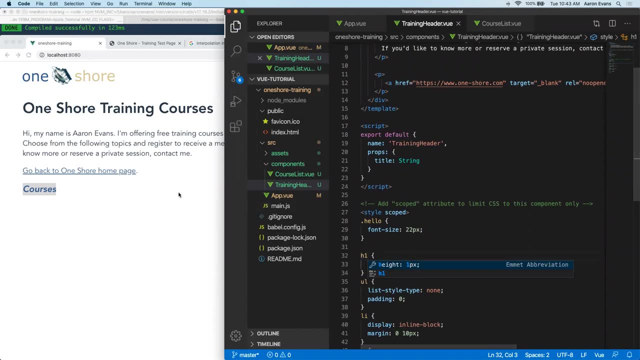 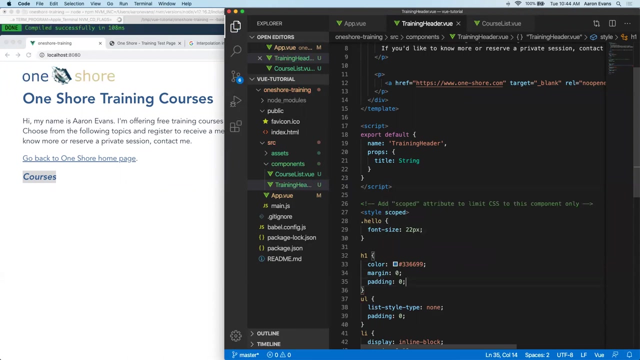 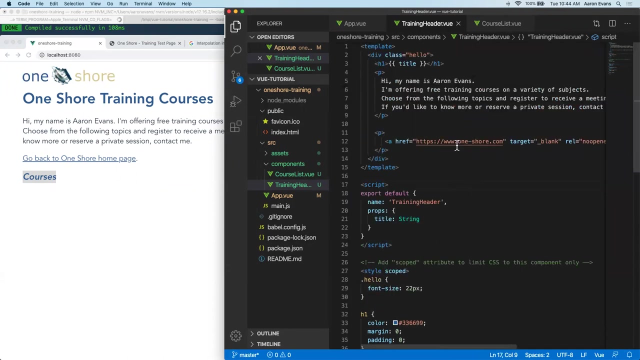 more things: um. on our training header. we want to um. does it have an h3 1h2? has an h1? um? first, we want our color. we talked about that before. Margin zero, adding zero. all right, And since we have one short training course, we don't need our. we don't need one short. 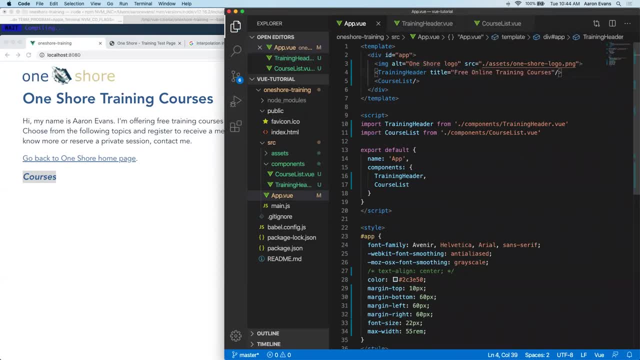 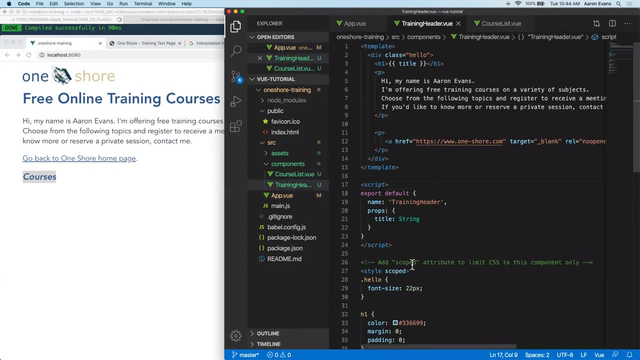 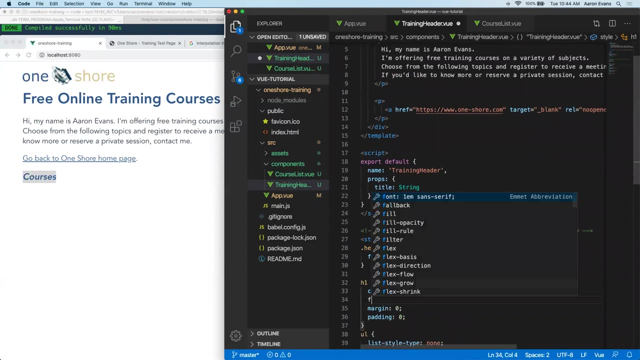 training course. We just need three online training courses And we want to change those margins. we also want to change our font size- Font family Radana- be consistent with our logo font weight- That's normal. And then we want a margin. 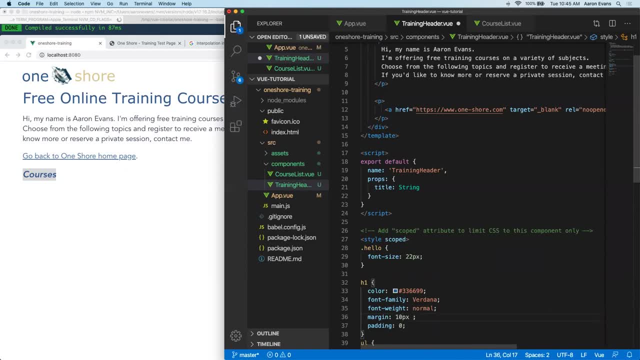 We want like a 10,. we want a margin, top of 10px, I think, and a bottom of 10px. well, let's do 15,. well, let's do this relative And padding. we want zero, zero. 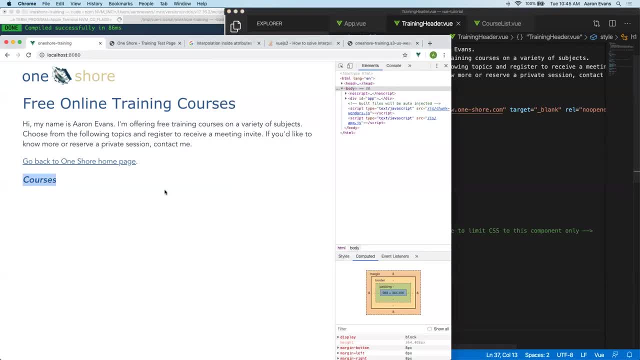 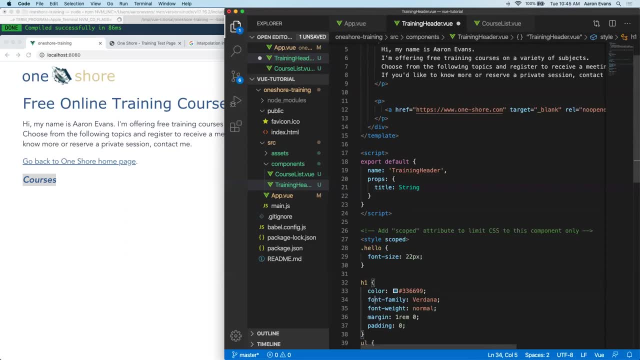 Three online training courses. font size. font size. I don't know what this is, but let's make this two. let's do three. no, let's do 2.5, all right? well, we'll stick with two. 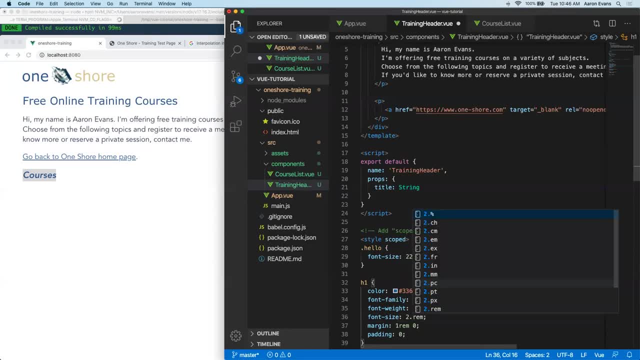 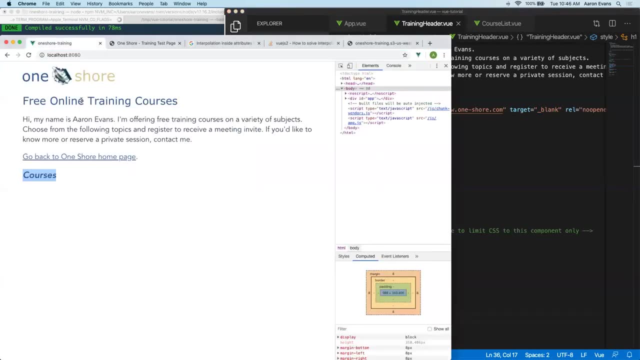 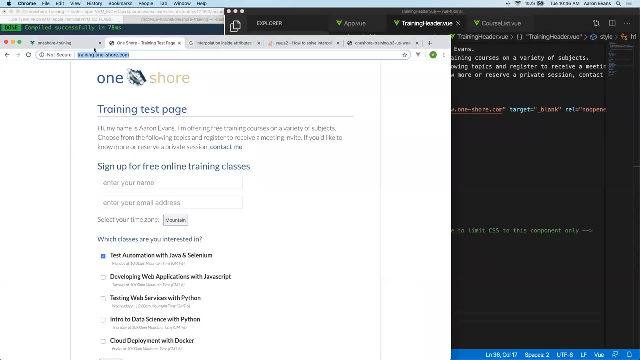 since we don't want that, All right, Let's move on to the next one. What does it look like on public? Pretty good, We've got a different font there. Okay, Free online training courses. Hello, my name is Aaron. 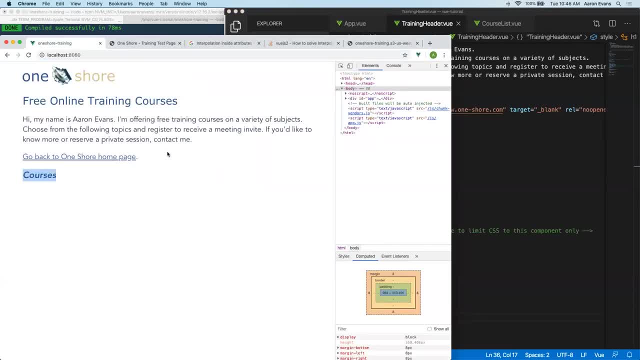 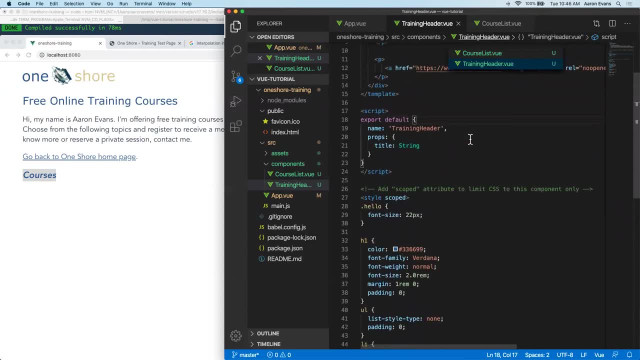 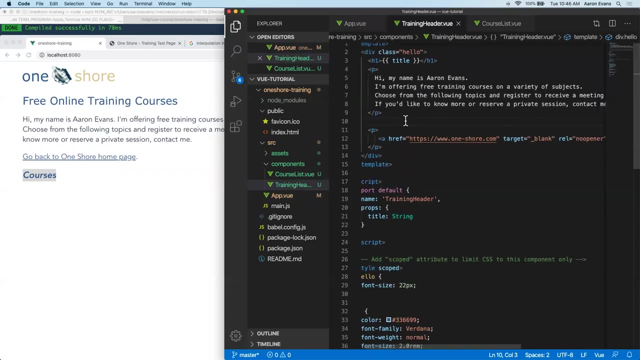 Sign up for free online training courses. We can remove this. go back to the OneShore page. We want that bottom. I'm not sure how to yield, because what I'd like to do is- oh, I do know what I would. 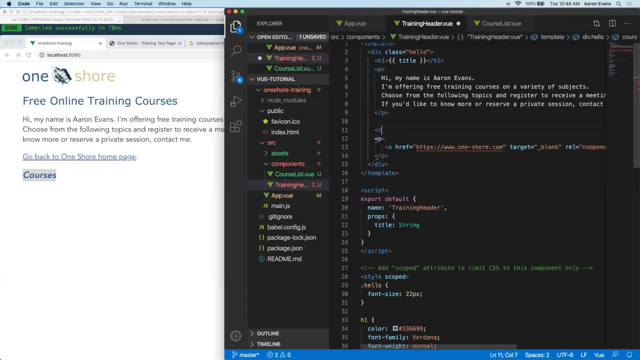 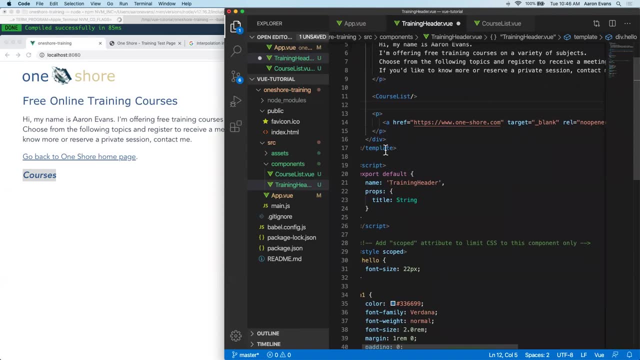 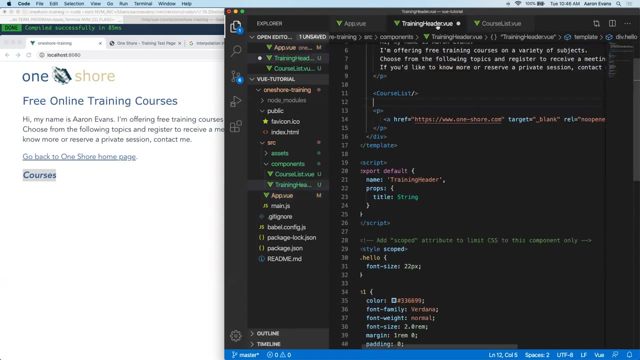 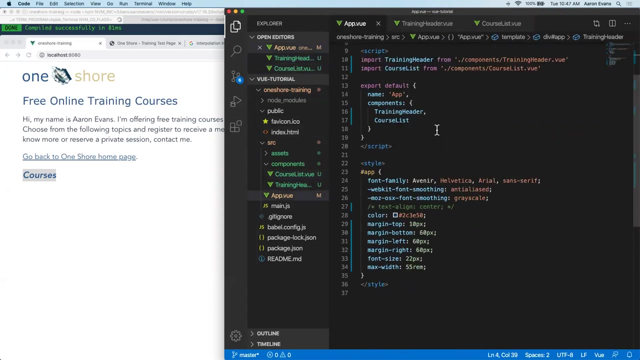 do is I would put my course list here. So let's do that. Let's remove the course list. Well, we're not going to do that, Not today, But oh, All right. All right, So we're going to remove this from the training header and put it in a Flitter. 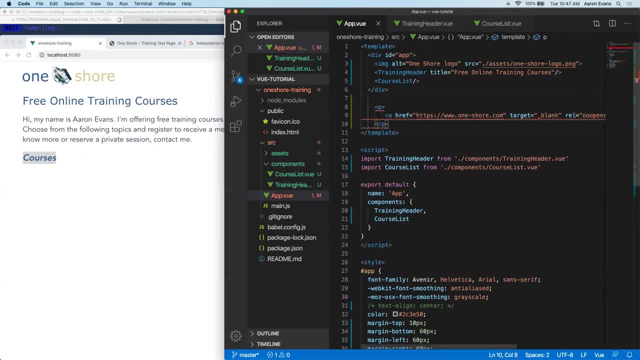 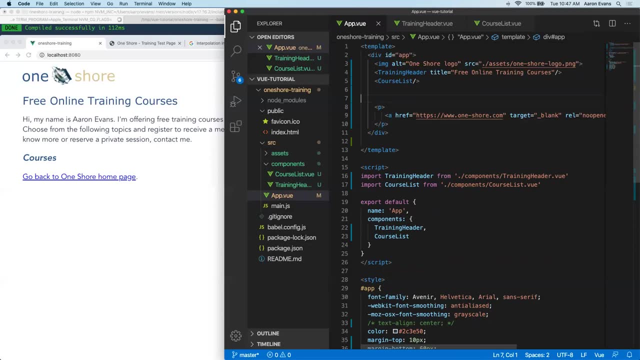 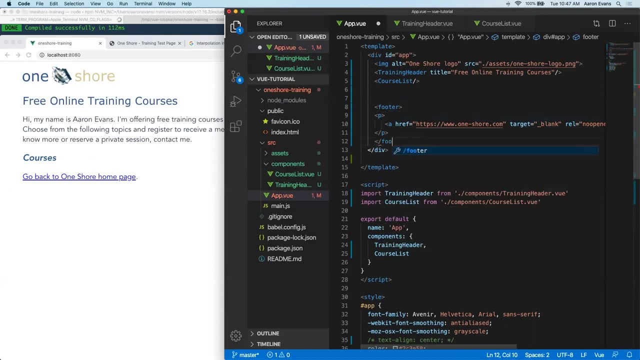 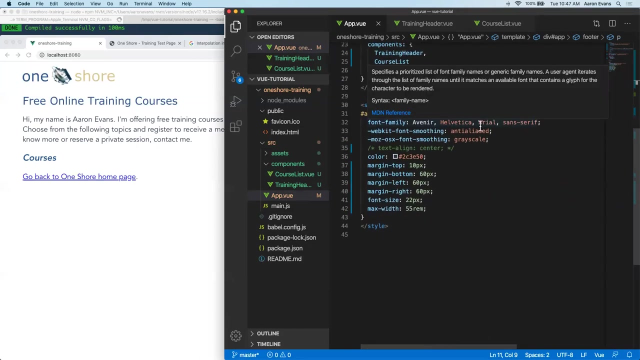 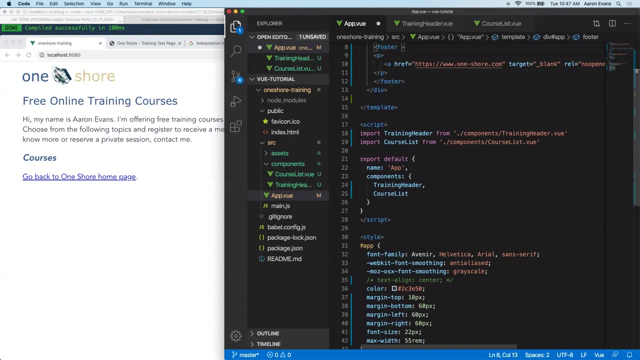 Maybe down here, And what you can do is you can, in your template, create HTML and eventually move it out into a template, And then you type in your code Into a component. All right, How do you do that? CSS? 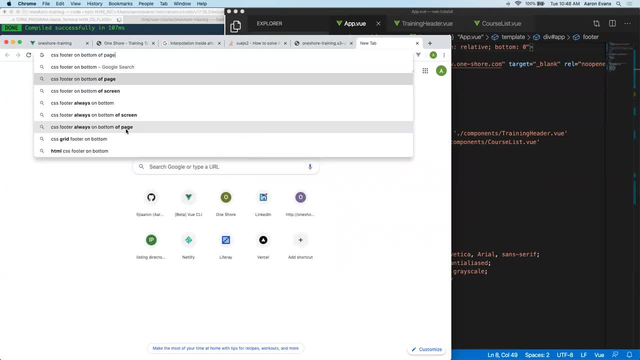 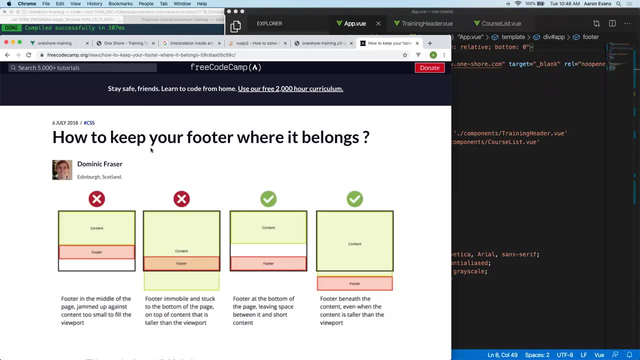 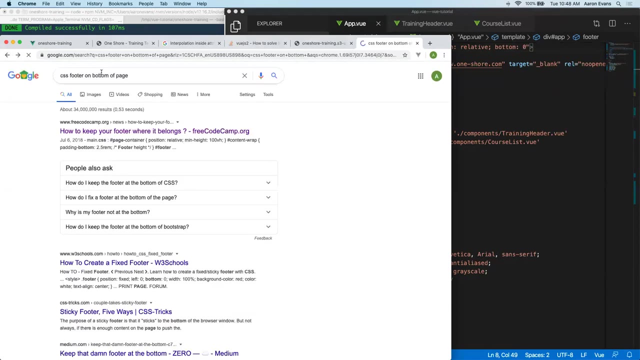 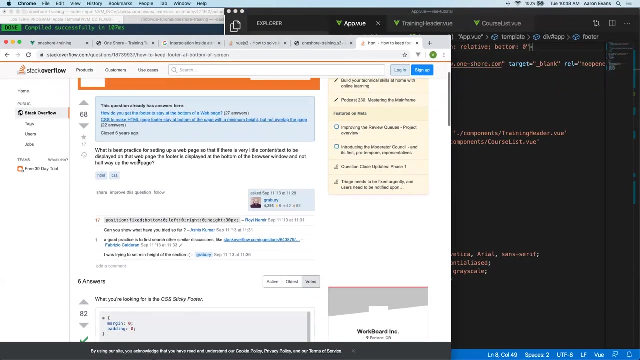 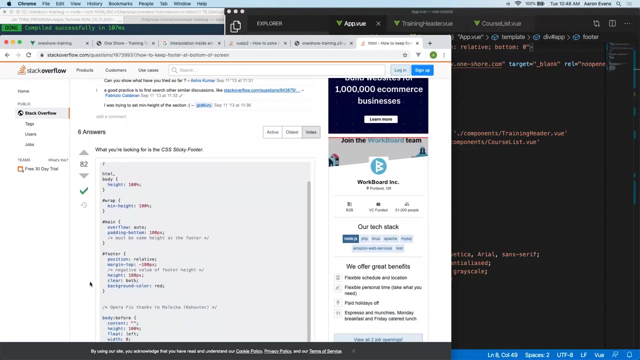 Flitter On at the bottom of the page. Let's keep it on the bottom of the screen. Position: relative margin top. we don't want that. Let's keep it on the bottom of the screen. Let's keep it on the bottom of the screen. 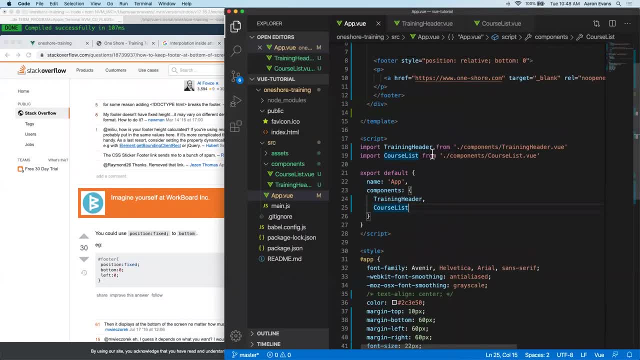 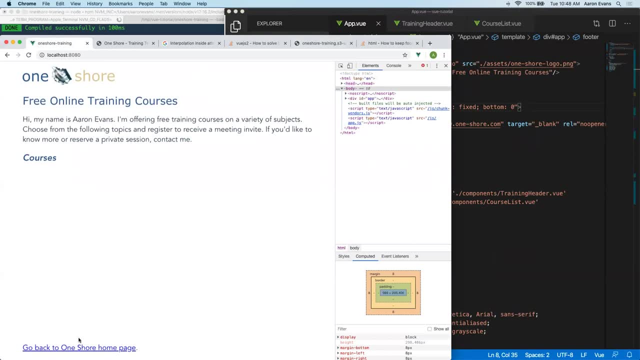 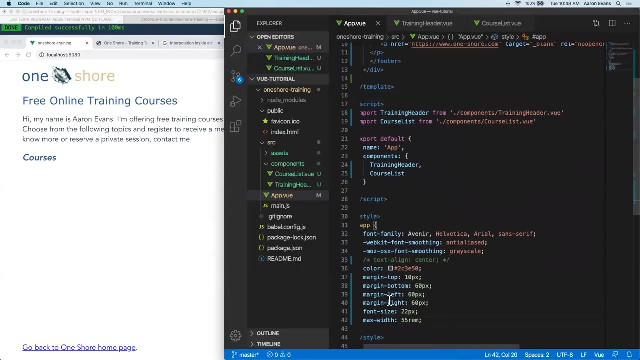 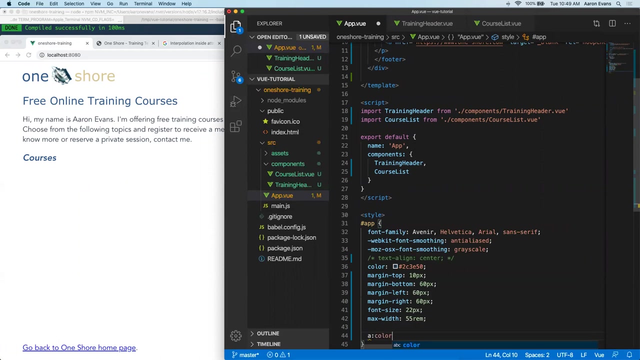 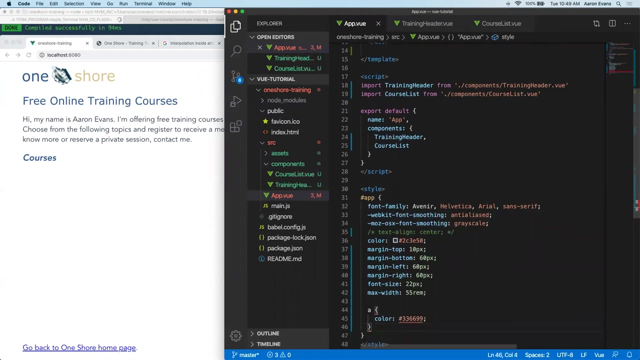 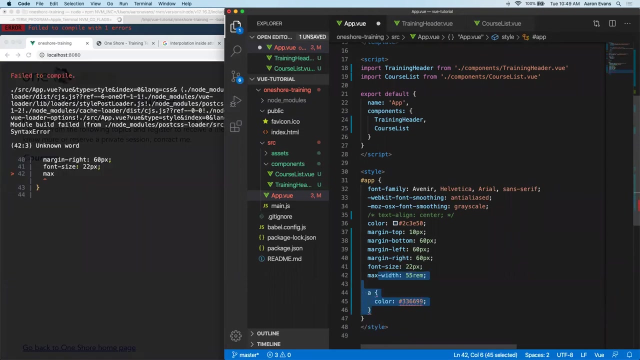 Position fixed: bottom zero: okay, There we go. beautiful, Well, something like that. And then what we wanna do is: we want oops A. oh, There we go. Ah, cut and paste error. Let's make that a little bit darker. 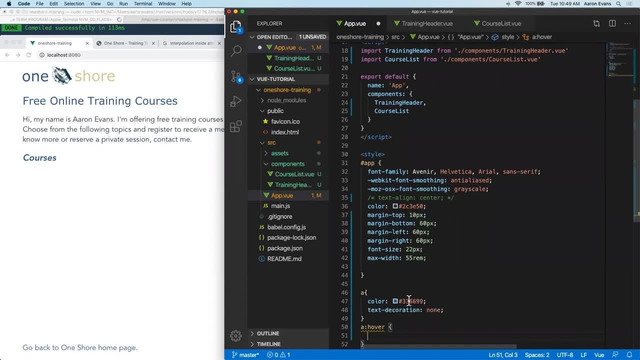 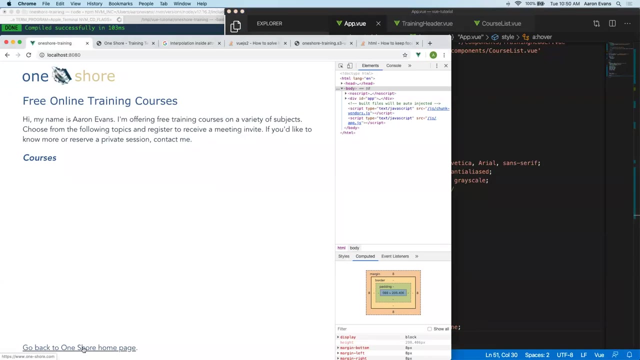 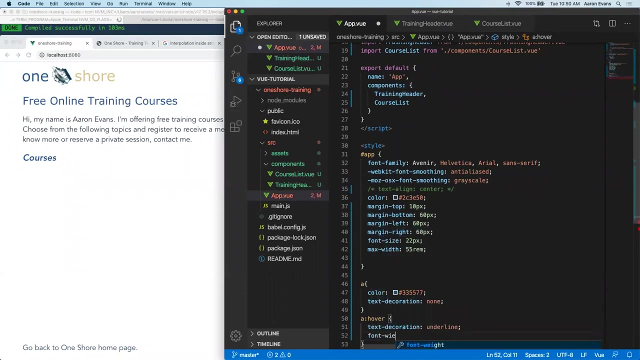 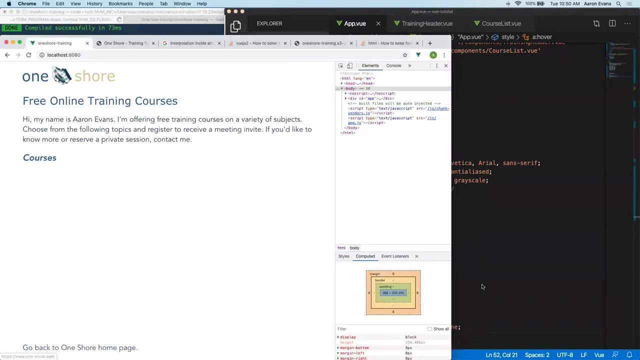 Let's make that a little bit darker. Let's make that a little bit darker And we'll just add a little Q when we hover over it. it underlines great, And we can even do something like this. Now it goes bold. 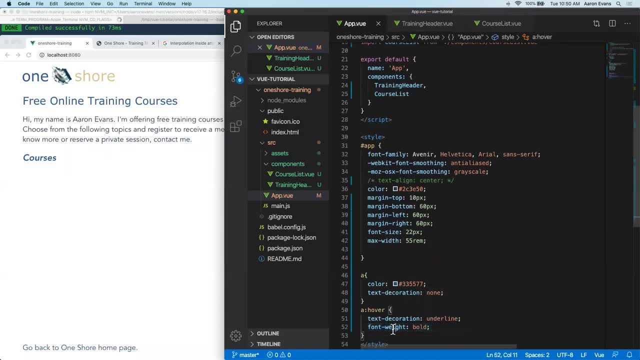 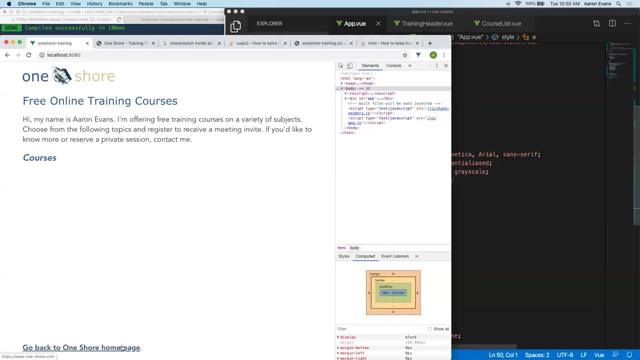 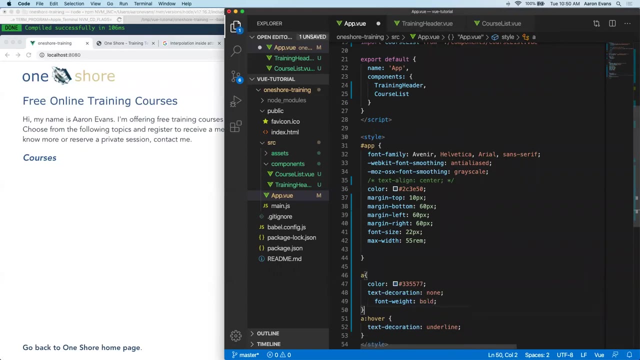 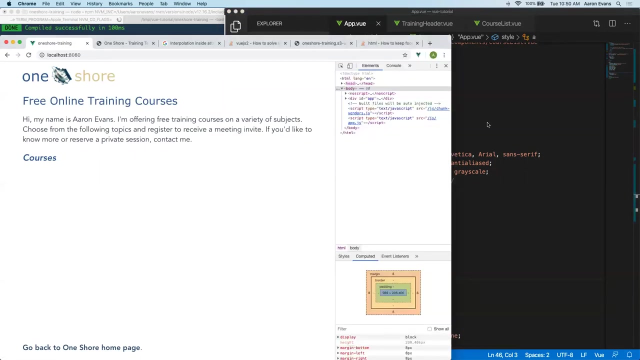 I don't like that Could make all of our links bold, though I think we want it semi-bold, but we're not gonna worry about that now. Okay, we've got our page working. We need to get our course list now. 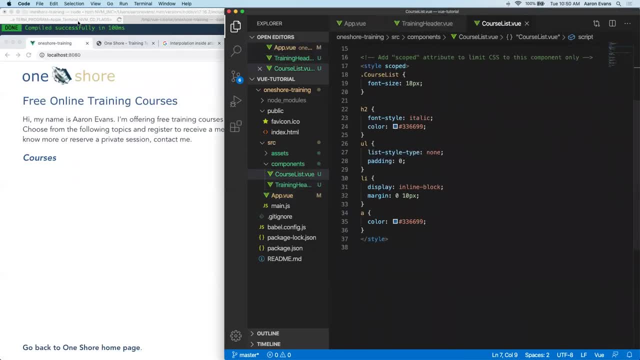 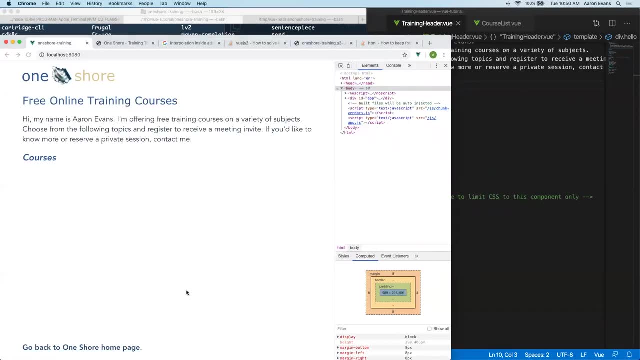 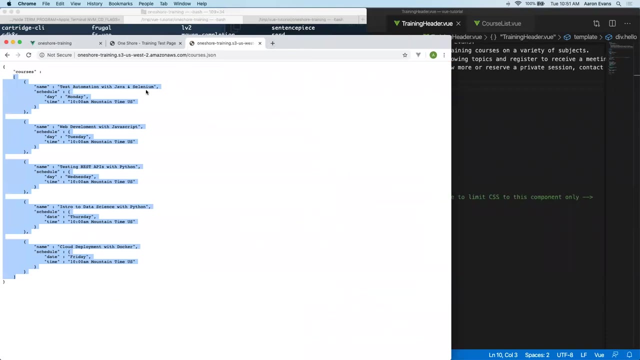 Okay, first thing we're going to do is we're going to do it the old-fashioned way, just to test out. So I'm going to grab my ah, Too many windows gonna be sick. All right, So in our course. list component. 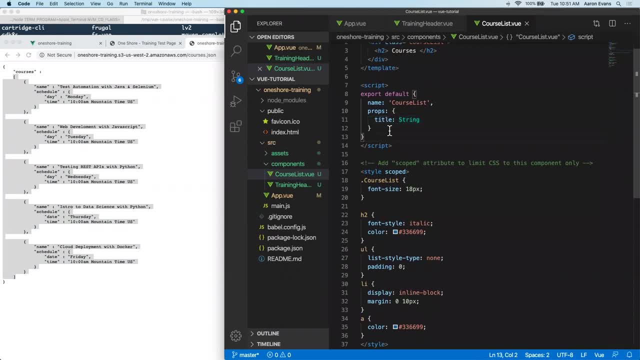 we've got our properties, we've got our title, which is a string, And it's actually a good idea to pass this in separately So you can do data colon function, Or you could do data with brackets And not the colon. I 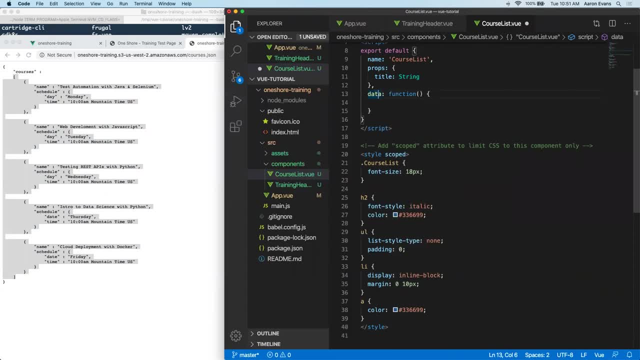 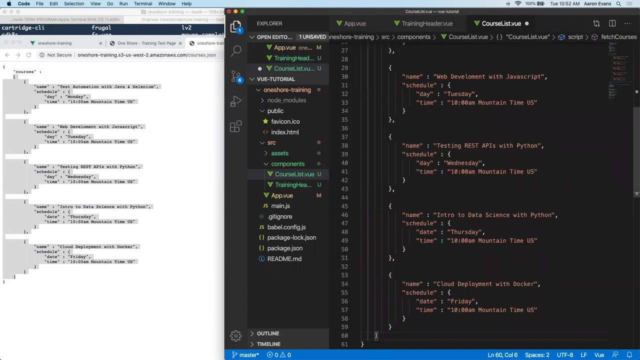 Like to be consistent. if I am creating an object, Then I I want them all to be colon, whatever it is. And what I could also do is I could also do Function fetch courses. that's a good start, And what this will do is this will return. 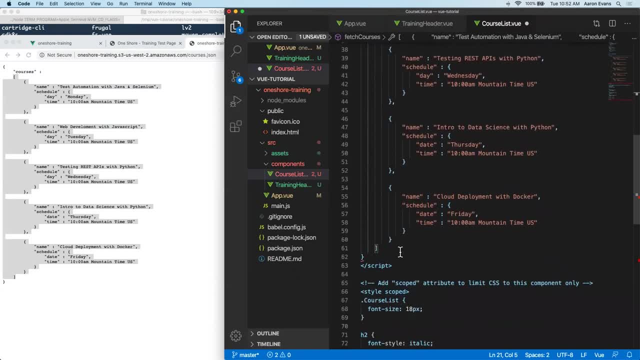 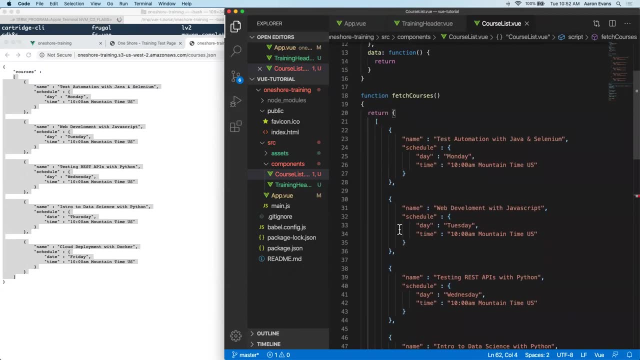 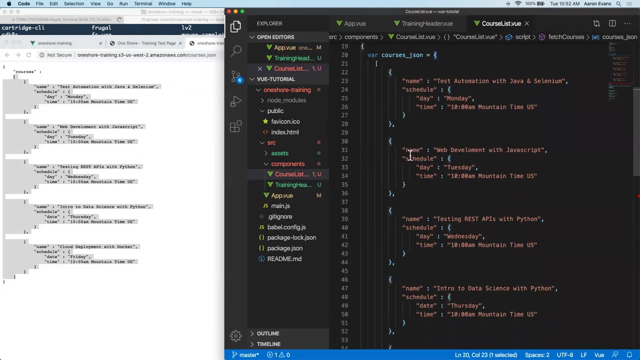 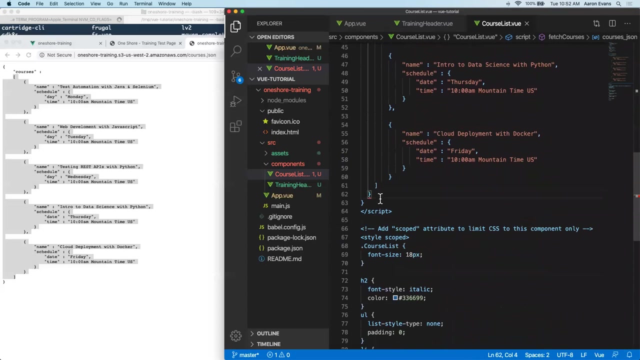 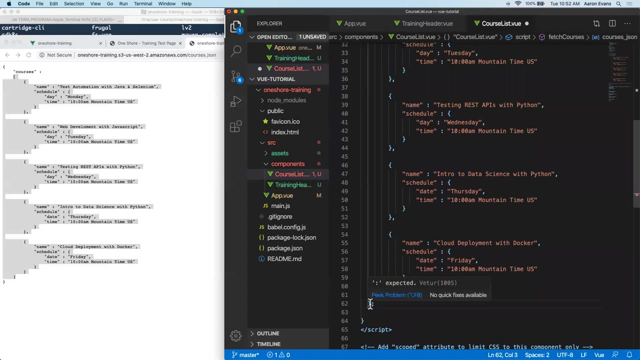 An object that contains my list. Let's see what does this line up with. does it want to semi-colon? what does it want to be happy? Let's see what does this line up with. What does it want to be happy? tell me VS code: expected colon. 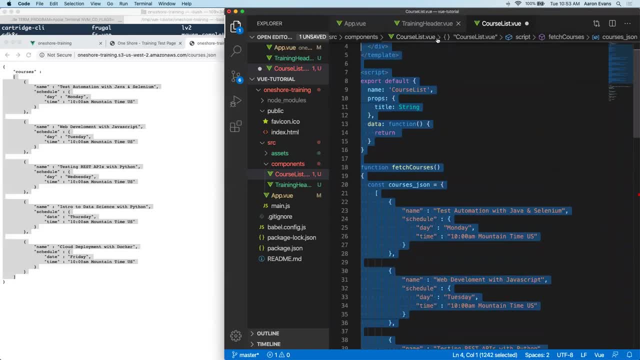 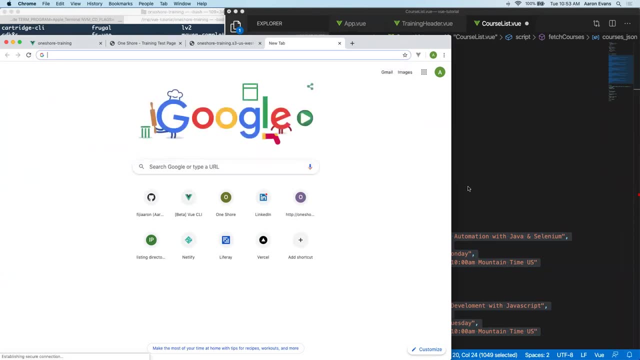 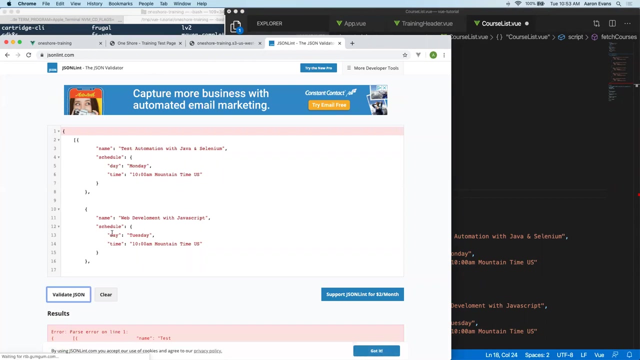 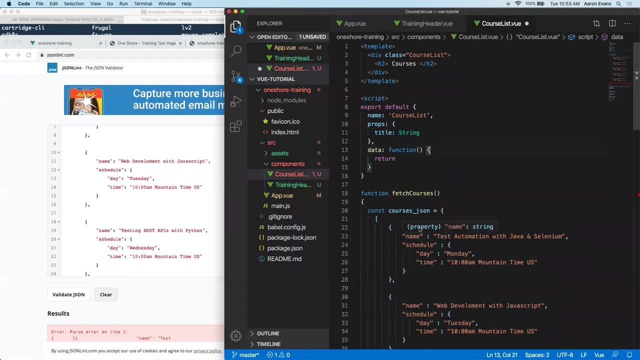 Expected colon. where do I have a parsing error? Is this even JSON? no, oh, it is JSON, okay, so I can Often do something like this when I need to see if I have a typo somewhere. Parser name: test line one: Is it the ampersand? 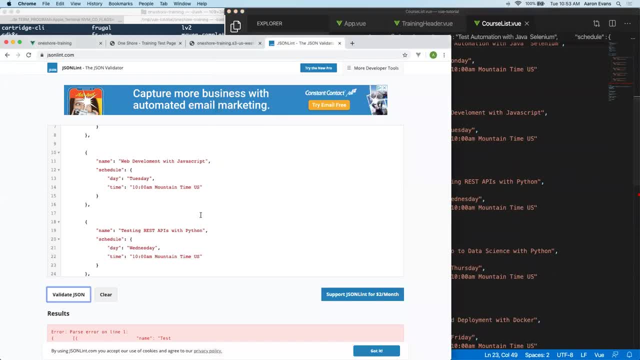 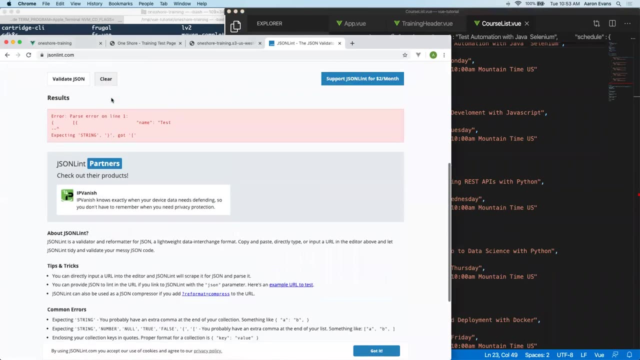 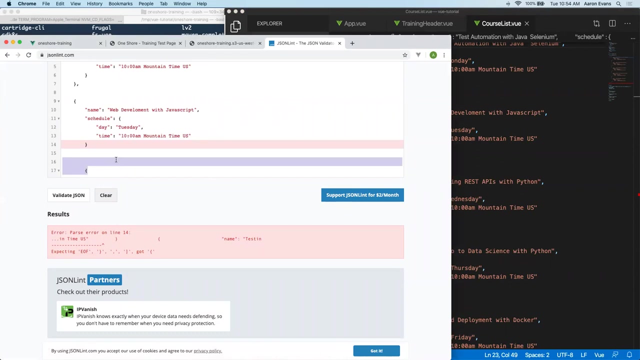 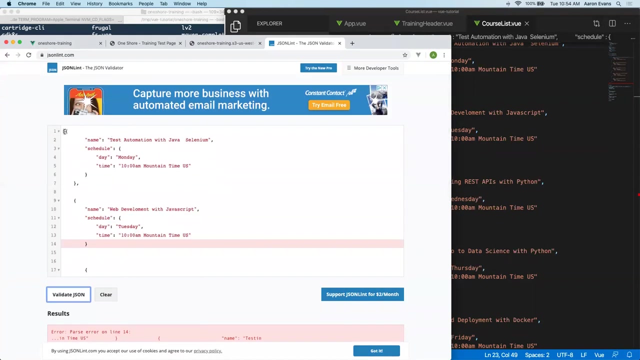 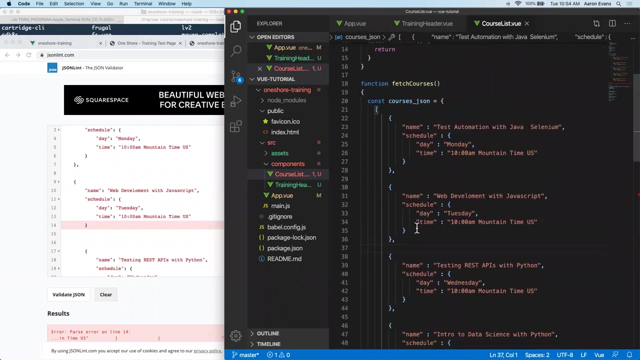 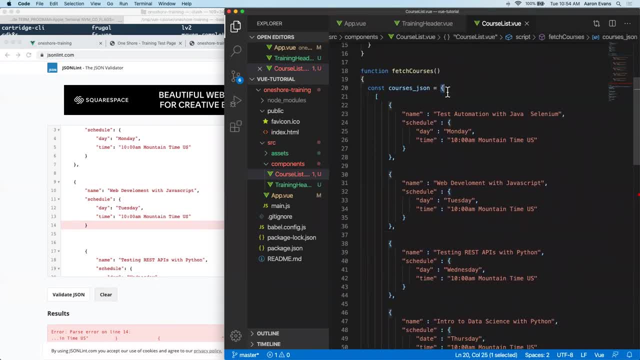 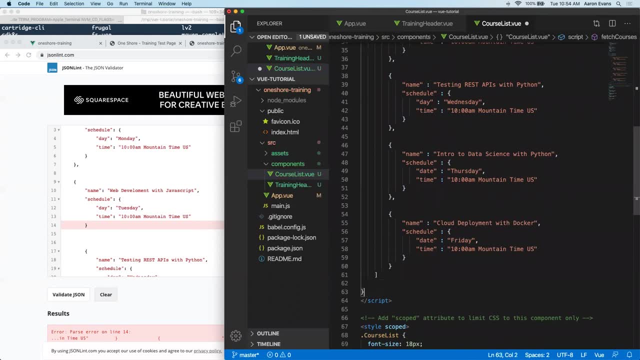 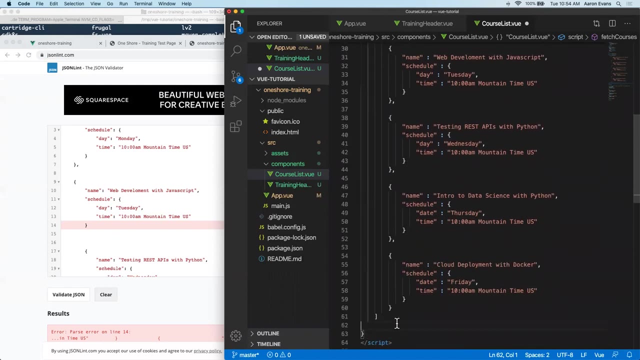 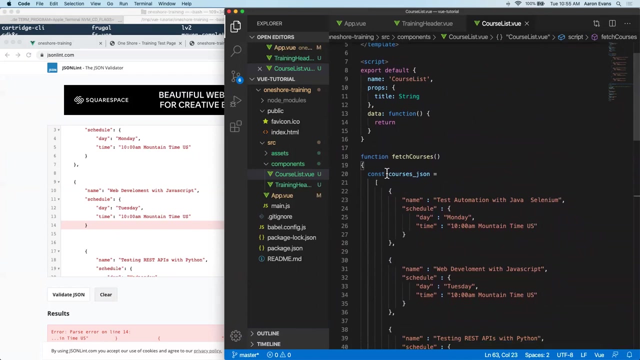 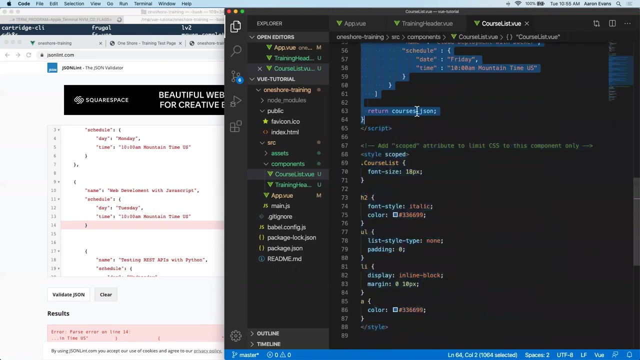 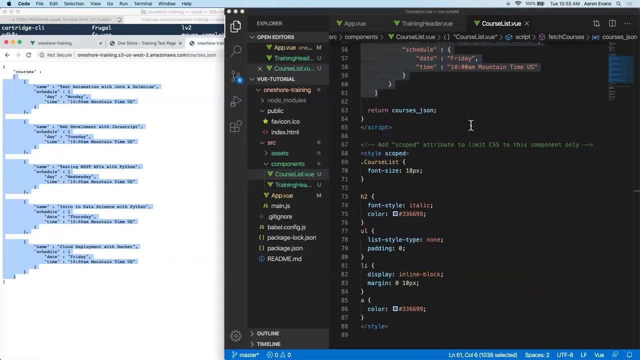 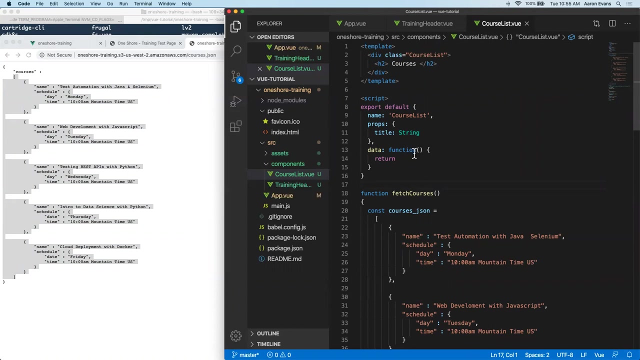 all right. I don't know where it was, something with the extra curly brackets. okay, so we've got our courses JSON. let's just validate this one more time. it likes it? all right, so now our data function. this is something that it's ugly. what we want to do is we want to return an object that contains this array. 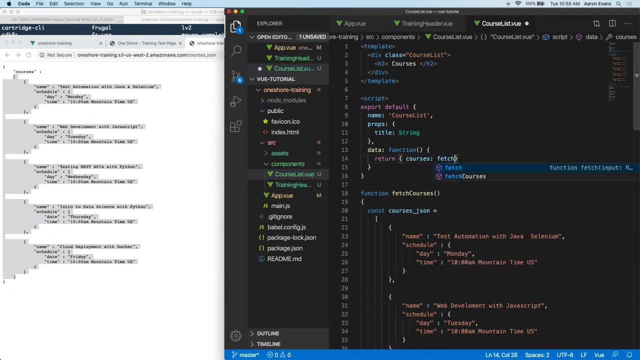 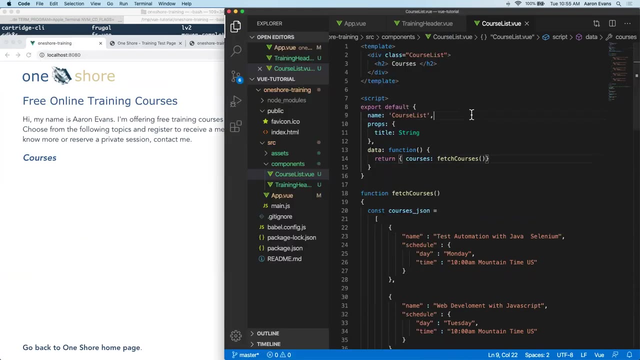 fetch courses. I'm not sure about the order of precedence. if it's going to no, it should export this after it parses that all right. so now I have in my data, I have courses, so I can do this. courses subzero dot name. right, there we go, and I can change that to courses sub. 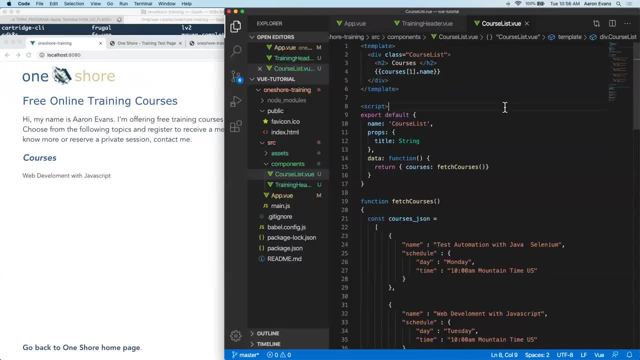 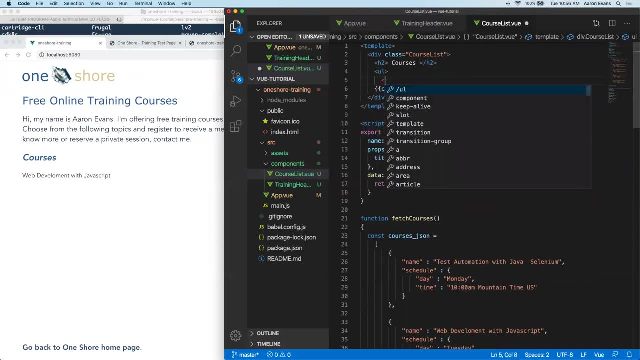 one dot name, web development with JavaScript, and so forth. so what I want to do? I want to go back to what we did last week. I want to create a list and for each list item I want to do v4. I want to do course in courses. let me show you how. 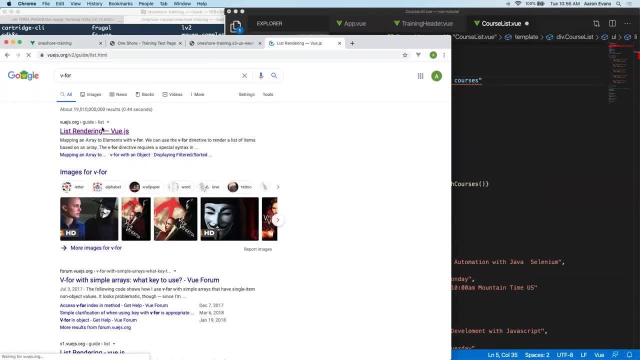 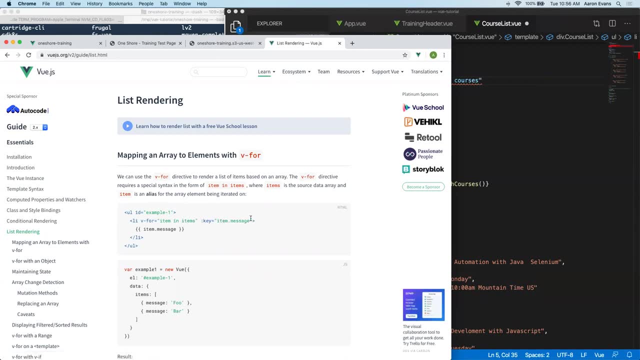 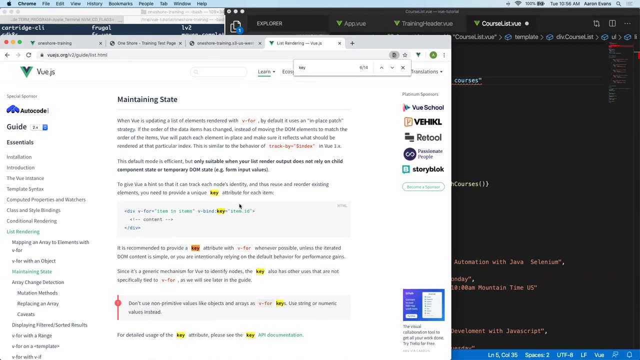 the documentation list, rendering v-4 item in items and you can see you can specify optionally a key there. it is recommended to provide a key attribute whenever possible, unless the Dom is simple or you are intentionally relying on the default behavior for performance change. don't use non primitive values like objects. 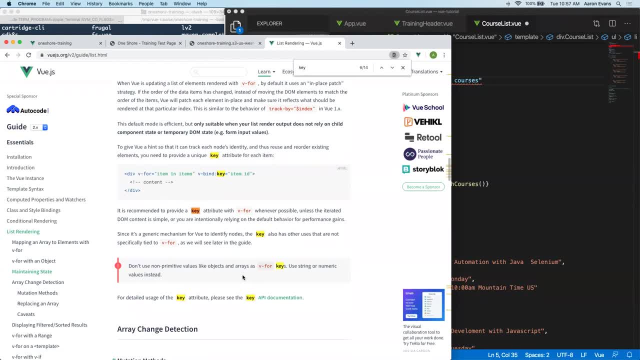 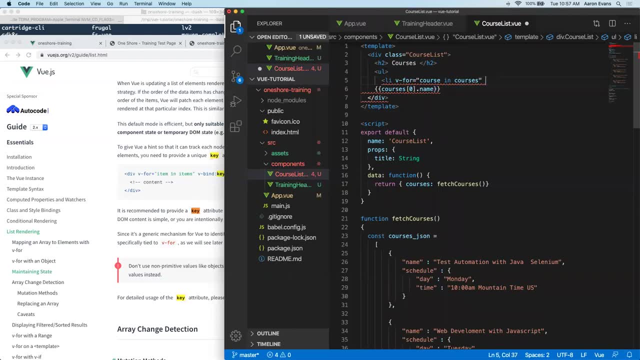 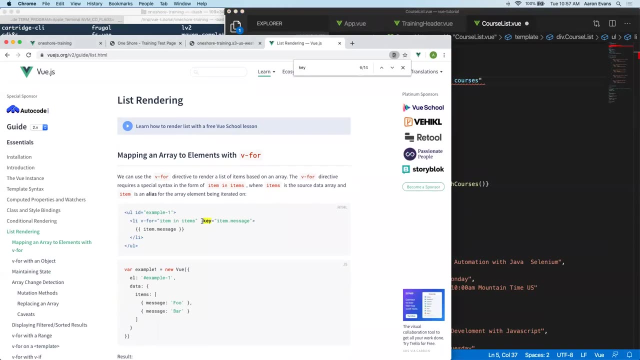 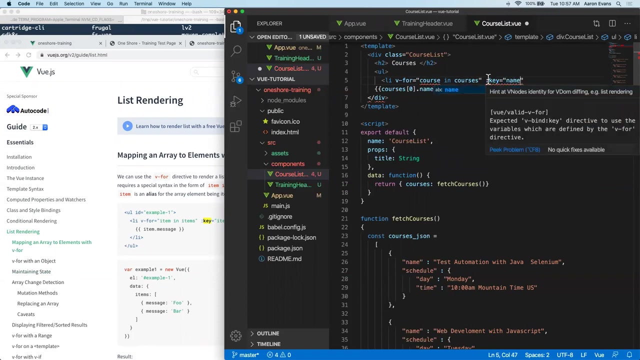 and arrays for keys use string or numeric values. now the key would be the name, so we could say key equals, or we could do colon key or, you see it, V bind key. so colon key equals name or equals course dot name. we didn't do that last week just because didn't need to. 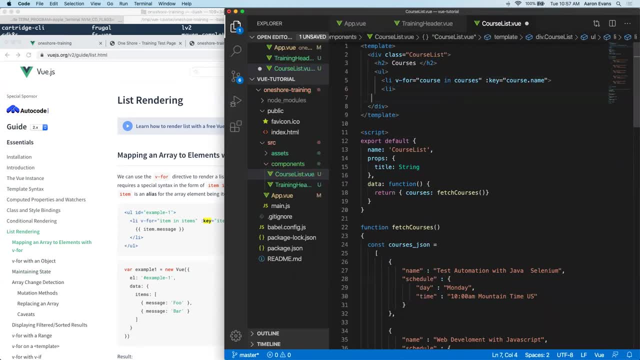 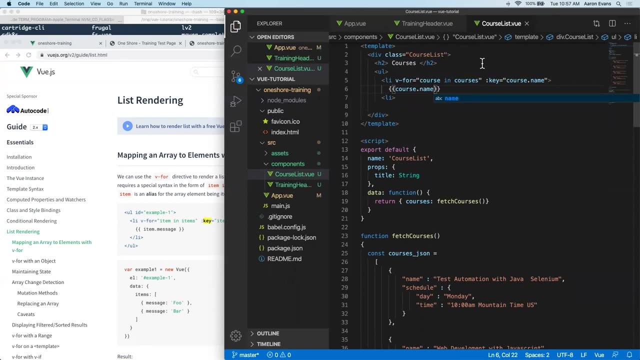 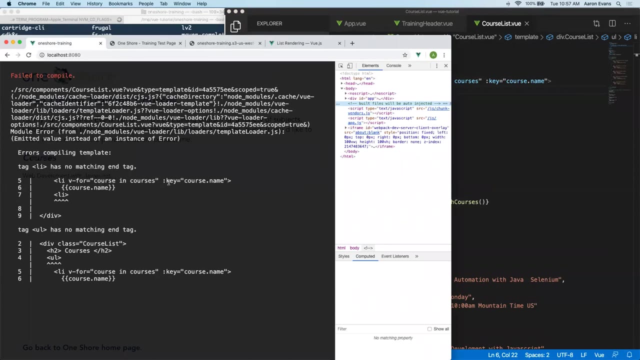 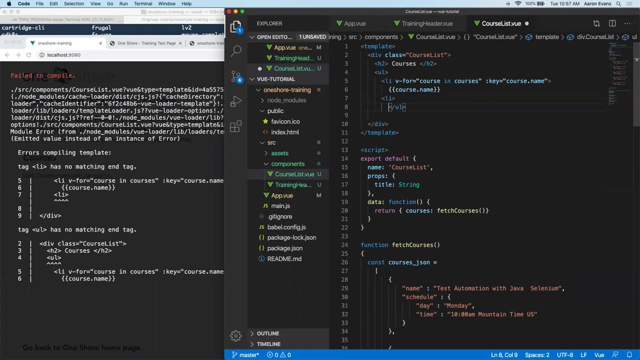 because you didn't know us yet, hit a mixed box, which is kind of interesting for complex series. okay, so now, instead of listing each one individually, I can do, of course, the hot name. hop back over here to our UI. we've got a compiler for course and course is key. course. name ul has no matching in tag, if you remember. 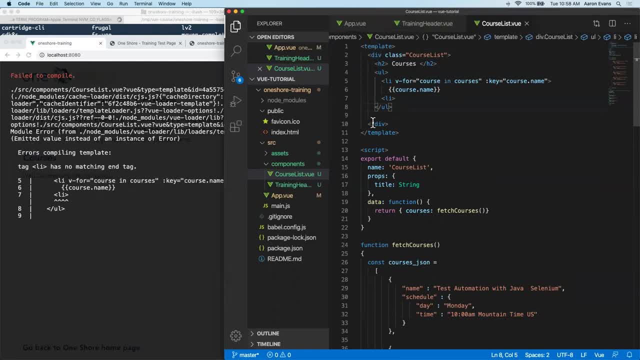 because I had two components and my close div tag didn't have a slash and Vue was just giving me these ridiculous errors. But it looks like Vue serve it gives me better errors. You can see here: my li doesn't have a closing tag. 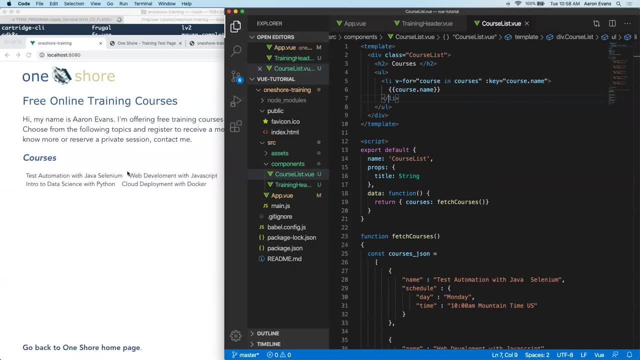 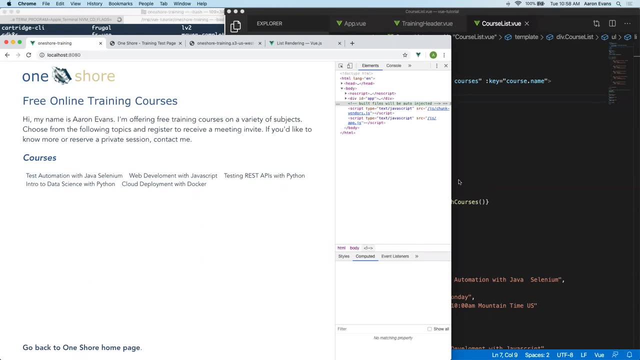 Tag li has no matching in tag And the Vue. Google developer tools can also help you get better. So now I have this, it's kind of ugly And because my list is an inline block, I don't want it to be an inline block. 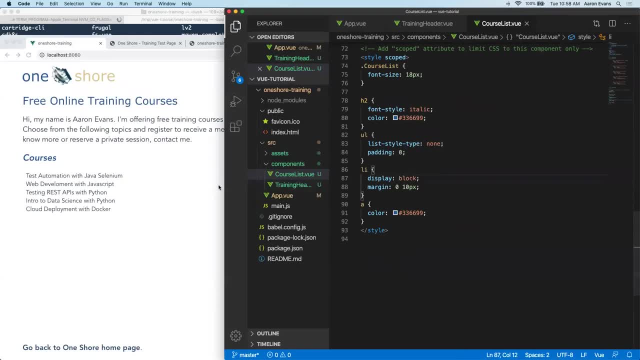 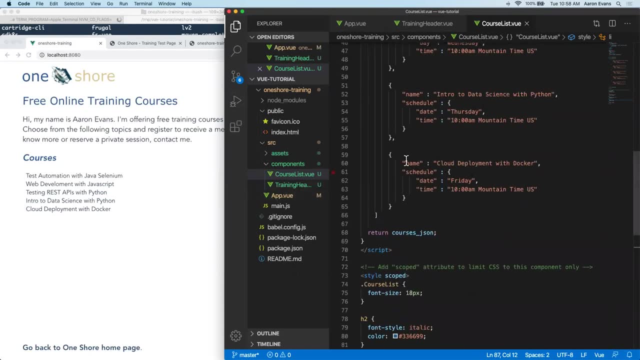 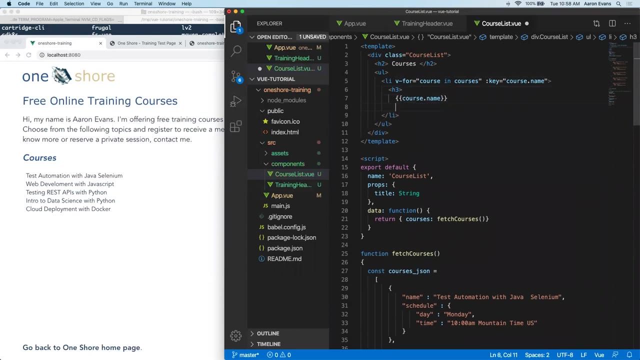 I want it to be a block. So now, I've got my list. What I want to do, though, is I want to have a title, So I'm going to add a little bit of structure to my list. I'm going to add a H3 element for the course name. 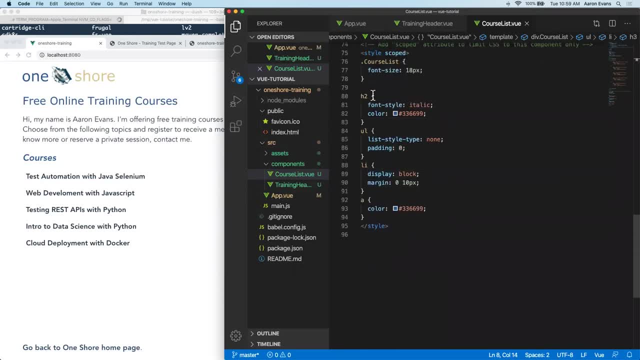 And we just make it a little bit bigger And I'm going to add a little bit of structure to my list And I'm going to add a little bit of structure to my list And we will eliminate this font style. We'll make that consistent across the different fields, the headings. 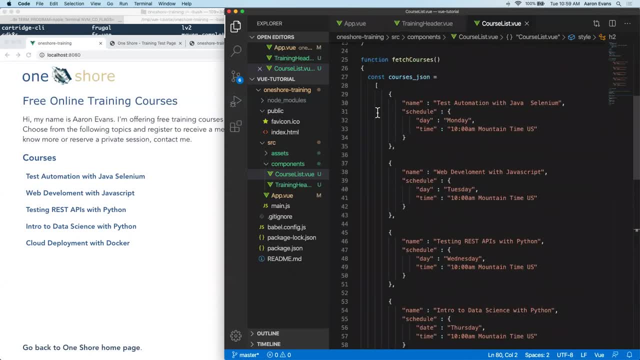 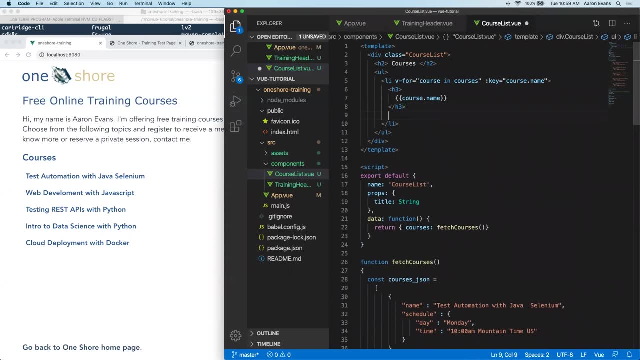 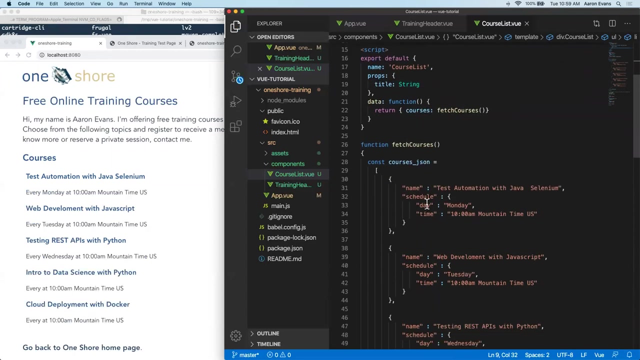 And then what we want to do is we want to get our dates right. So every Course schedule dot day at course schedule dot time- I need to look at my JSON here. Schedule day, schedule time. There we go Every Monday at 10 am. 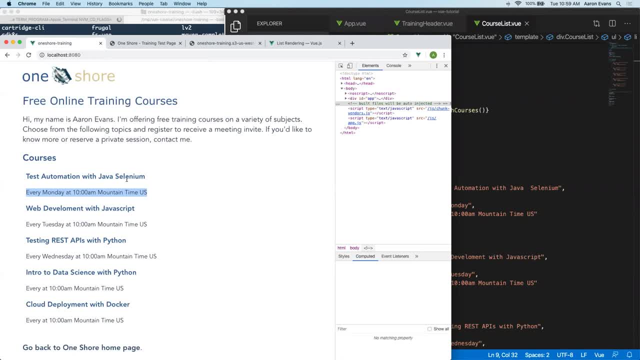 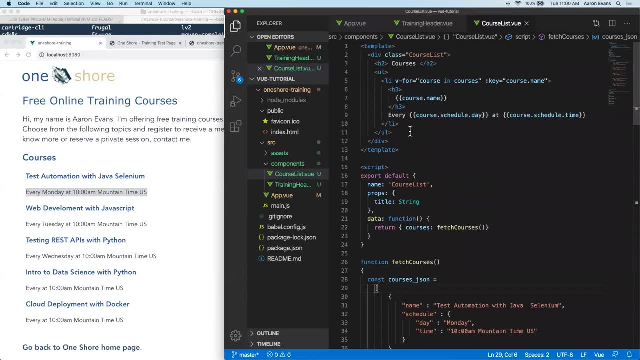 Okay, So we've essentially got to roughly where we were before last week Only instead of. So, instead of implementing it as a standalone component, we're building it with the Vue CLI. We've got standalone components. We didn't implement it as standalone components. 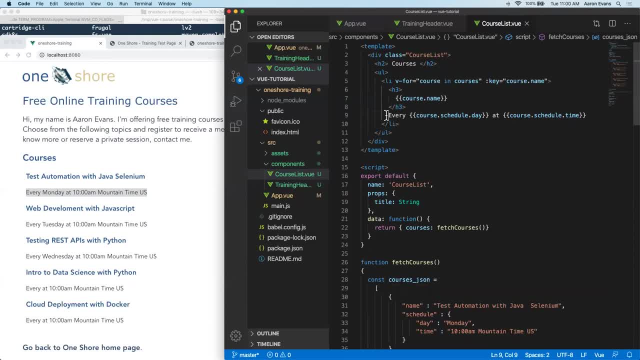 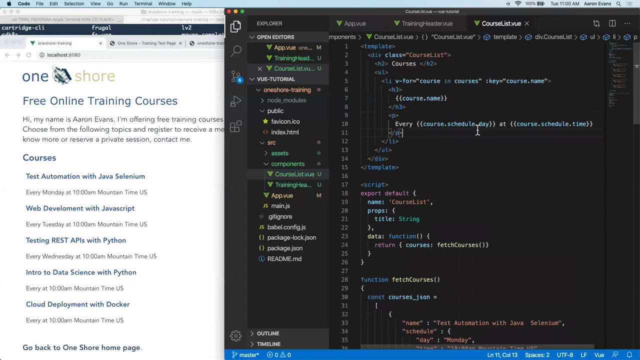 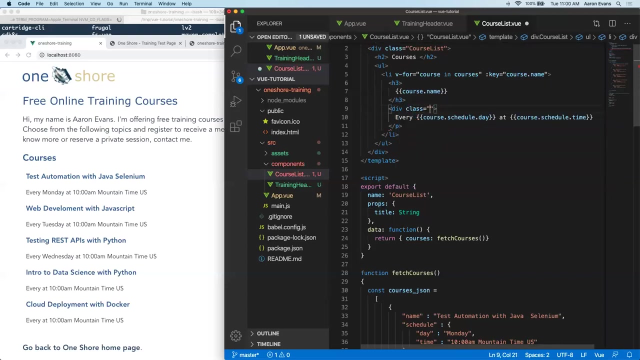 We did it in line with our HTML last week, So, And we can create that as a P tag paragraph. And then what I'm going to do? Well, we don't want that as a paragraph. We want that as All this div class equals schedule. 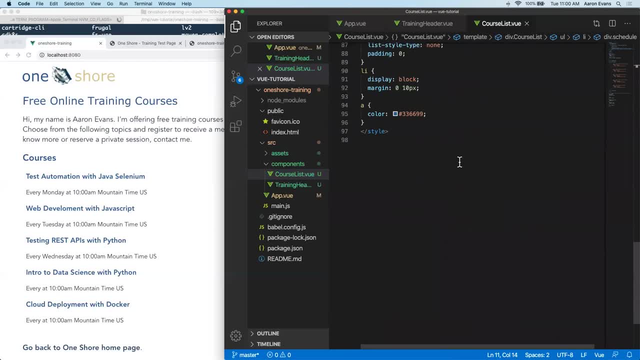 And then just the last thing we'll do is we'll do something like in our scoped div. The nice thing is now I don't have to worry about all the different CSS tags and stuff. Yeah, Um, Schedule, And then I can do font style italic here. 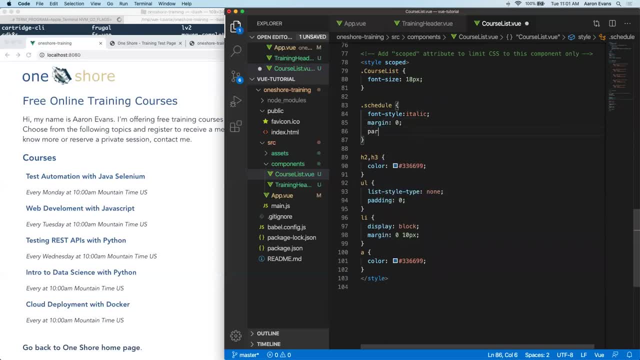 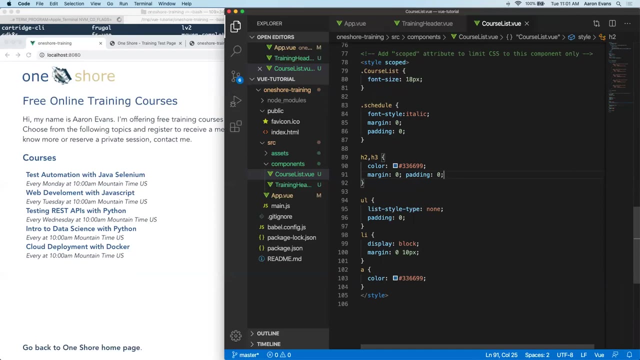 And um, Always clear to find out what's going on. Um, oh, my heading, I think, is Issue there. Okay, So we want to dial that back and say we want the margin here to be something like 10px and 0..